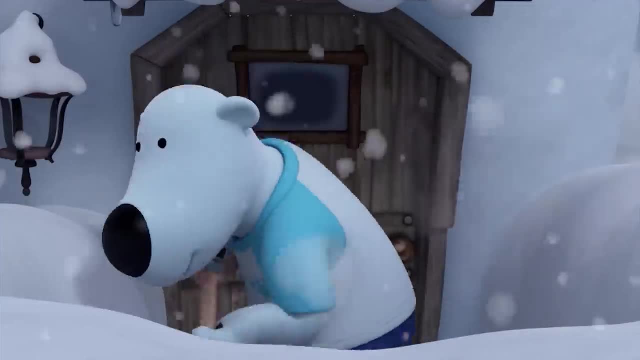 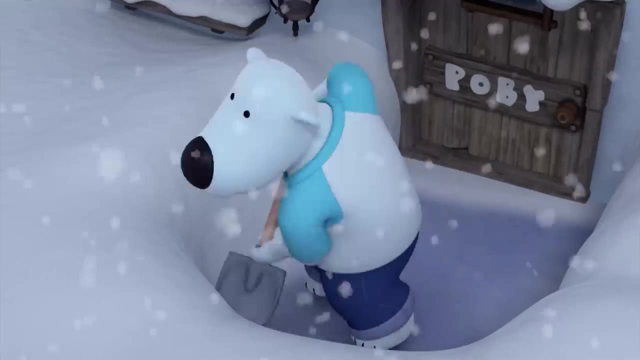 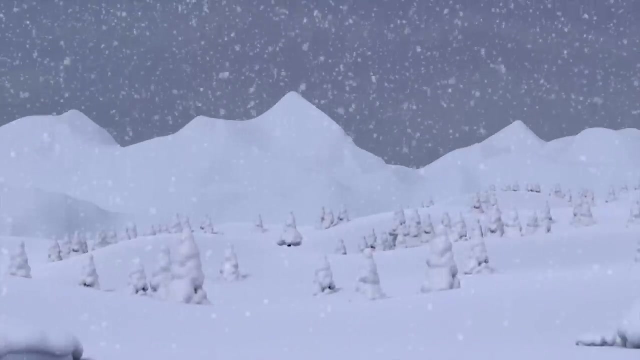 Snow. Snowflakes are like fairies from heaven, dancing snowflakes. It's snowing a lot. Look at that. Because of that, the roads and mountains are all covered in snow. Then does that mean we can't see our friends? 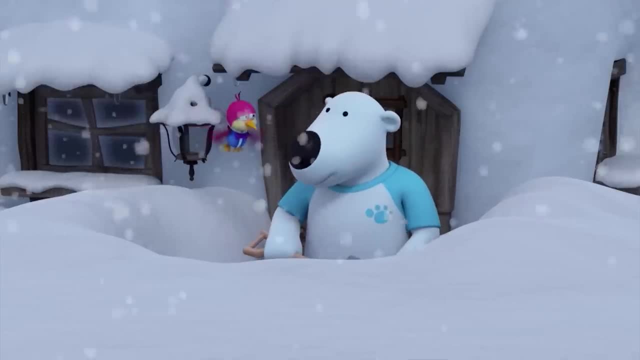 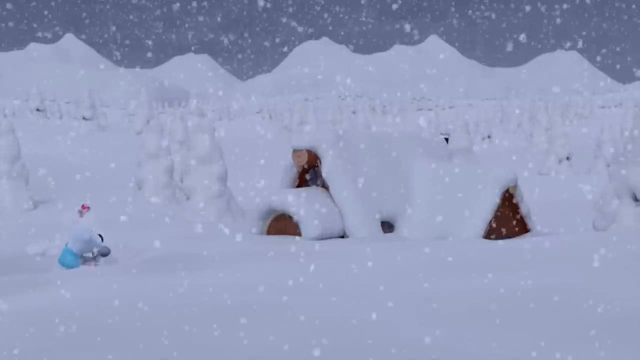 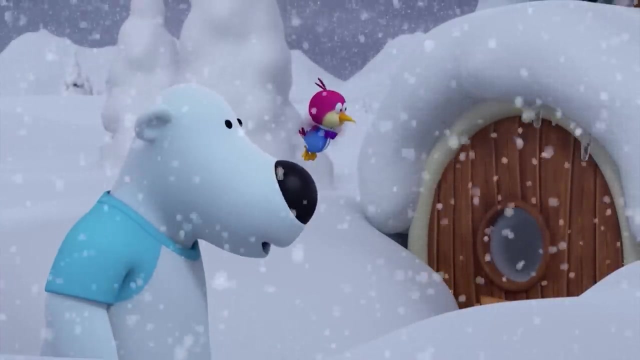 Ah, Let's go and help clean up the snow. Okay, Poby and Harry went to Pororo's house. Pororo Krong, We're outside. Ugh, The door won't open. Look, It's Poby. 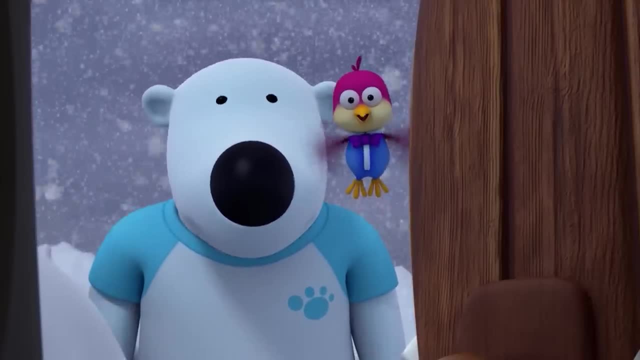 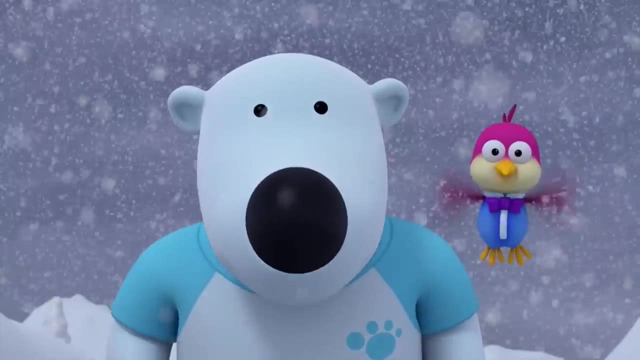 Hello, Pororo, I'm here too. Hello, Harry, Krong, Krong, We're here too, Hello. So you are all here. Hold on. I don't see Eddy and Rhodey since it started to snow. 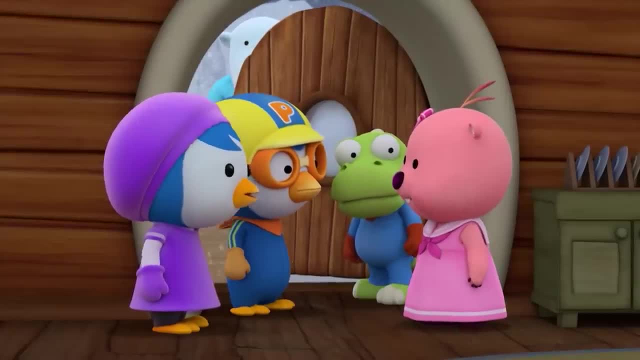 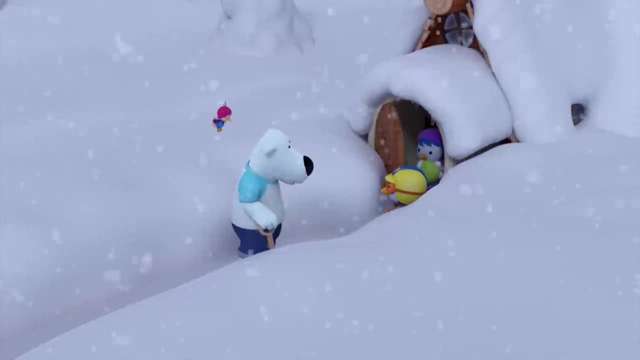 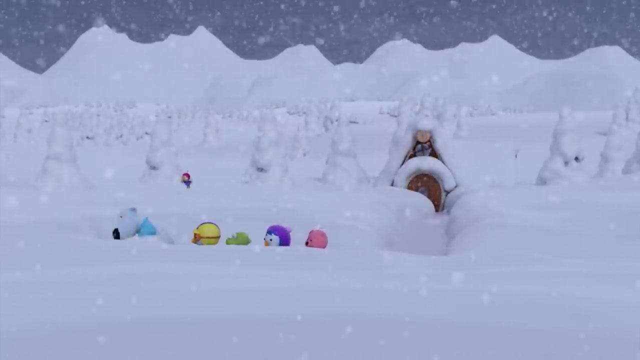 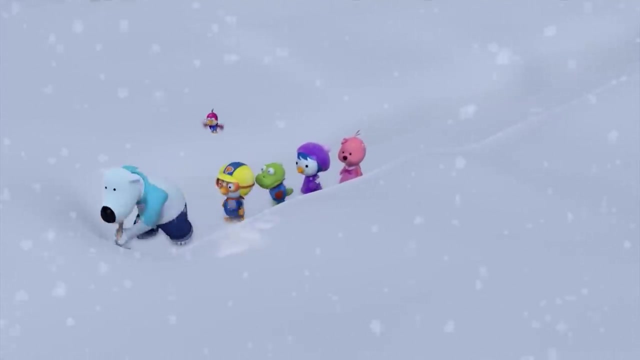 You're right. Let's go to his house. Krong, Krong, It's open. Be careful when you come out. Okay, Pororo and his friends are going to Eddy's house. Huh, There's no snow here. How strange. 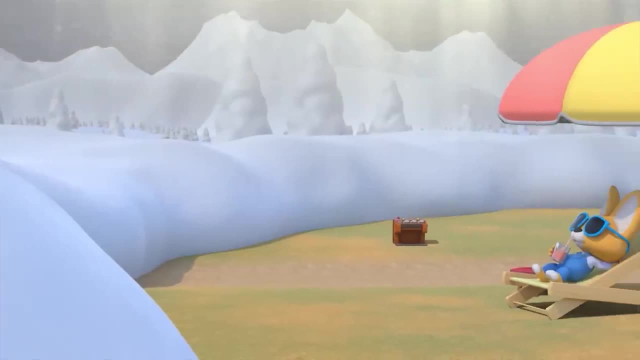 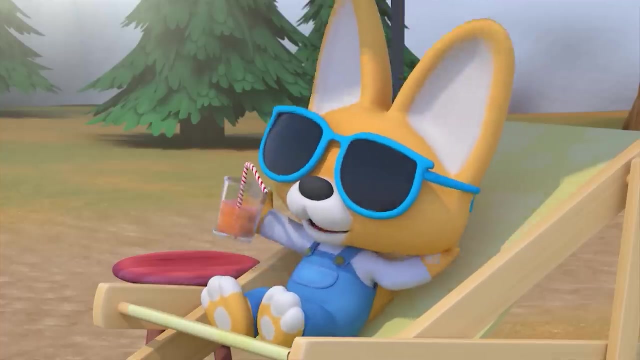 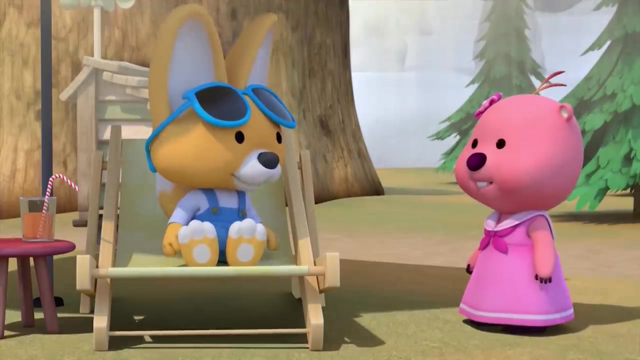 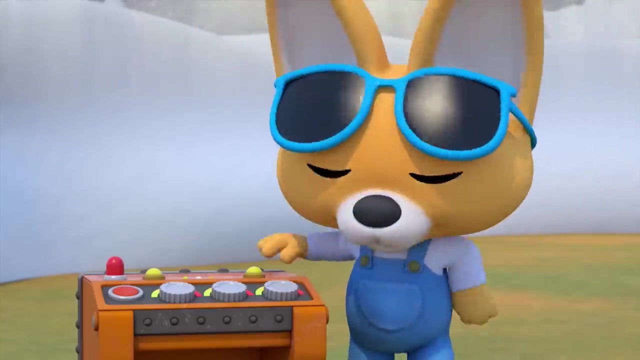 Huh, What happened here? Hey, Eddy, Huh, Oh, you guys are here. Hello, Snow is falling hard everywhere except here. Oh yeah, You noticed that. huh, I wonder what happened. It's because of my new invention. 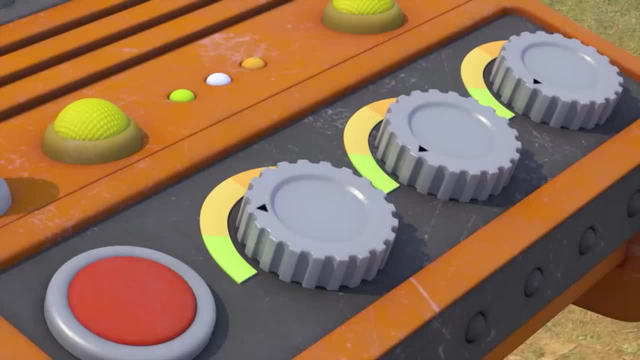 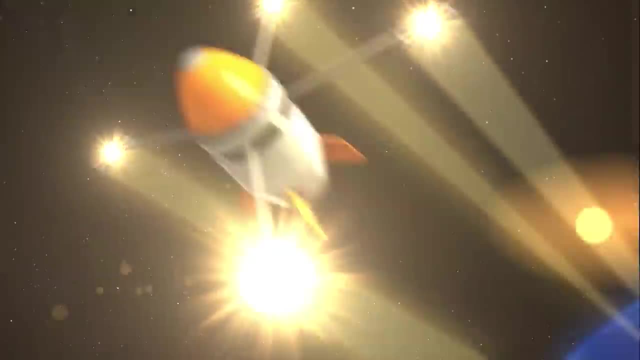 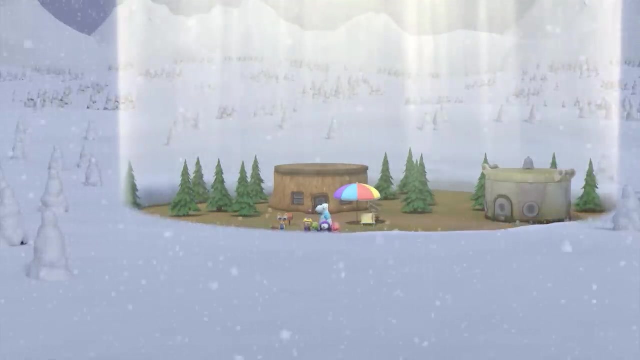 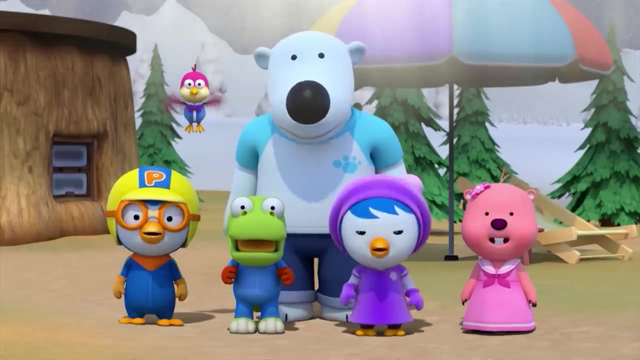 What's that thing? Come on, I'll show you. If I do this, Whoa, The snow is disappearing. But how did that happen? This device is able to change the weather Really. Then remove the snow from our house too. 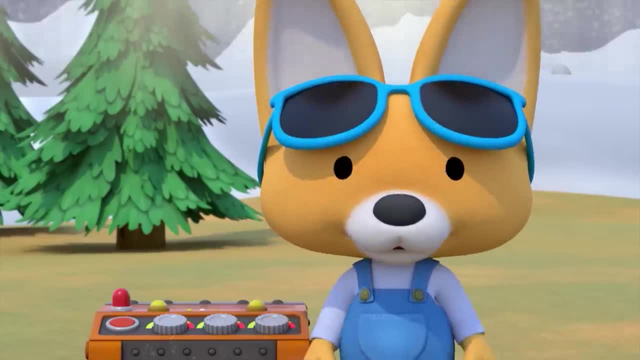 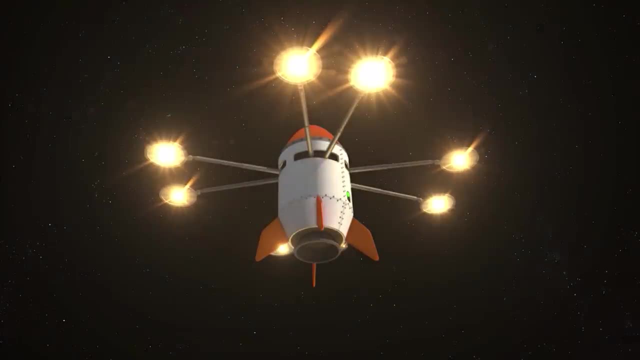 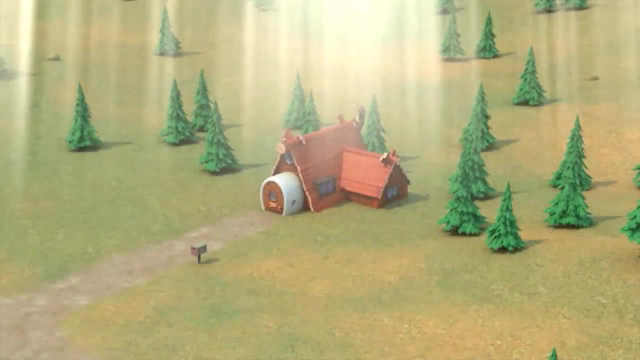 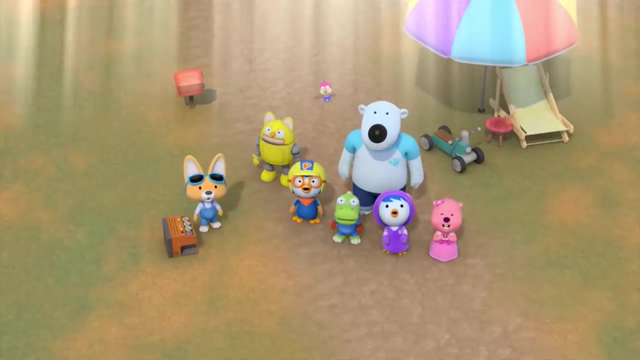 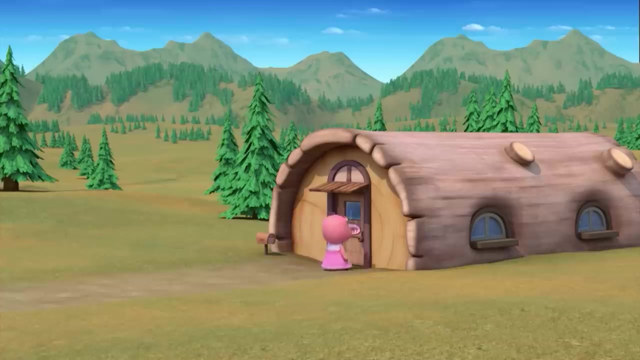 My house too, Really Okay. then, Amazingly, the snow around their houses melted away and the snow piled up in the mountains disappeared. Wow, That sounds so cool. Oh, this is nothing. This is amazing. All the snow melted. 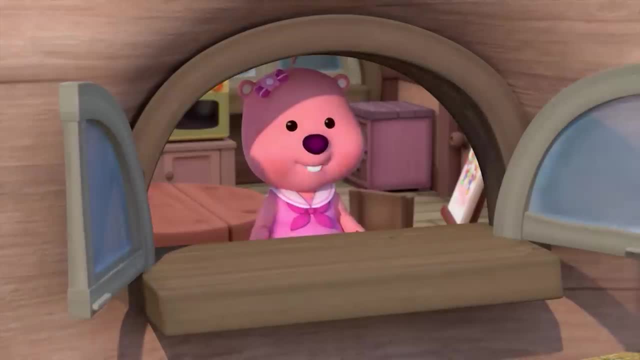 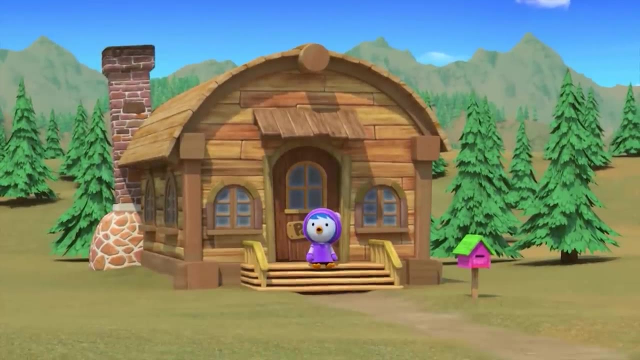 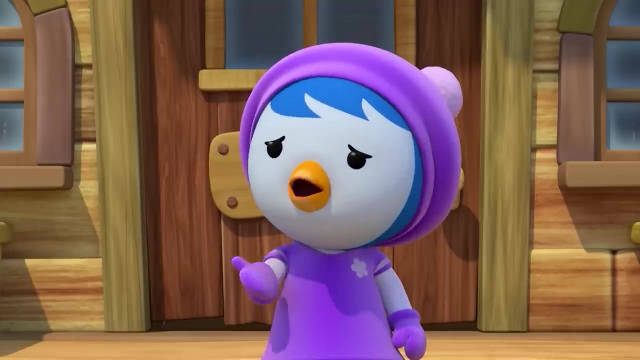 The weather is nice and warm. The weather is nice and warm. Oh, this feels nice, But I I think it's getting a little hot. The snow that piled up disappeared and the warm sun continued to shine, and the weather started to get hotter. 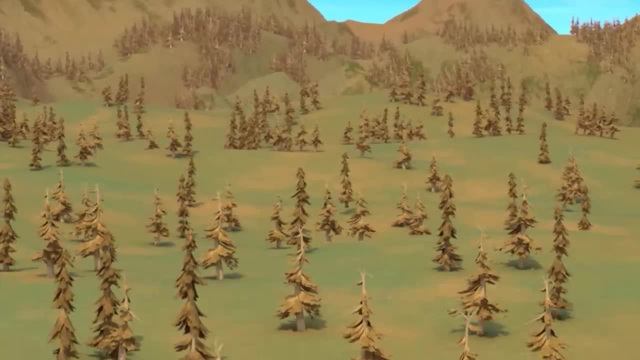 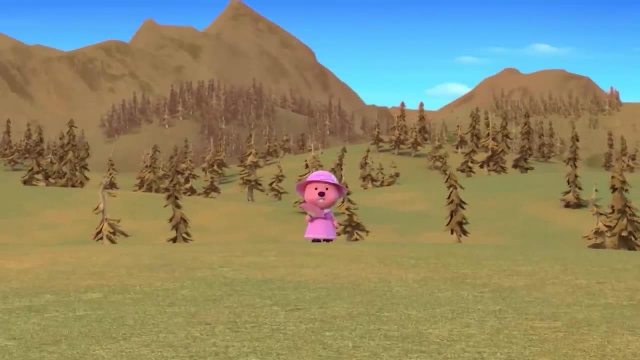 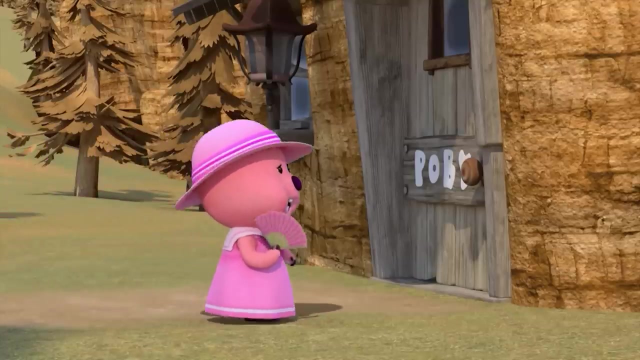 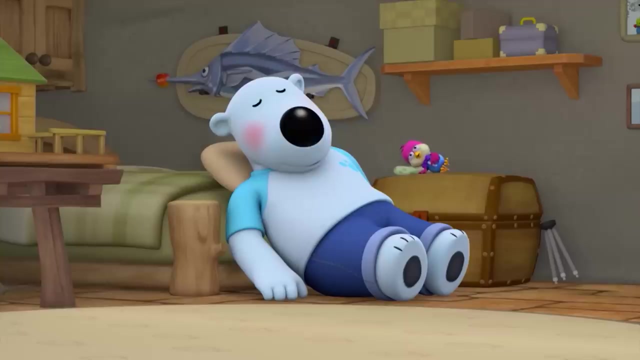 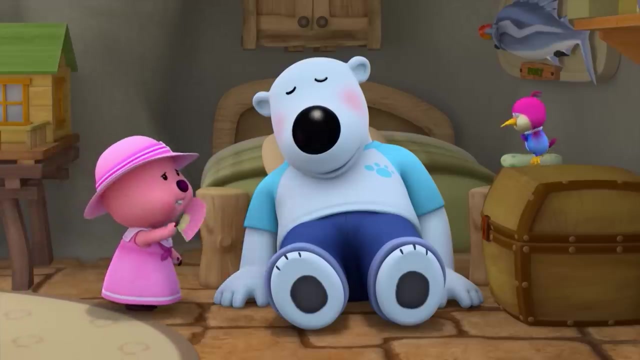 It's getting a little hot. It's getting a little hot. Continued to shine and the weather started to get hotter. Hi, Lupe huh. Moby is exhausted right now because of the extreme heat. It's it's so hot. I think I should talk to Eddie about what's happening. 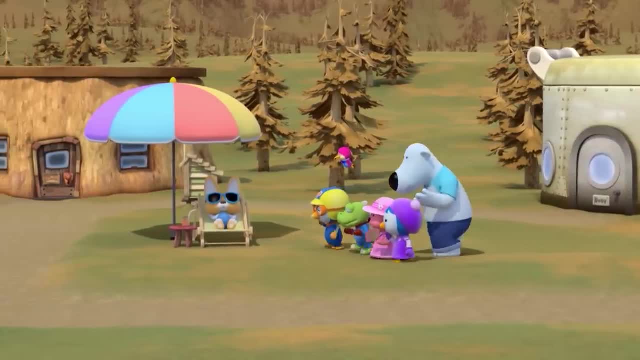 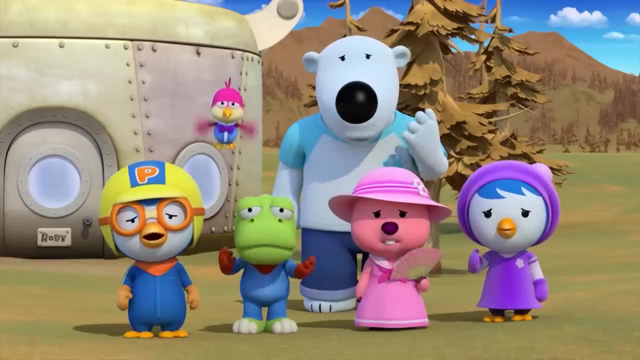 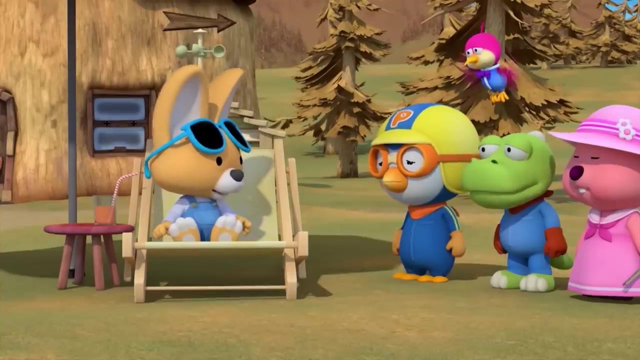 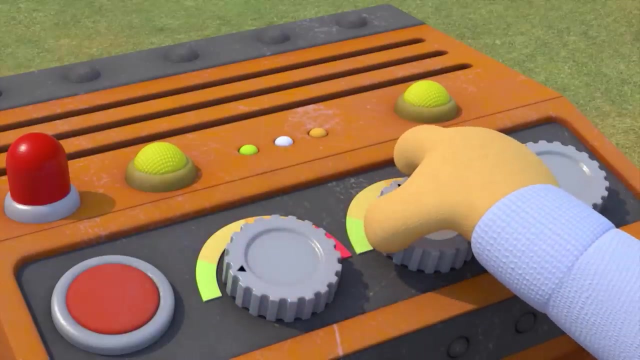 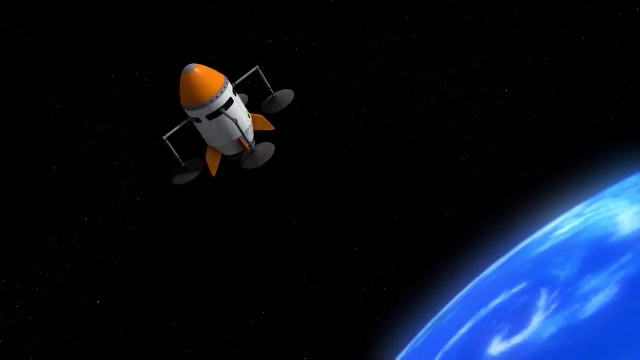 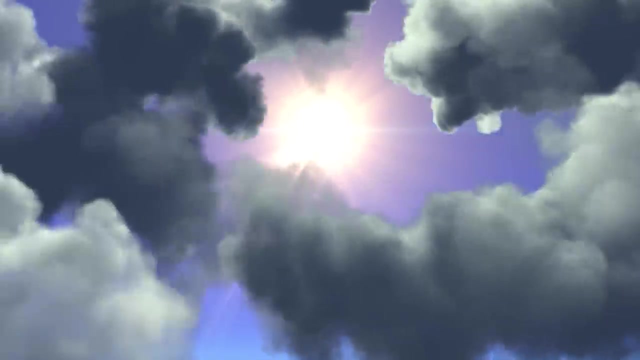 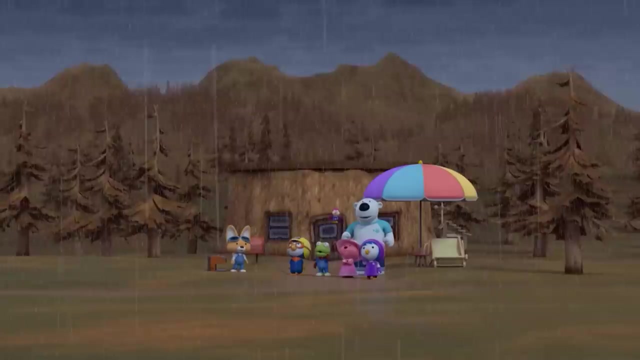 So at that instant, everyone went to Eddie's house. Hello, welcome back everyone. the weather is too hot, Eddie, Really So shall I make it rain then, please? Okay, let's see. Huh, whoa, it's really raining. Eddie, your invention is amazing. 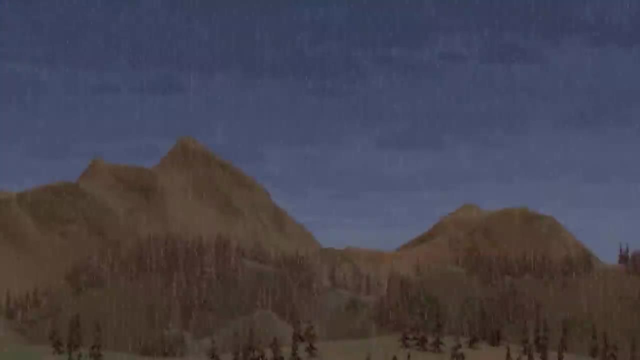 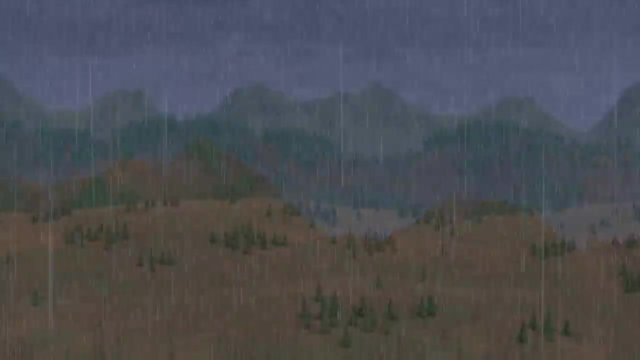 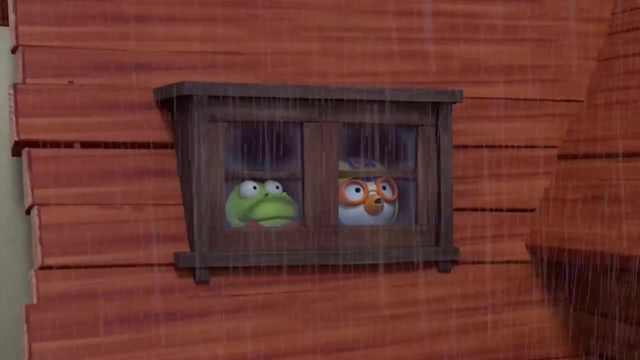 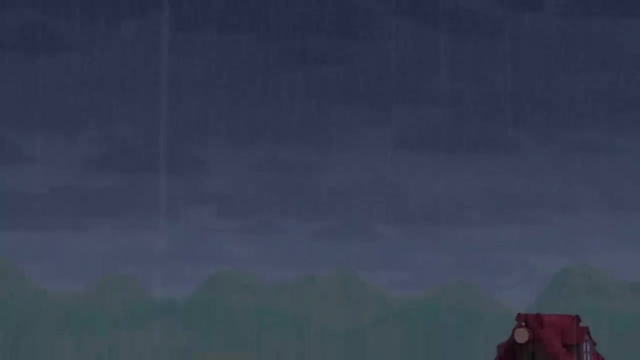 No thanks, This is nothing. But since then it kept raining and raining. not once did it stop. It's been raining and raining the whole day. it won't stop. It rained for several days more, and soon bottom, bottom village started to be submerged in water. 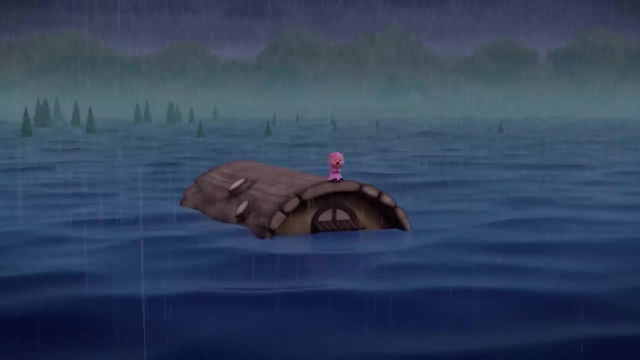 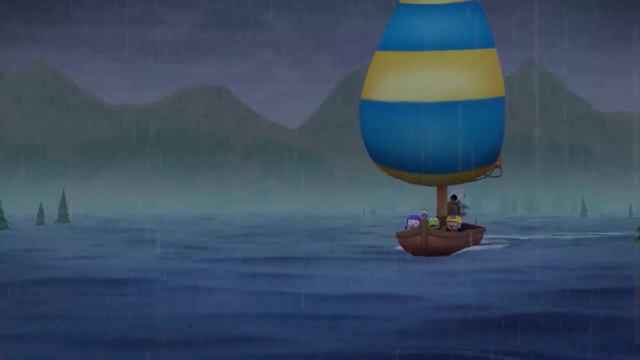 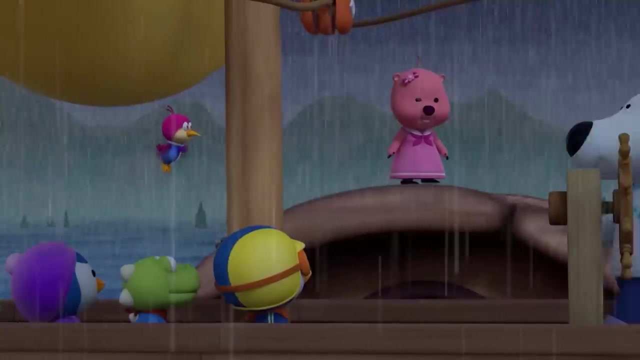 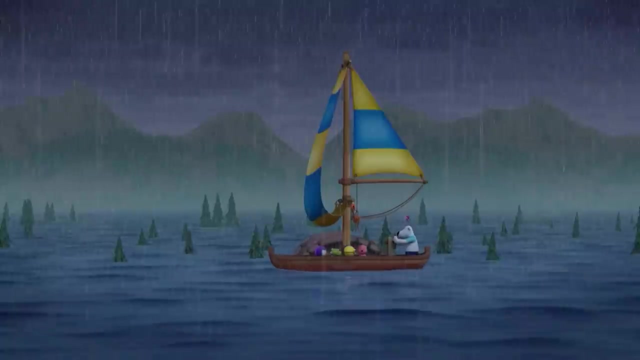 What can I do for you, Booby? I'm there. Boobie got Loopy and put her on the boat and then they went back to Eddie's house. I See Eddie and Vwordai. I see Eddy and Rhody sitting over there. 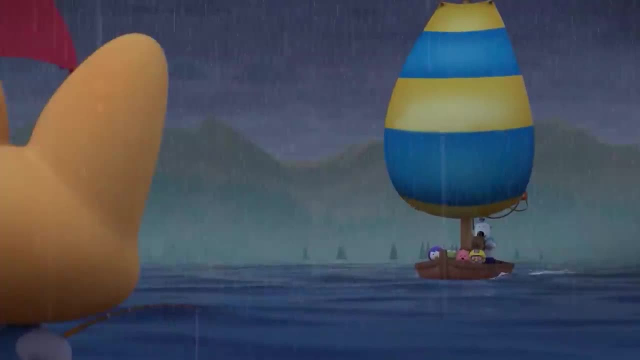 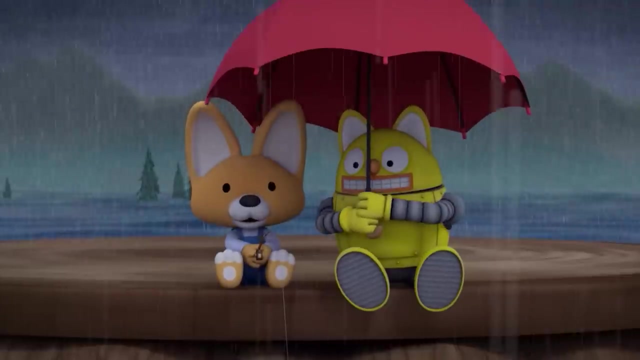 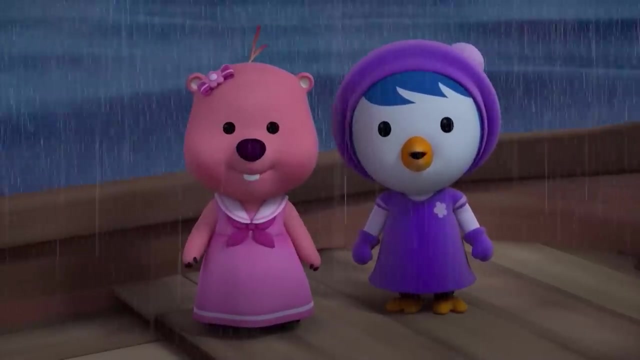 Eddy, Huh, What are you doing there? It started to rain a lot, so I came up here, Me too. Don't stay there, Come down here with us, Rhody too. Uh, shall we? Yes, Uh. 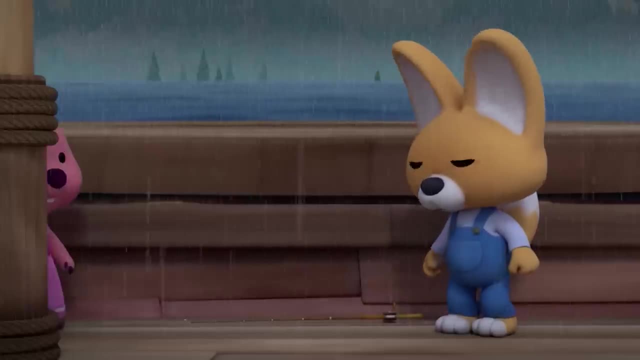 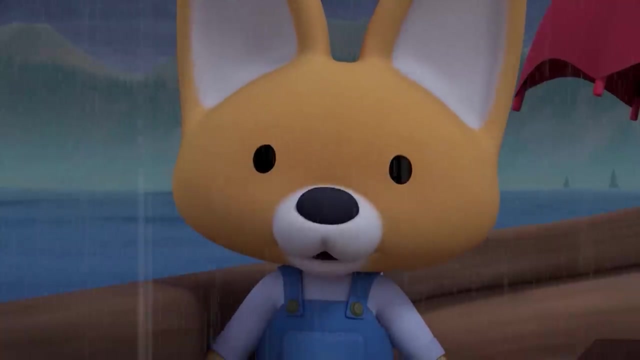 Uh, Uh. It rained so much that everything is under water. Yeah, Can't you make the rain stop? To do that, I need to adjust something on the machine. I can't go into the water because I don't know how to swim. 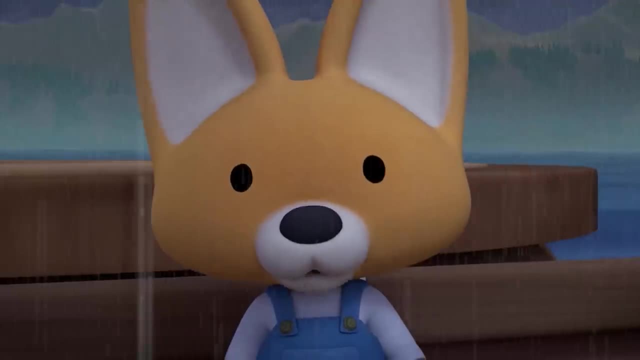 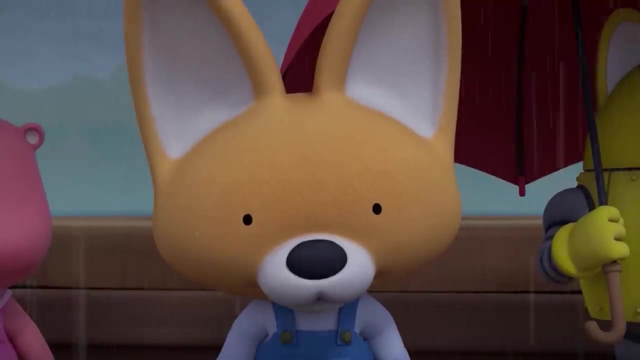 I'll do it. Tell me what I should do. You just have to turn the dial. Okie dokie, Oh, hold on, There's more than one dial Here it is. Oh, Which one should I turn, though? 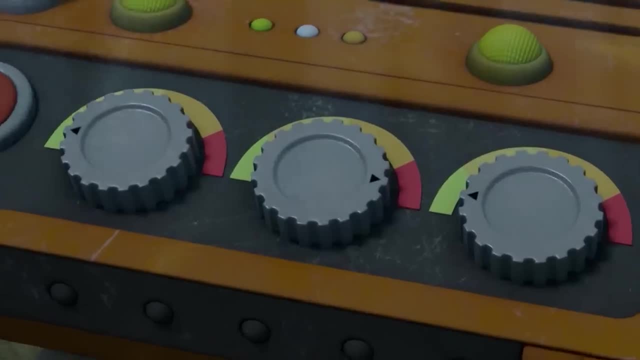 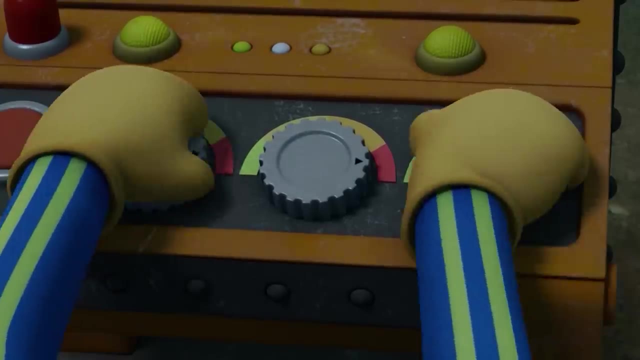 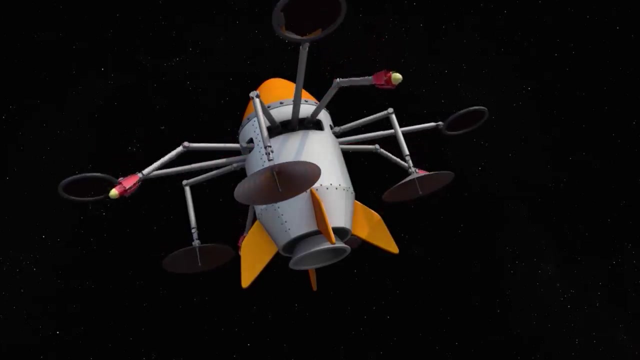 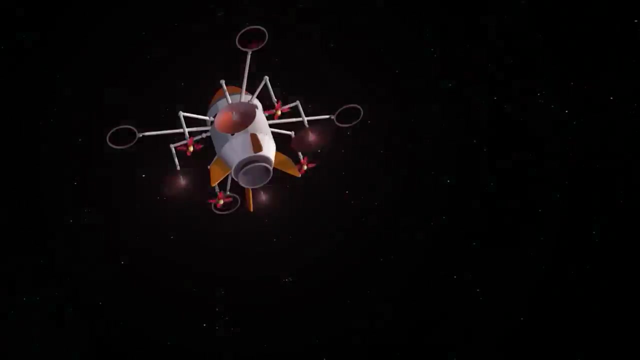 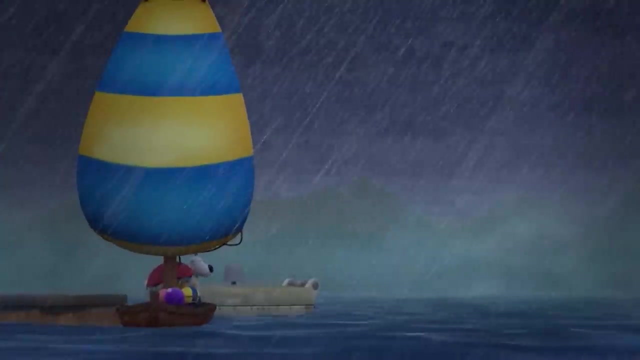 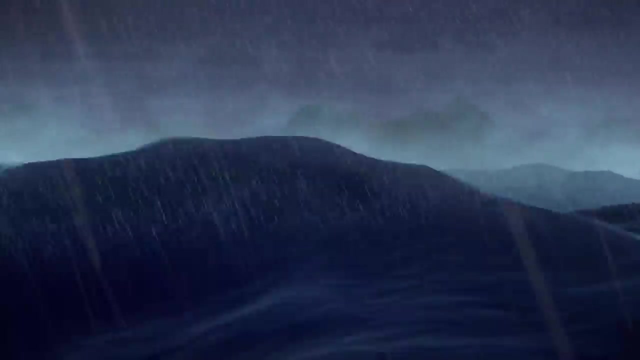 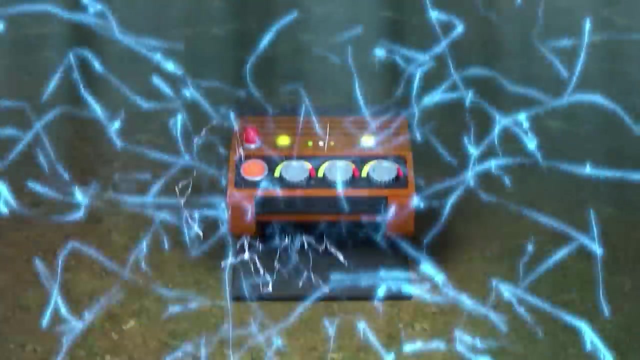 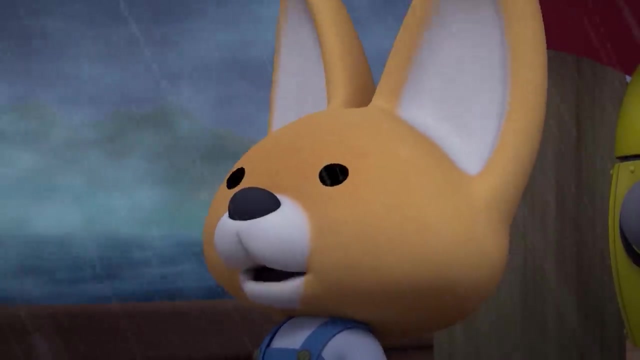 I don't know. Oh, hidden until it all stops. Wait, I did it. Oh, Oh, Oh Huh, Ahhh, Ahhh, Oh, Urgh, I think something bad's going to happen. What could happen? 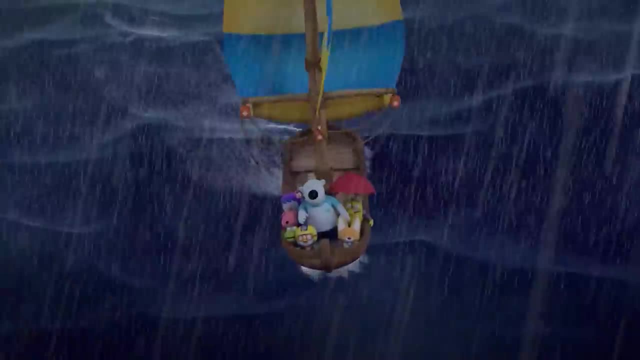 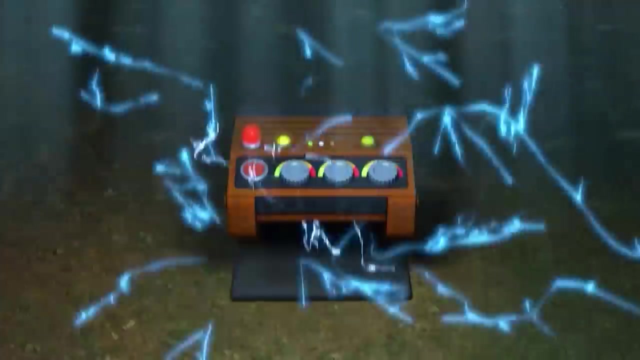 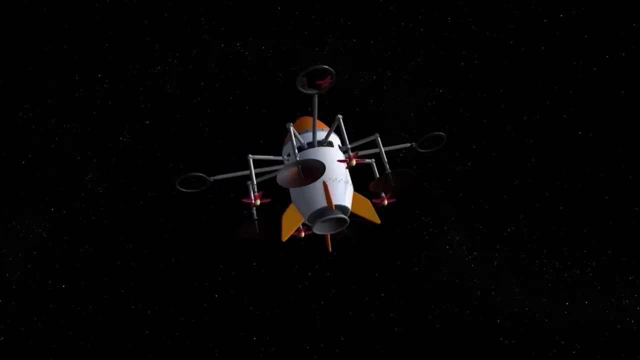 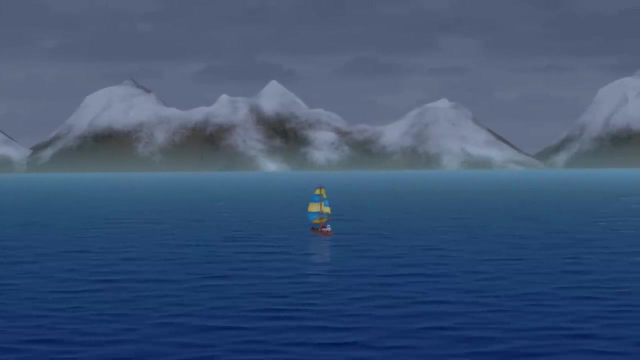 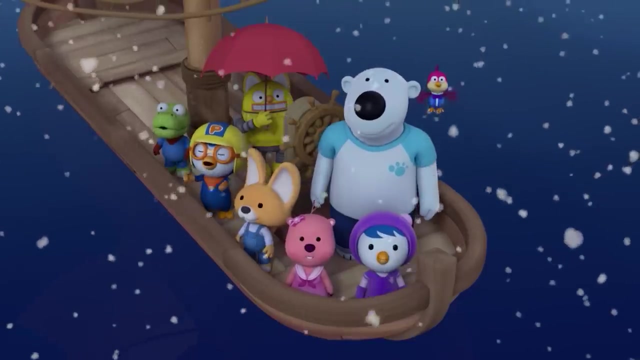 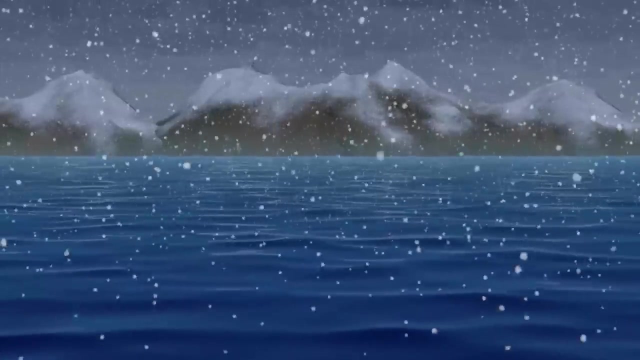 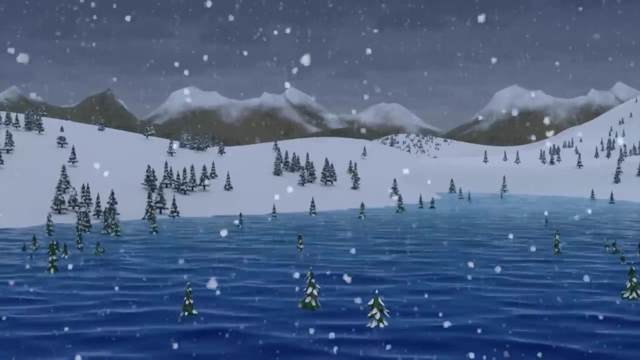 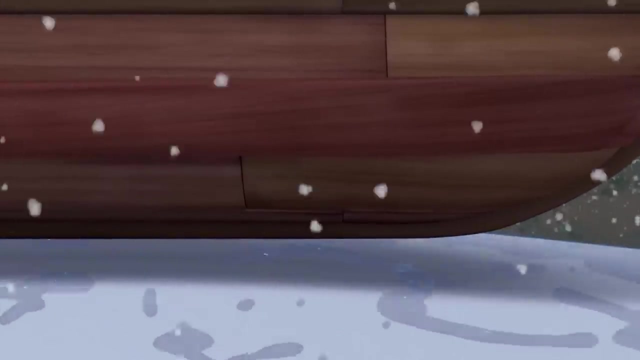 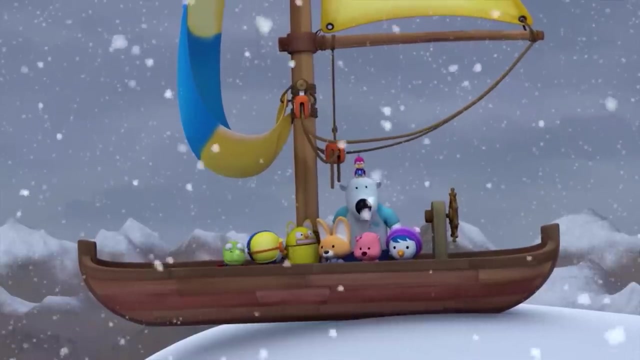 The fish are coming away. Crong Crong, It's snowing. Wow, Finally the water started going down. Wow, What a relief. Look, The water is all gone. But, guys, we're at the top of the mountain. 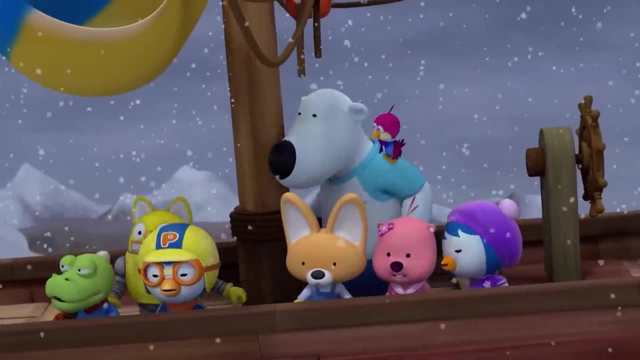 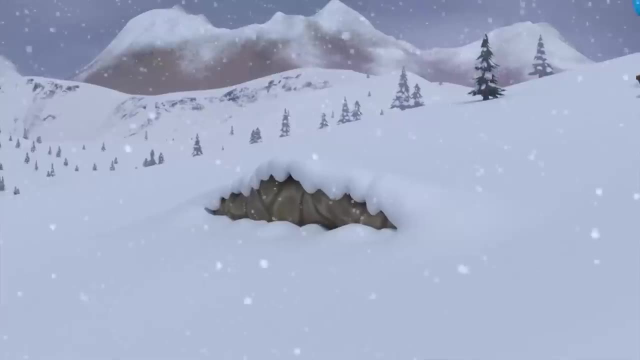 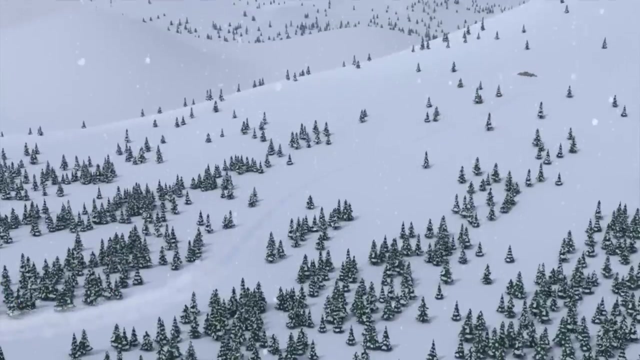 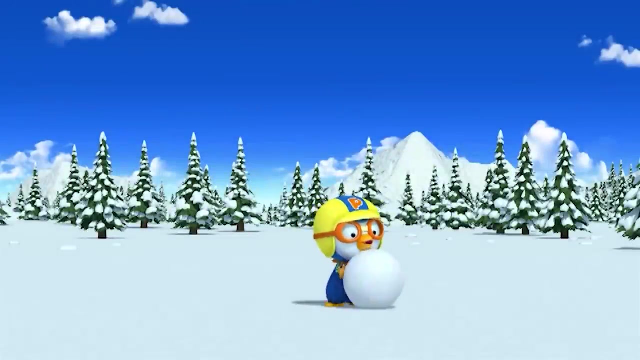 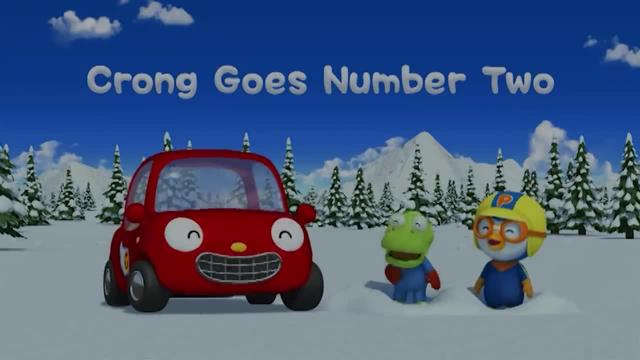 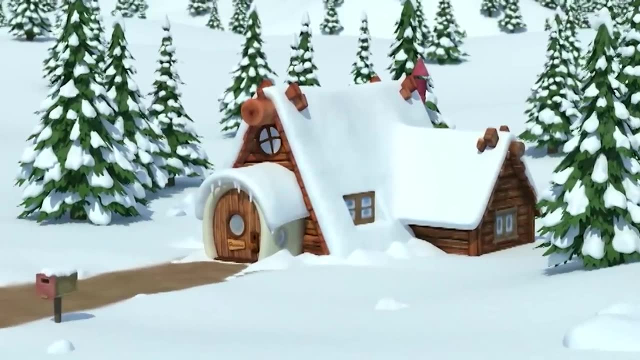 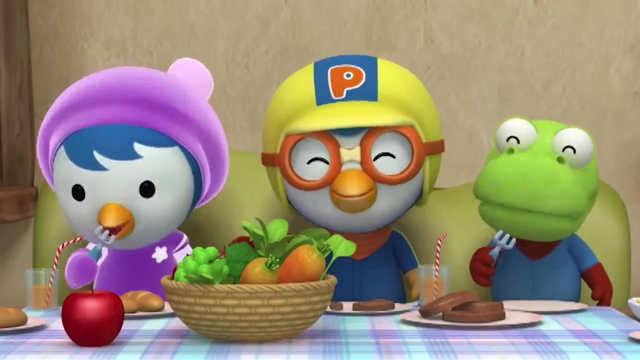 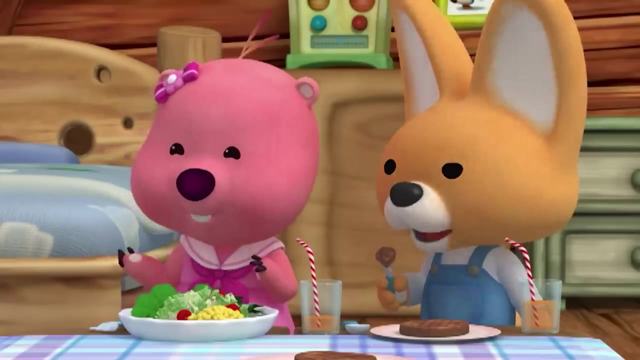 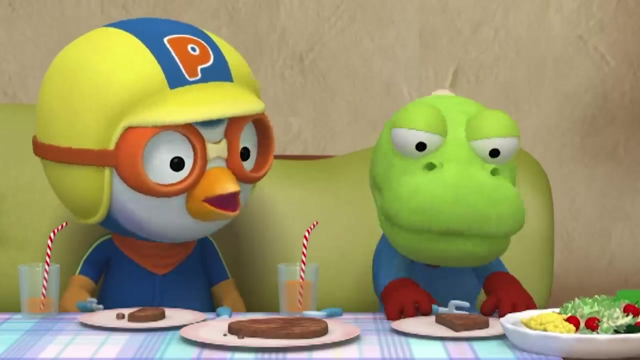 Crongles number two: Everyone is at Pororo's house. Let's join them. They're eating lunch. Wow, Crong, Crong, Crong, Crong, Crong, Crong. Very good, everyone. They're eating vegetables too. 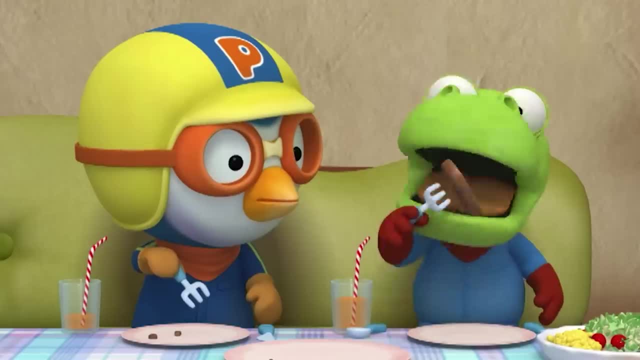 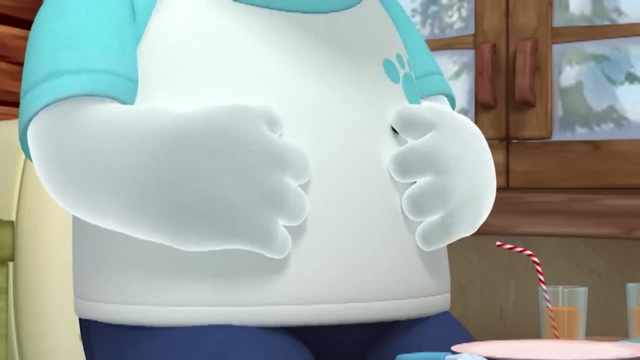 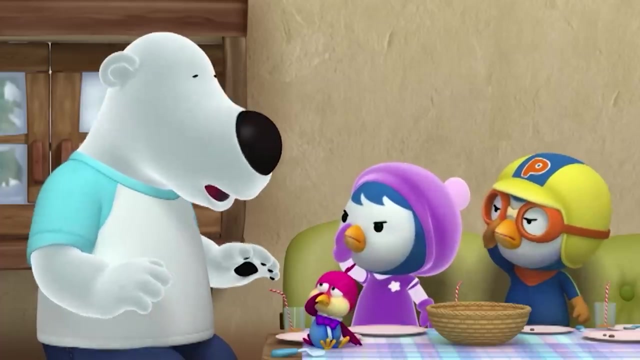 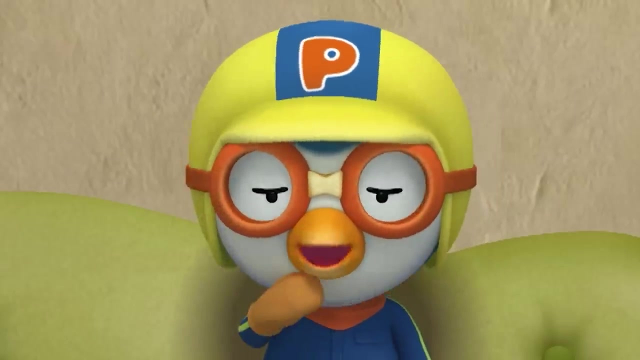 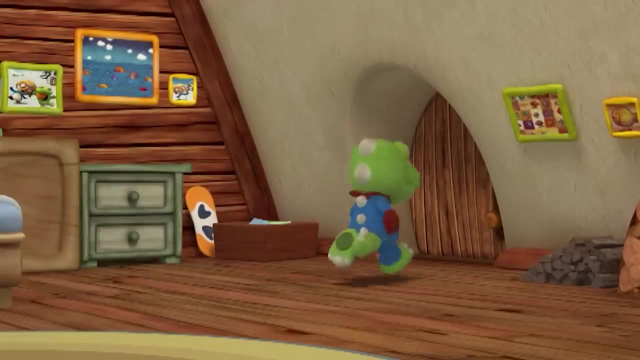 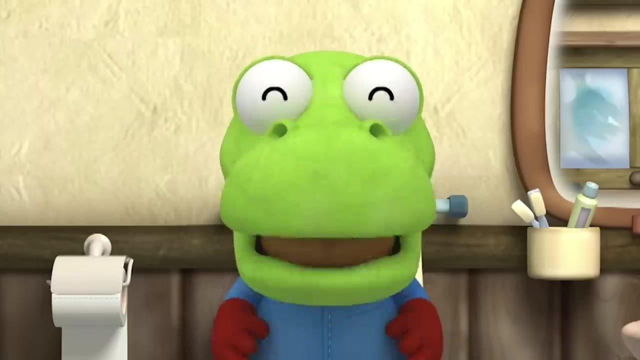 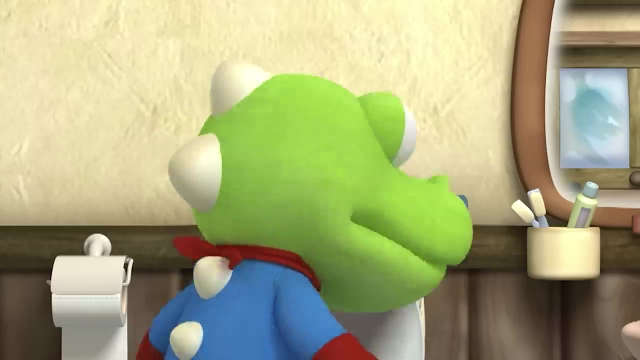 Here. Eat a balanced diet. Yummy, I'll have a little more. Uh, Uh, Ah, You're so greedy, I'm really full. That was stinky. It wasn't me, Then who? He still hasn't gone. number two: 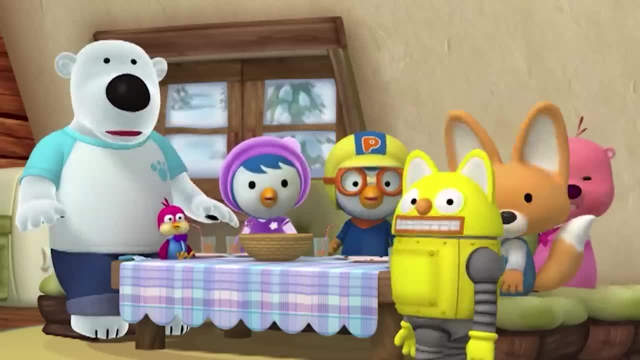 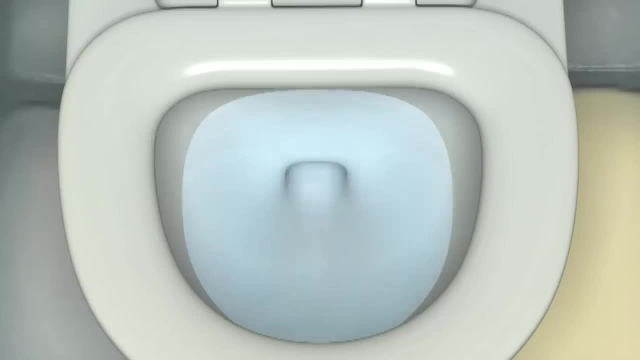 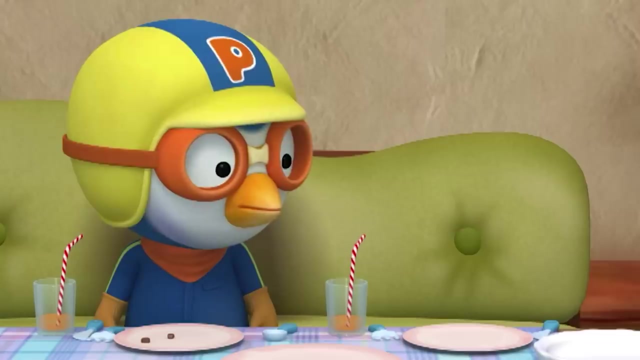 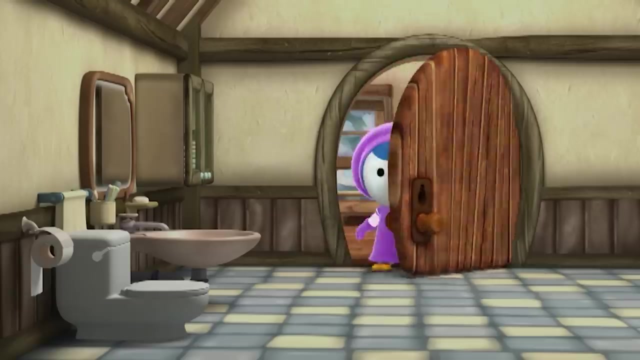 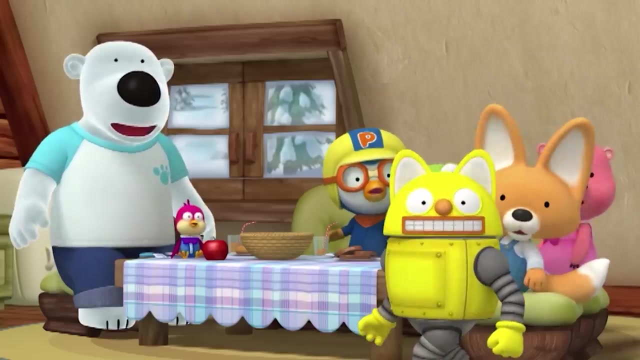 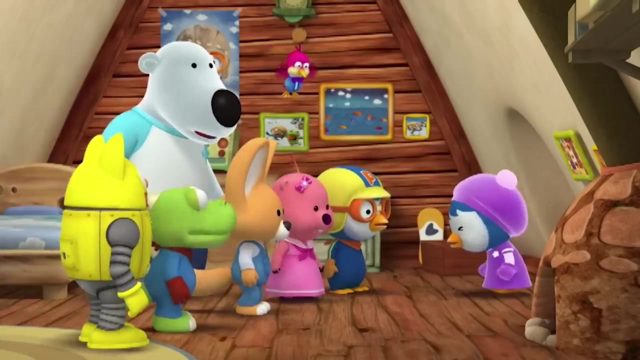 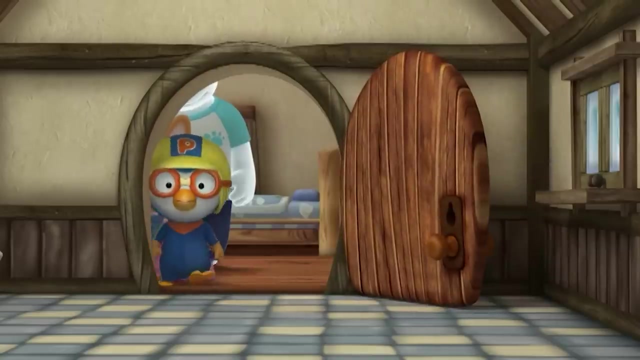 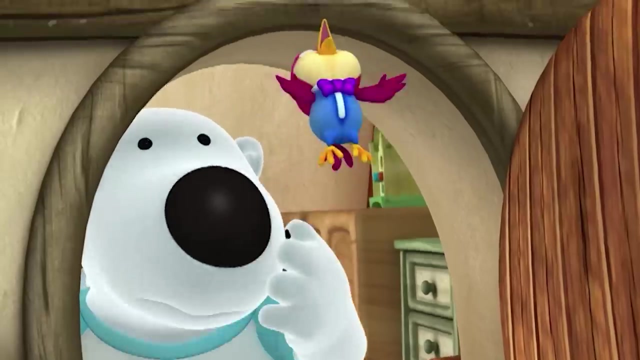 But anyway, Krong's trying very hard but he can't make number two. I'm going to wash my hands. What's going on In the bathroom? Bathroom, What is it? There's nothing here. Hurry, Close the door. 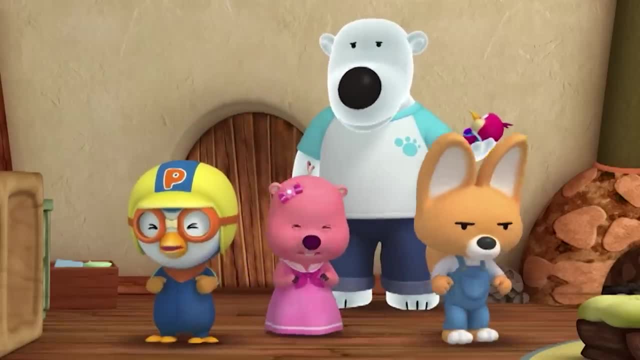 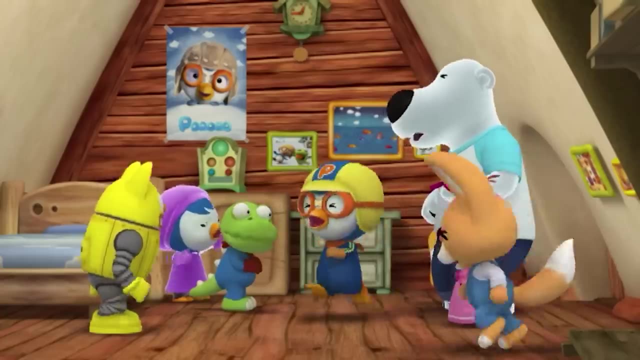 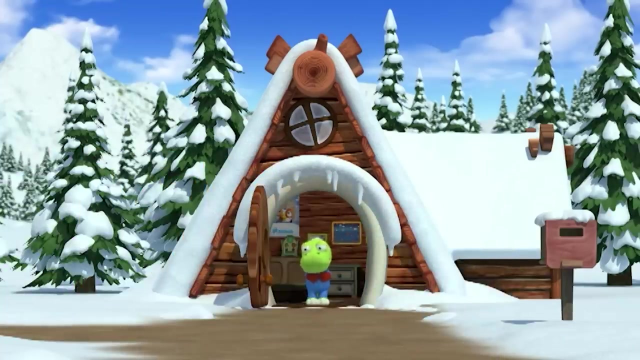 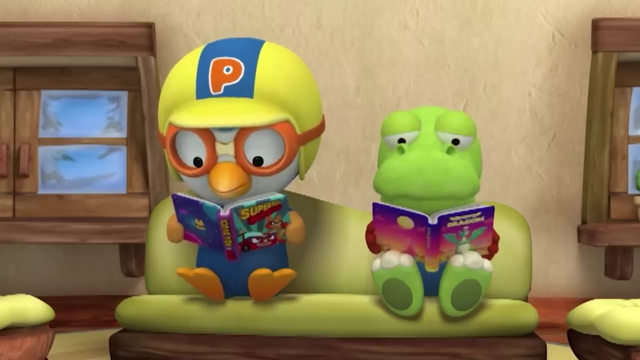 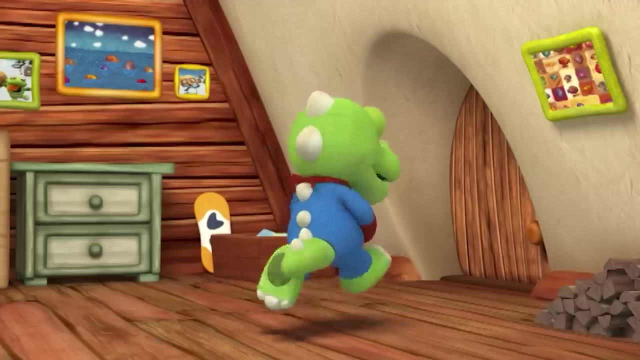 This is definitely Krong, Definitely. Oh no, Everyone ran away. because of Krong's Well er Stinky farts, The day turned into night. Krong, Are you going to the bathroom again, Krong? 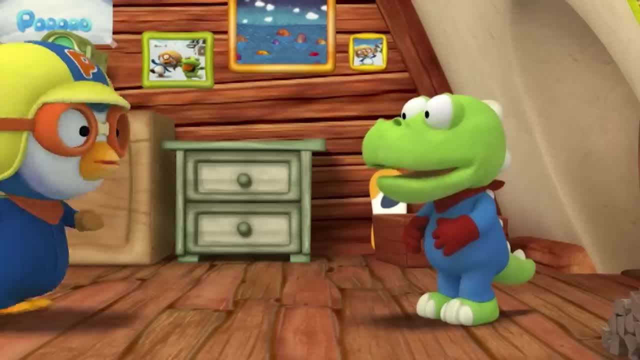 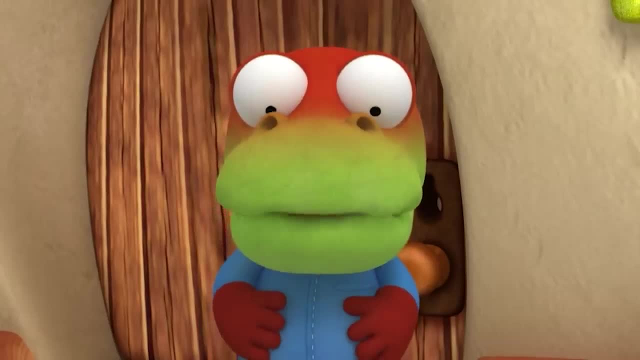 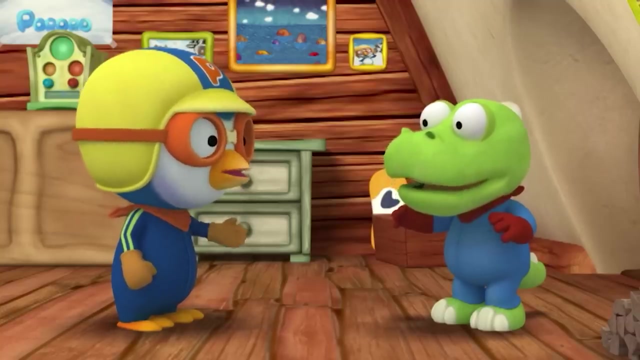 Krong, Krong, Krong, Krong. are you okay, Krong, are you okay? Ah, Huh, Ah, And I almost, I Ah, Krong, Krong, Krong. If you need to go number two, go to the bathroom. 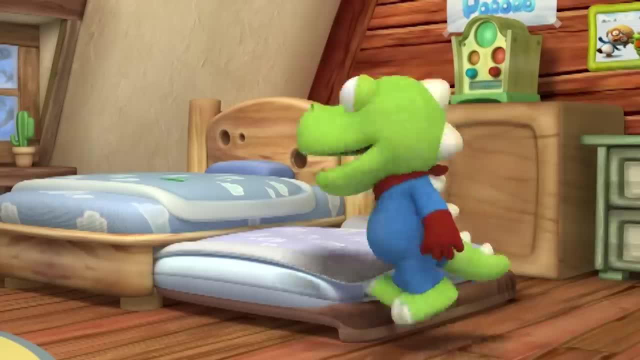 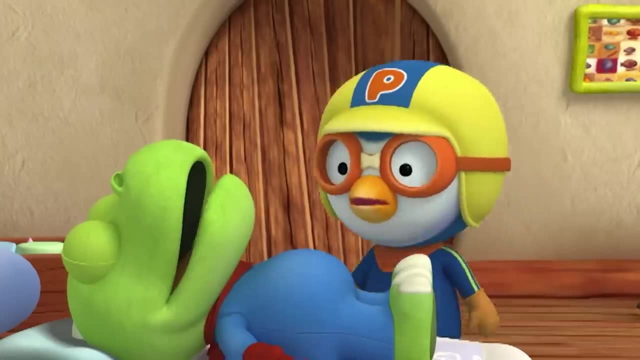 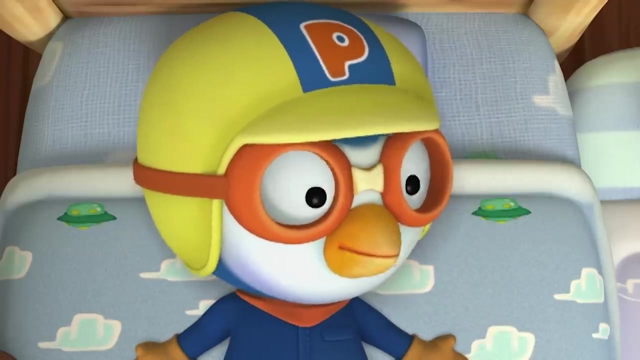 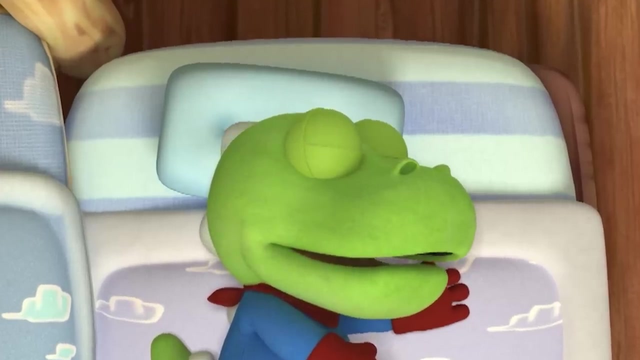 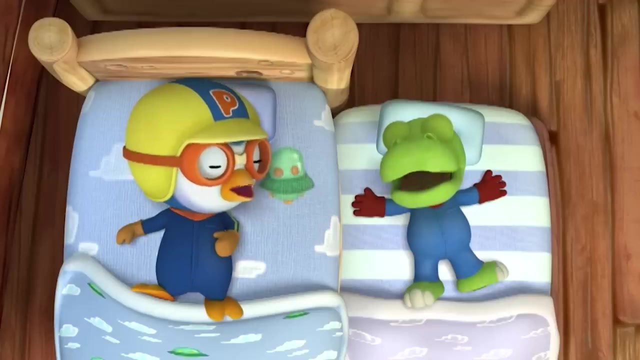 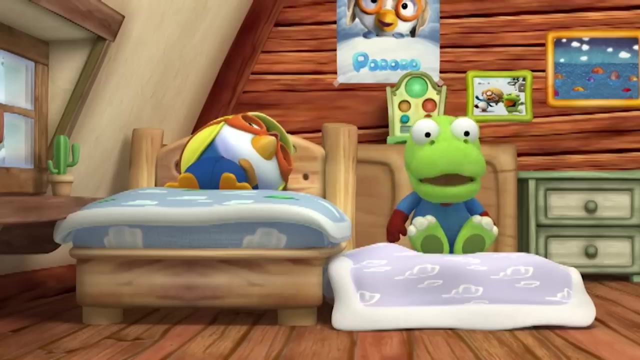 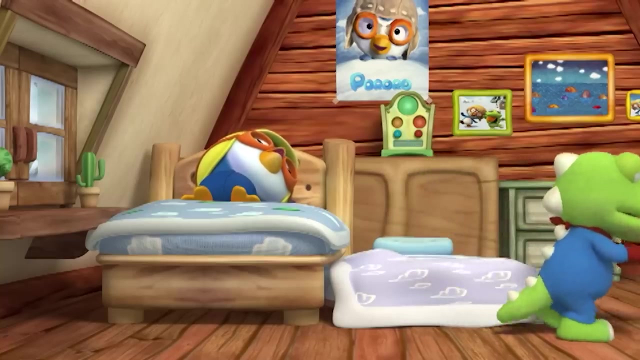 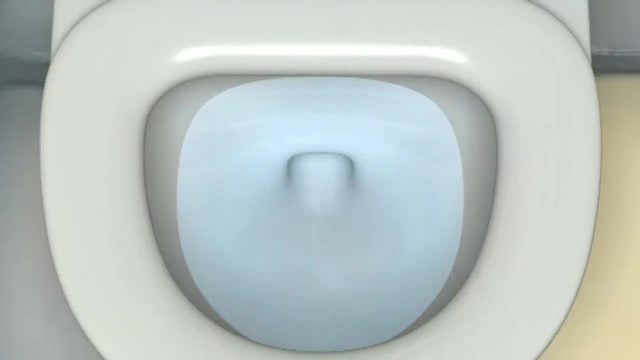 Krong, Krong, Krong, Krong, Krong. What Krong didn't want to go to the bathroom in front of Pororo? Ah, Are you okay? Well, good night, Sweet dreams. Morning came, He still couldn't make number two. 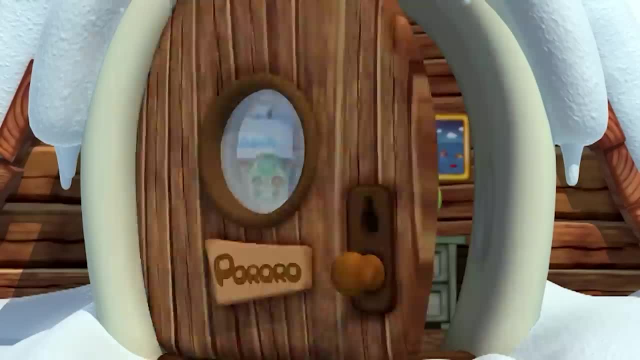 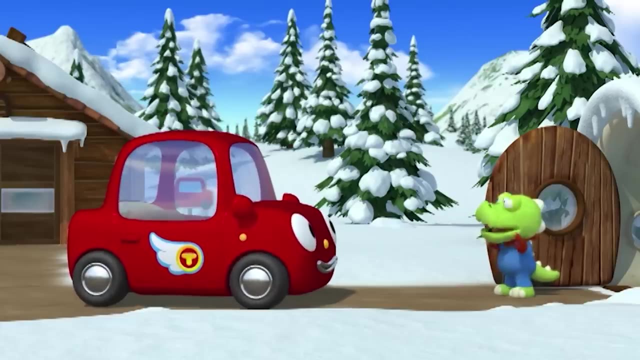 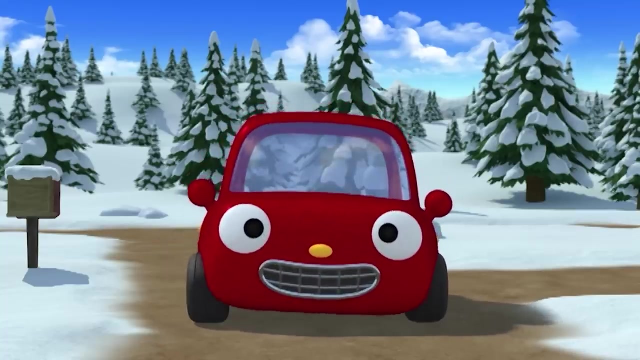 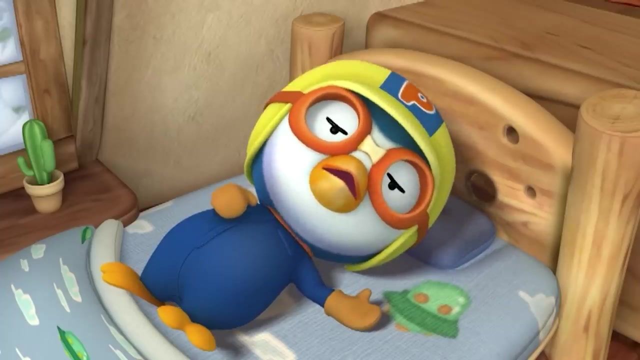 Pororo Cron. Hi Cron. Where's Pororo? Hey, Oh, he's still sleeping, But we said we were going to meet at Eddie's for a picnic. Cron Tutu gave Pororo and Cron a ride to Eddie's house. 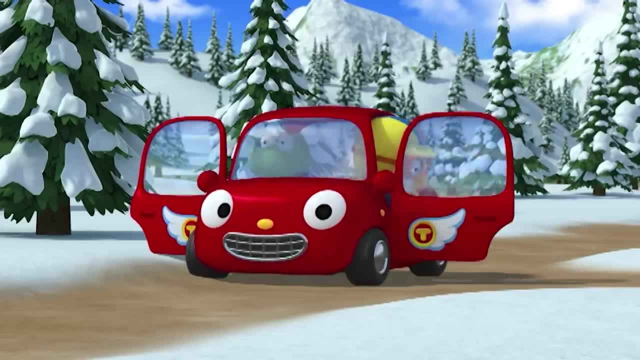 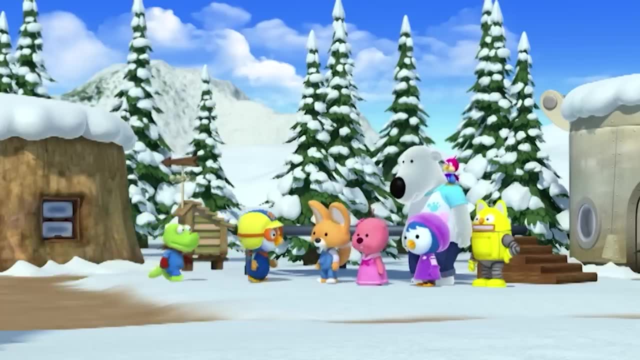 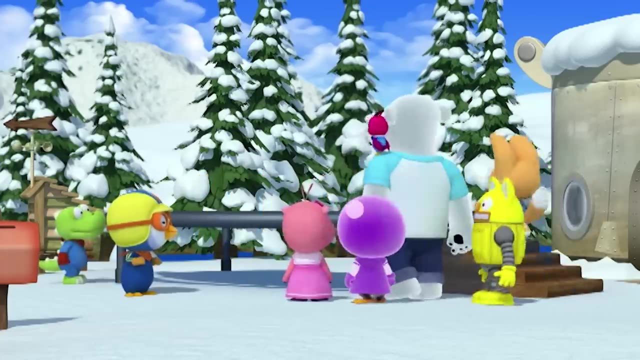 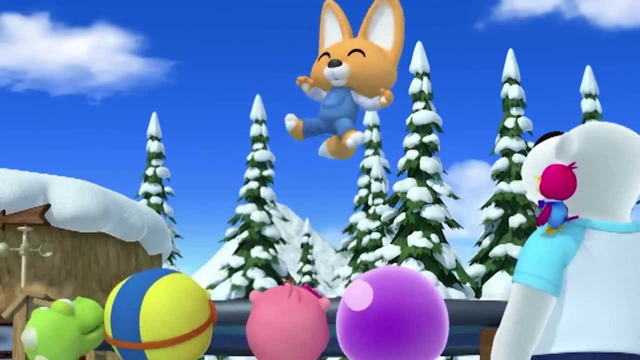 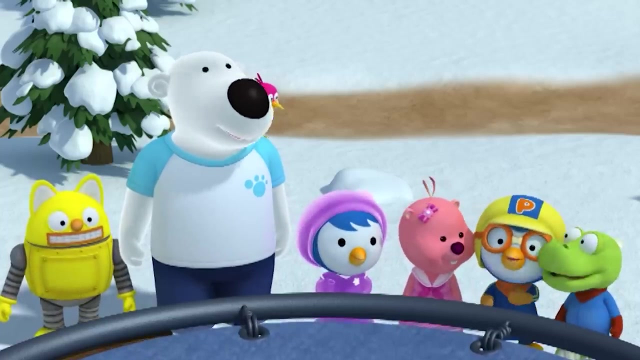 It's Tutu Hi, Tutu, Hi, Hi, Hi, Hi guys, Looks like everyone's here. What's this, What's that? Just wait right here, Watch carefully. You jump on it like this. Eddie, I want to try. 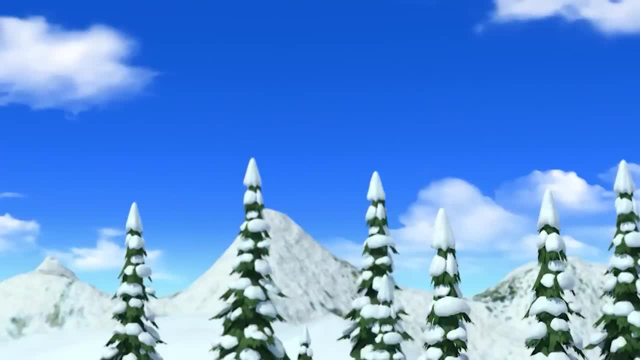 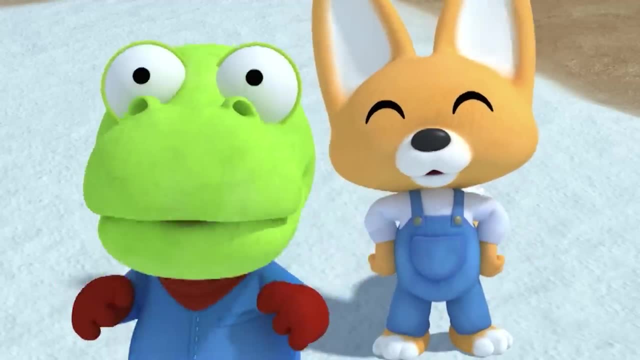 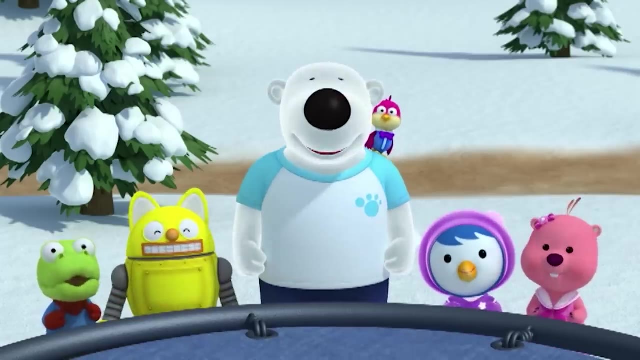 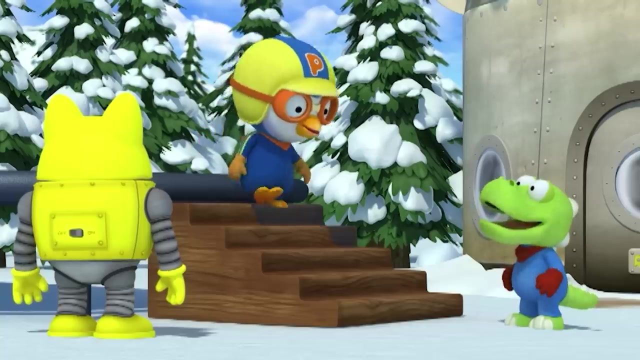 It won't fall. What Cron deposit lenght? What's that? Your diary Cron rich? Here you can take a look. Found something? Yes, that's right, We sure did. I will check. Go on, Hold on. 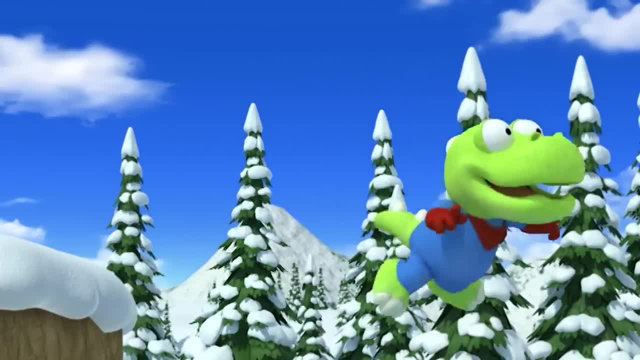 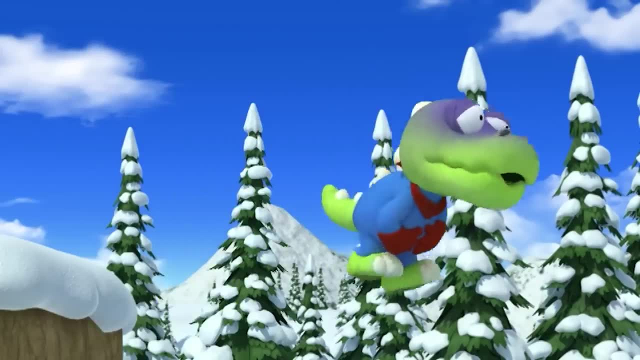 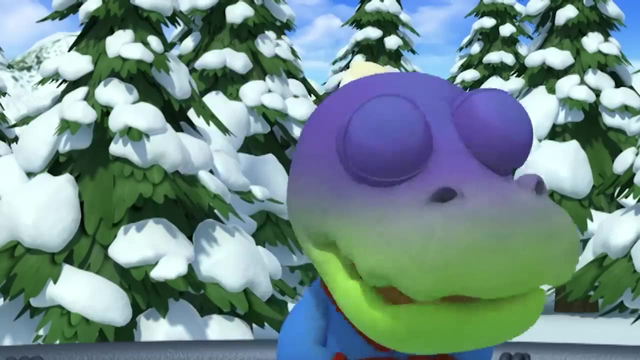 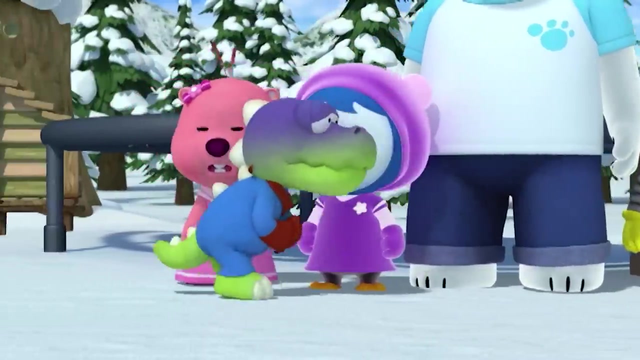 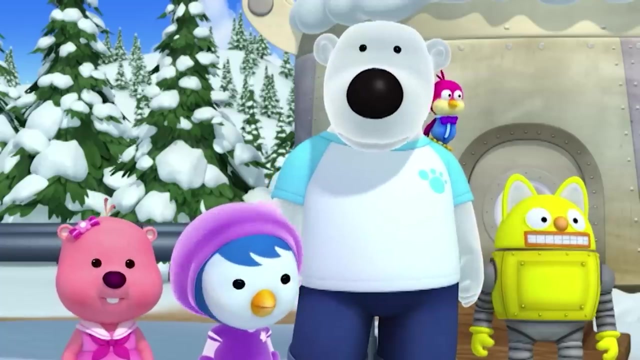 The camera is rate really low. He's here. Oh no, Krong's stomach is making strange sounds. Krong, what's wrong Huh? Hmm, Okay, it's time to go on our picnic. Wow, Yay. 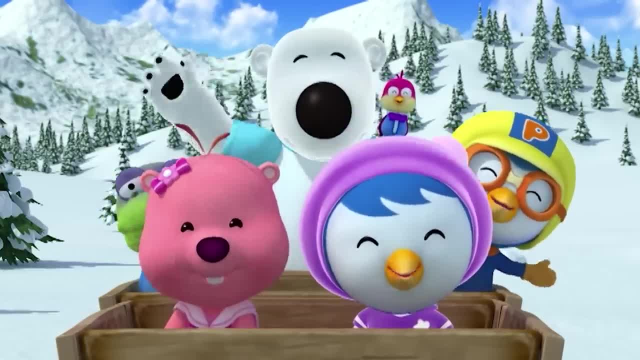 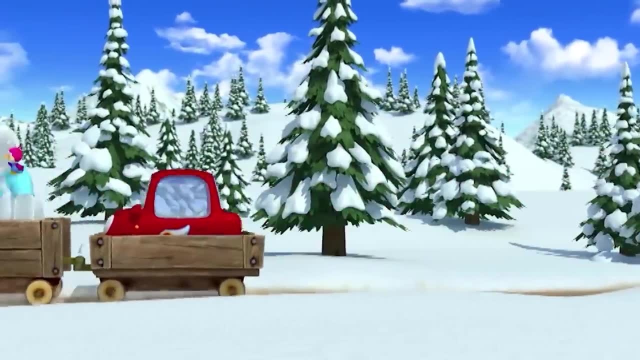 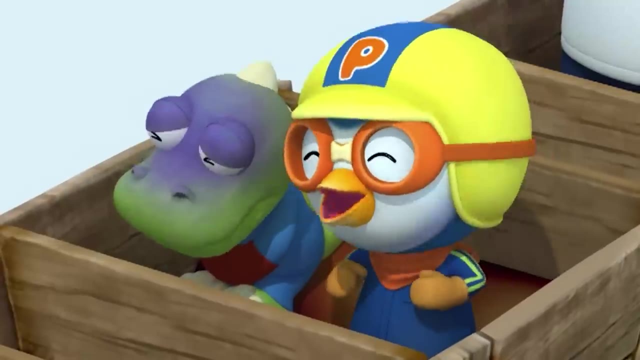 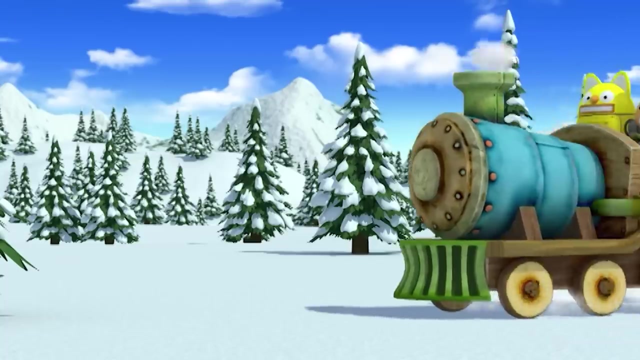 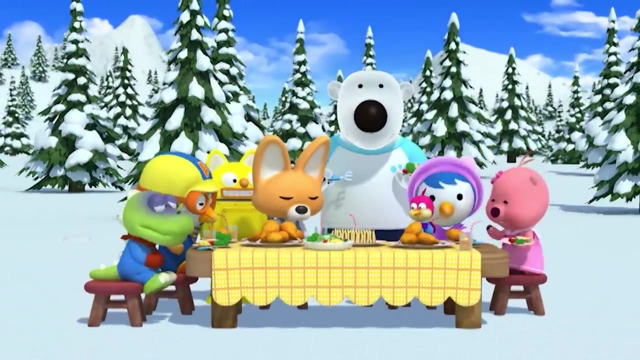 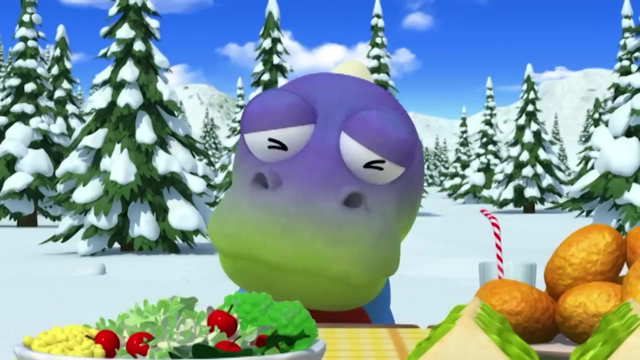 I'm excited. Is everyone ready? Yes, Then off we go, Off we go. They are going on a picnic and they are in a great mood, All except for Krong, whose stomach is hurting. Oh dear, Oh dear. 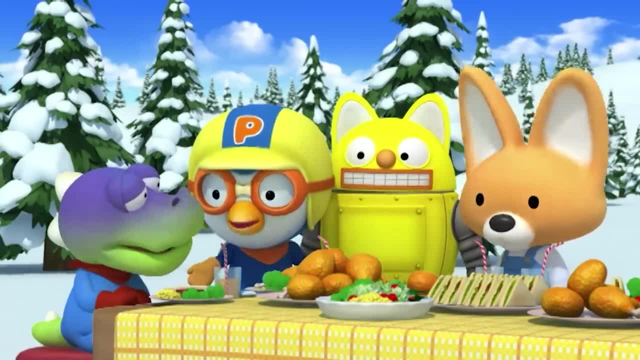 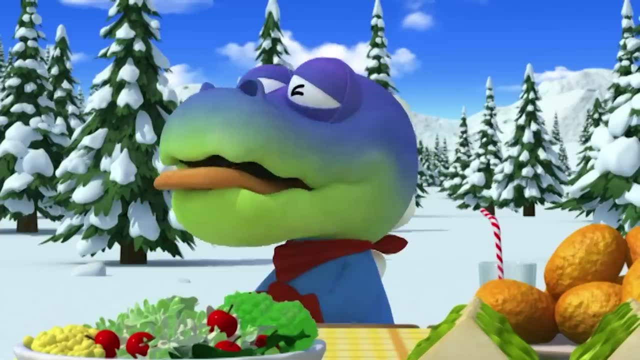 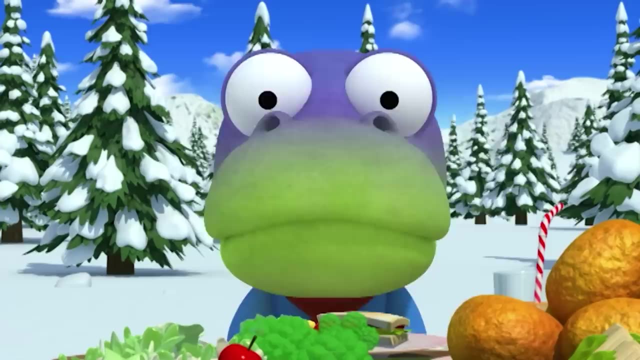 Krong's stomach is hurting again. Krong, are you okay? Yeah, Krong. Krong didn't want his friends to know that he needed to go number two. Are you really okay, Peña? you don't look so good. 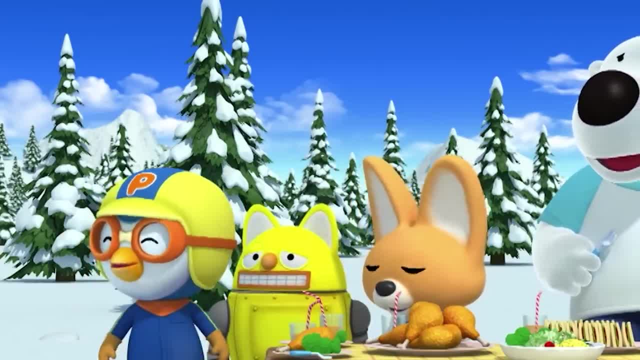 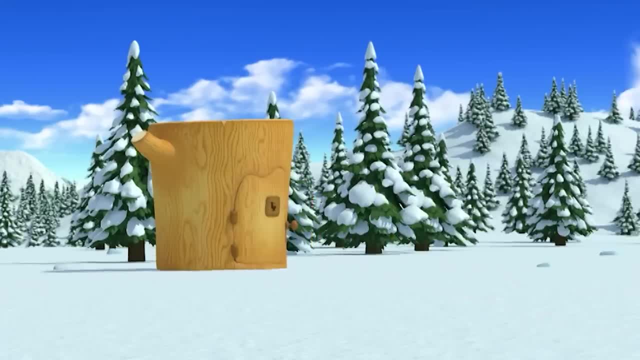 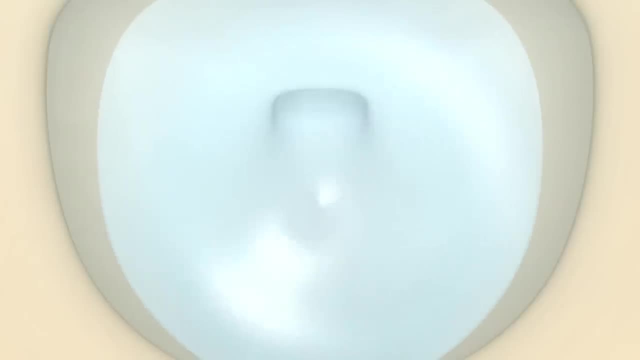 He has to go again. Krong is a regular pooping machine. I don't think Krong is feeling too well. Poor Krong, He still couldn't make number two. Krong, Krong, Krong, Krong, Krong. 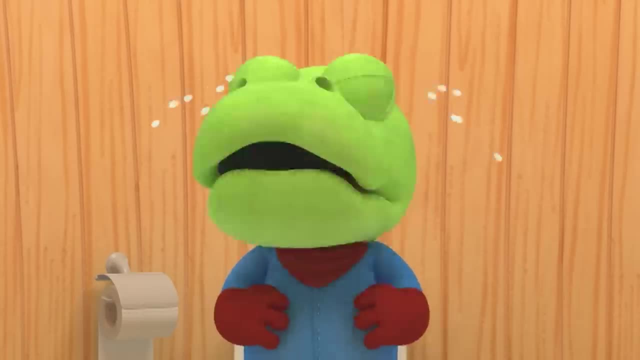 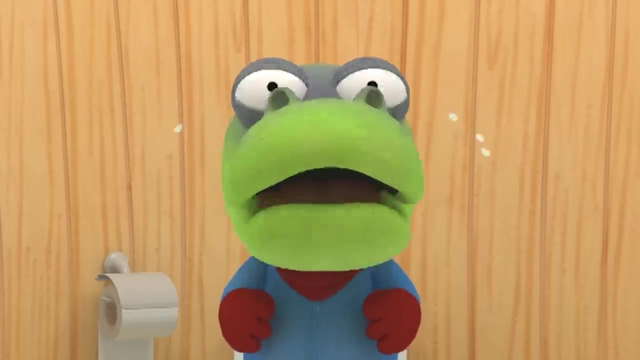 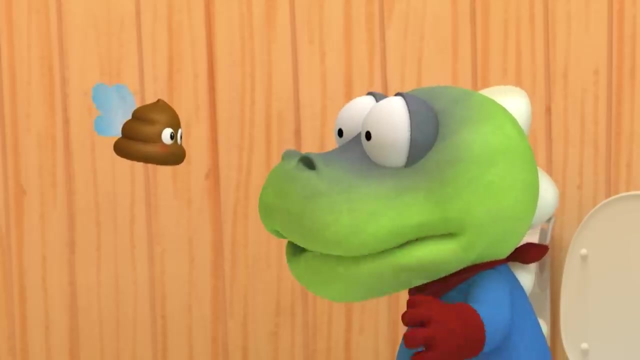 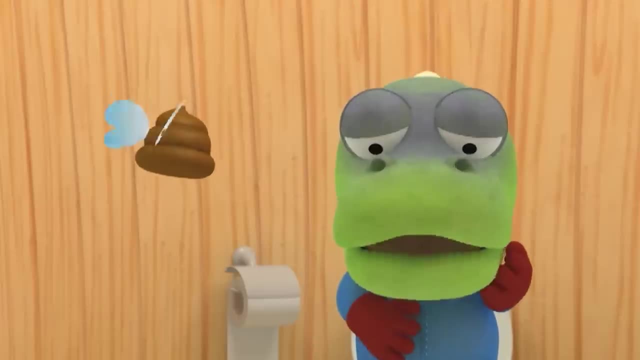 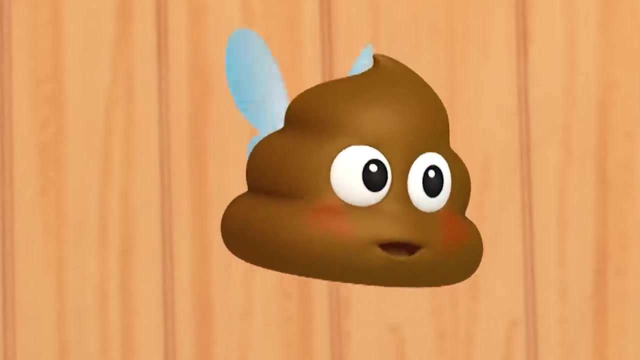 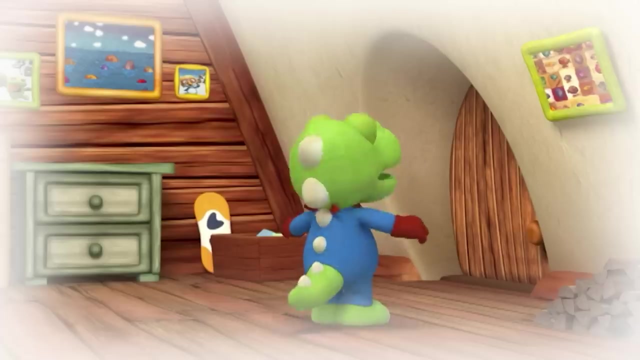 I'm the poo-poo fairy, But why are you crying? Your tummy hurts, but you can't go. Hmm, Do you want to know why that is? It's because you only ate meat and didn't have vegetables, And every time you had to go, you waited and didn't go. 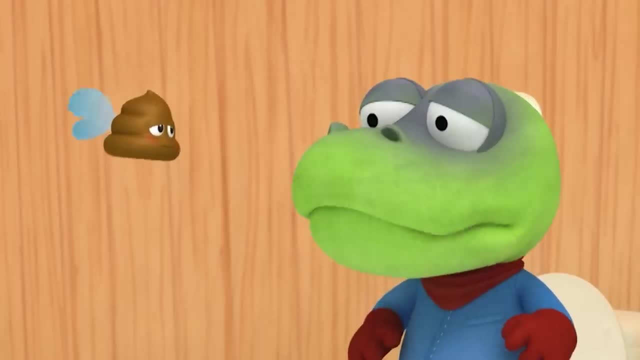 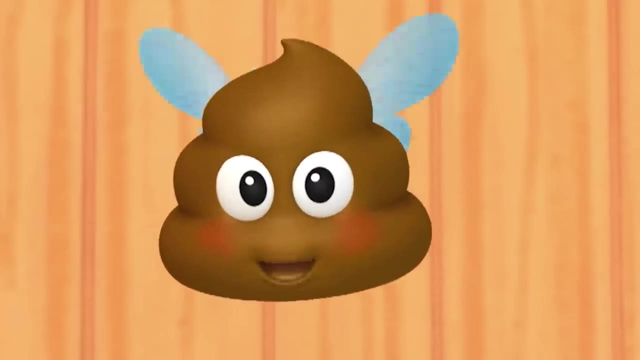 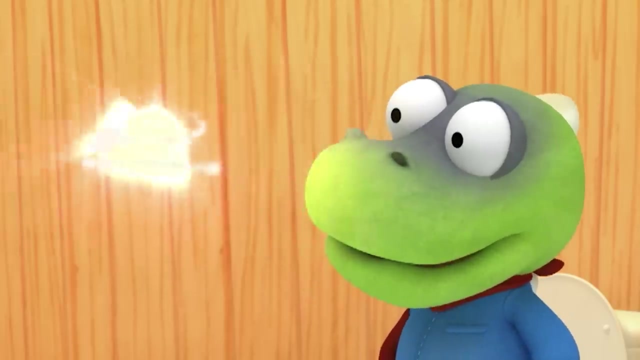 So that's why you can't make number two now. It's not hard to make number two. Just eat vegetables And when you have to go, go to the bathroom right away. Think you can do it All right, Then I must be off. 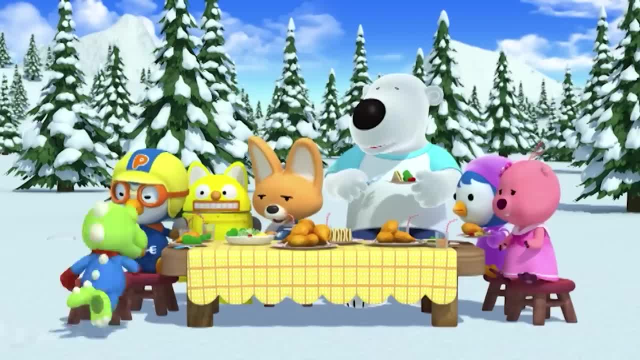 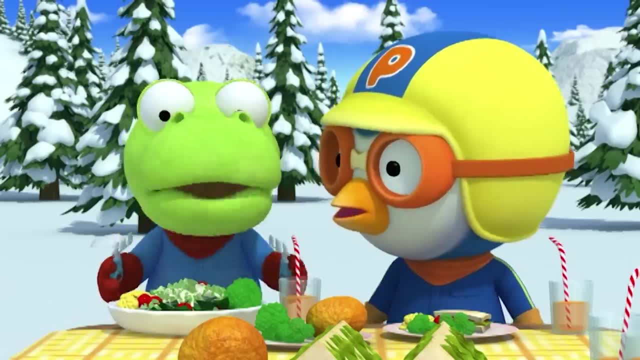 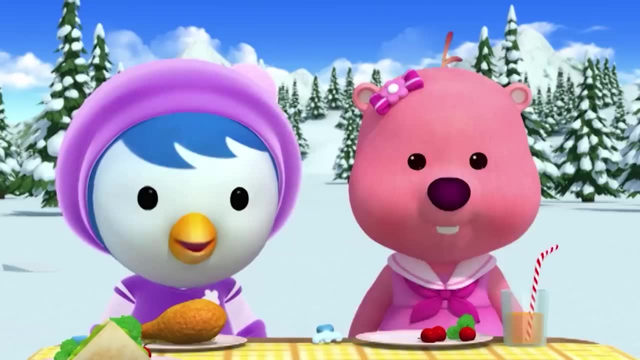 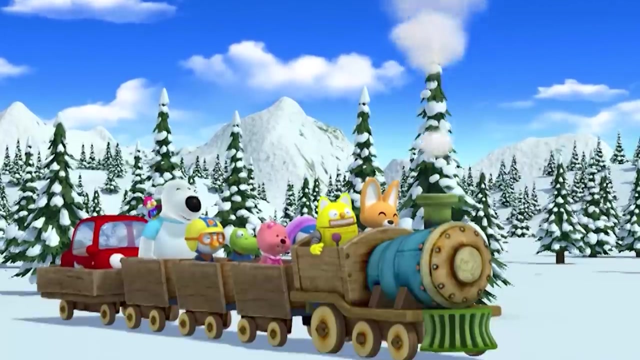 Krong was so happy to know how to make number two. well, Krong, do you feel good? He's eating vegetables. Krong Krong, ate all his vegetables. Krong Krong. Okay, now let's go, Let's go. 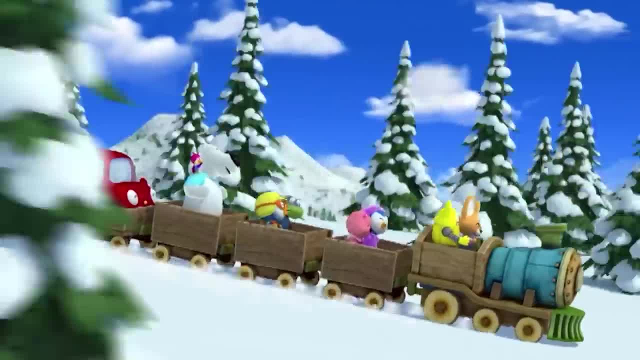 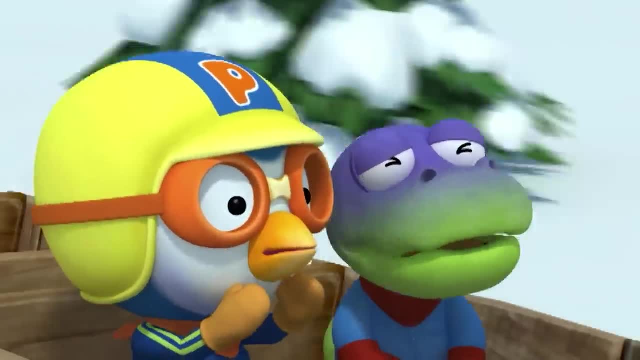 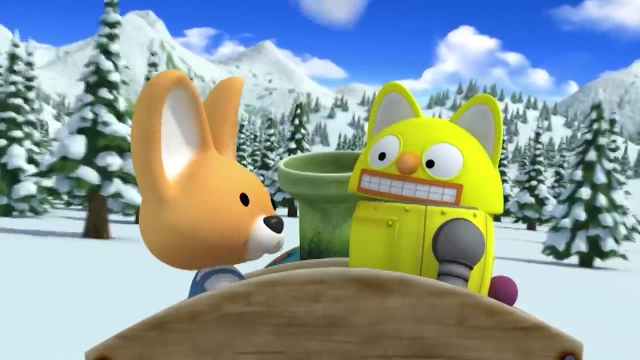 Whoa, Yeah, Krong, Krong, Krong, Krong. Okay, hurry, Krong really needs to go to the bathroom, So hurry. You got it, Brody, let's go faster, Okay, Whoa. 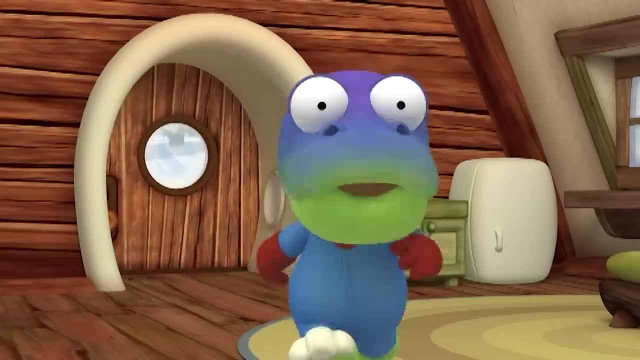 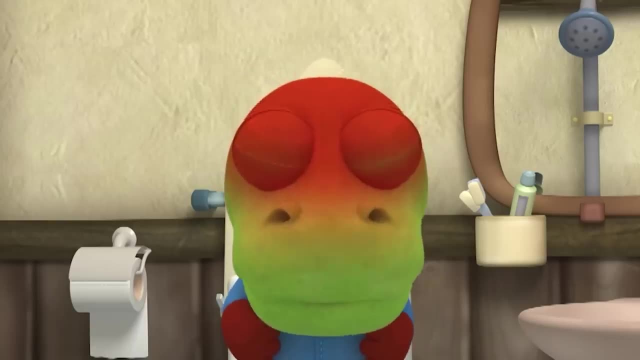 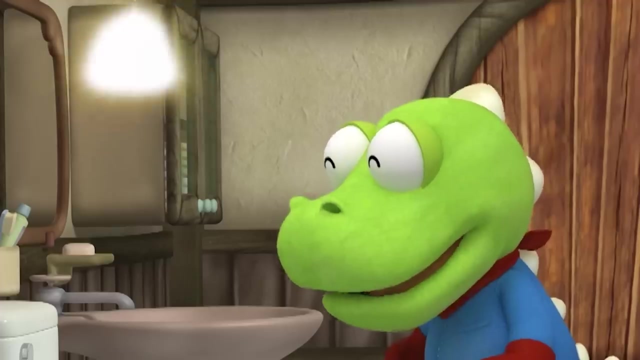 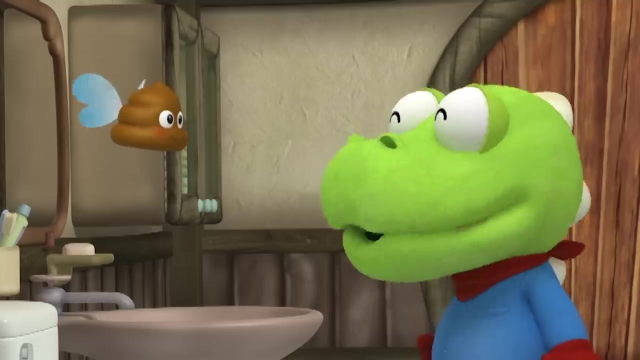 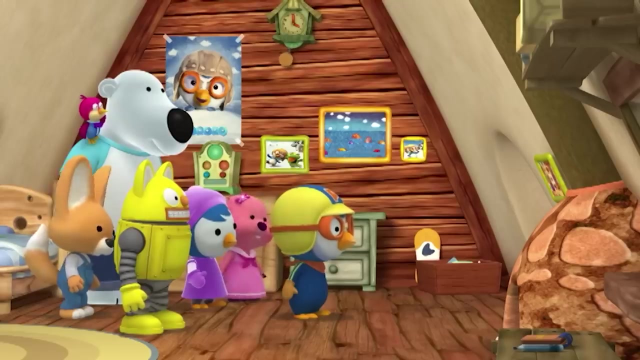 Everyone arrived at Pororo's house. Finally Krong went. number two: Krong Krong. Good job, Krong, Krong Krong. Bye, bye, Krong, Krong, Krong Krong. did you go, number two, Krong, Krong Krong. 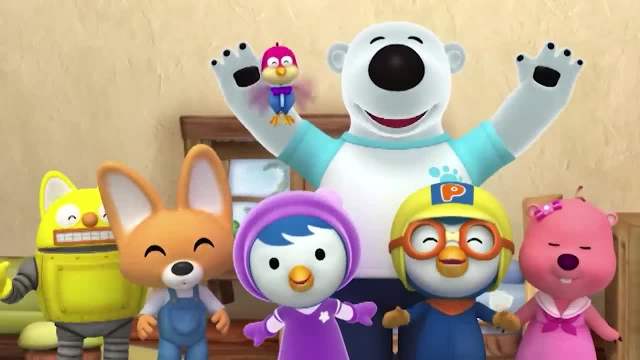 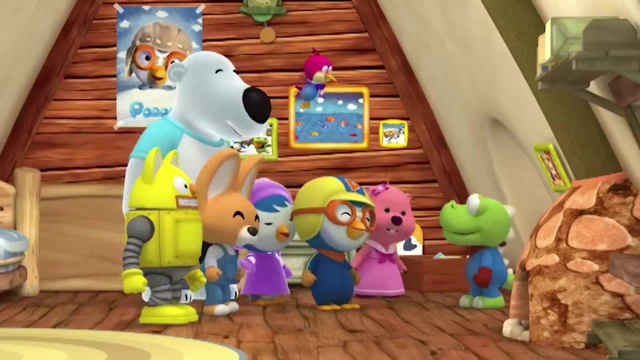 Krong, Krong, Krong, Krong, congratulations, Good job. I was worried, but now I'm relieved. you went. Good job, Krong. Good job Krong. My crumb is much calmer now. Now, Krong is an expert at making number two. 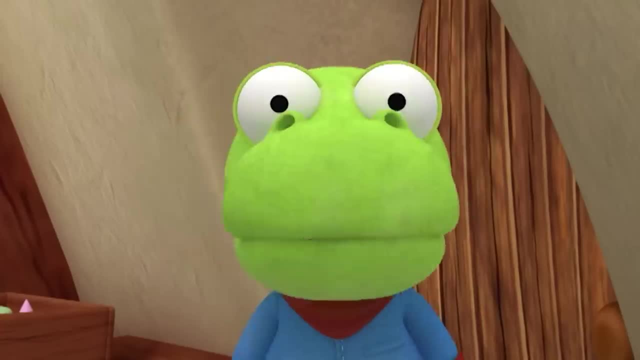 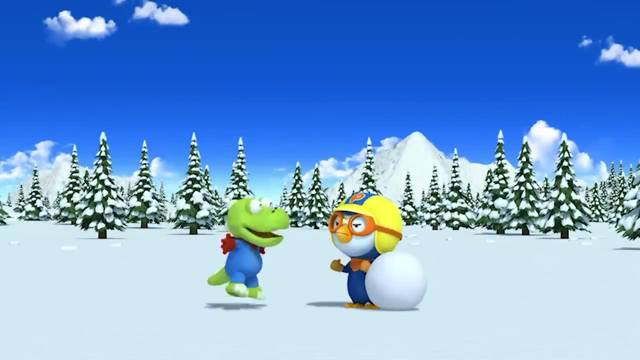 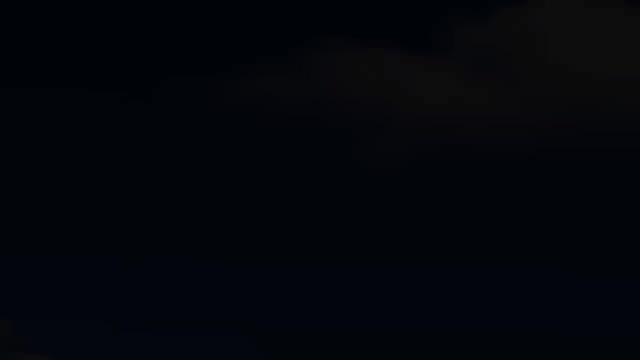 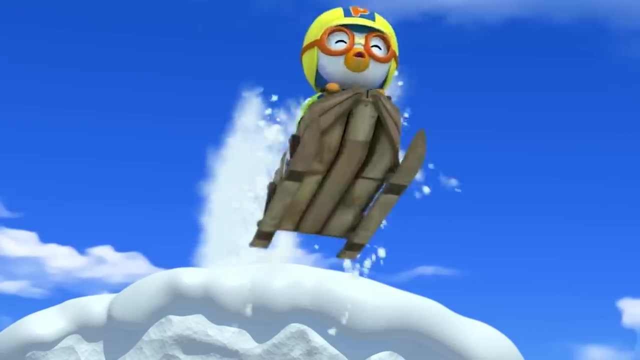 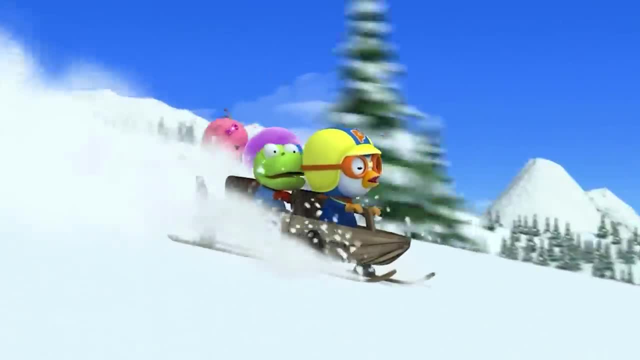 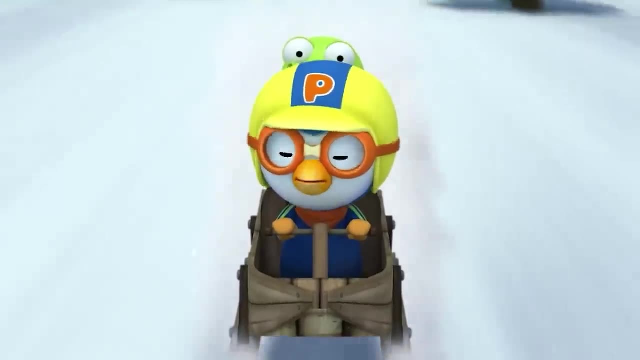 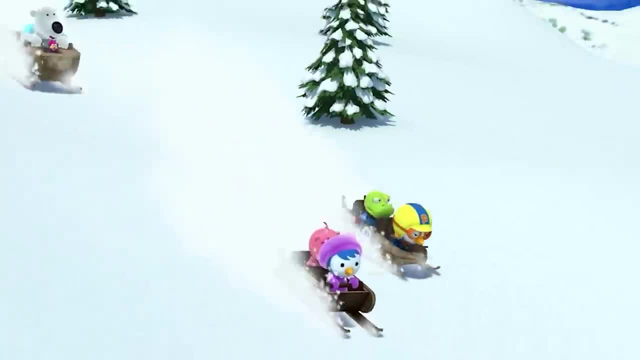 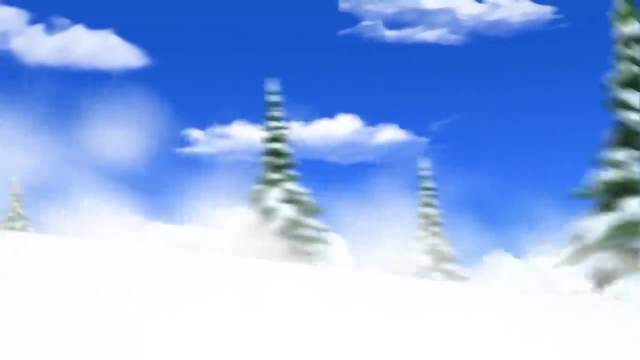 Hey, hey, yippee, Move out of the way. Oh, Oh, Pororo, Whoa, We got worse place? I don't think so. We're first. No, We got first place. What, What's that sound? 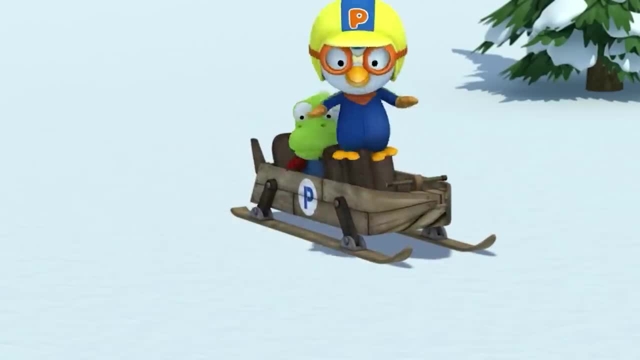 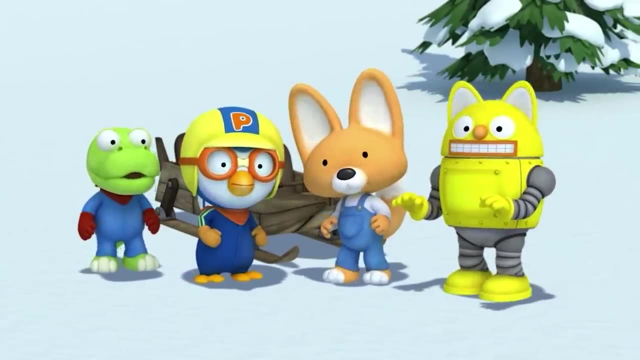 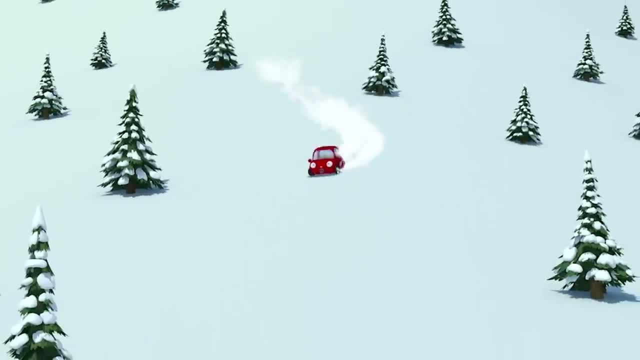 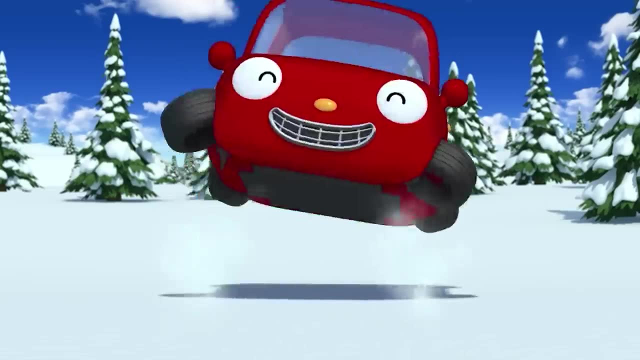 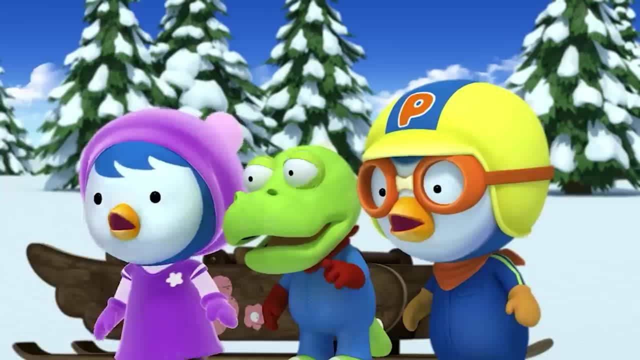 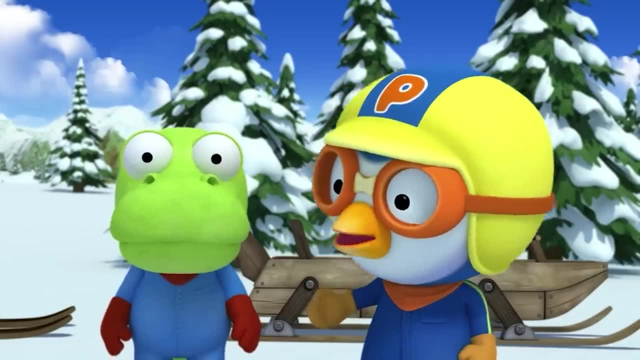 Whoa, Whoa, Oh, Hooray Cool, This is fun. Ha-ha Huh, I've covered you in snow, I'm sorry. Whoa, What? Whoa? They're paradox, Don't be surprised. 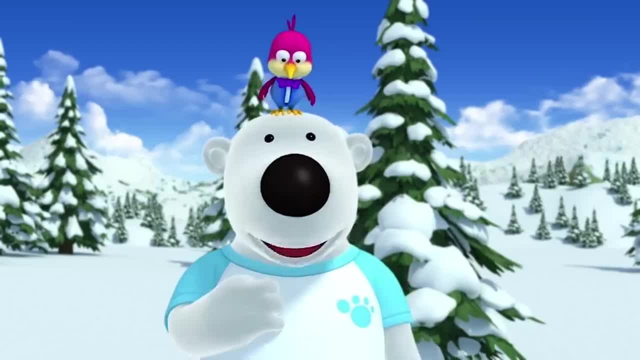 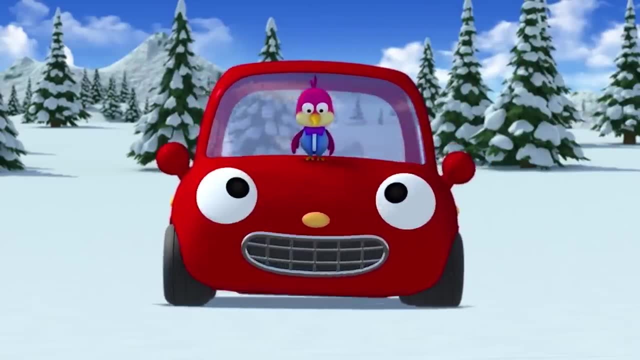 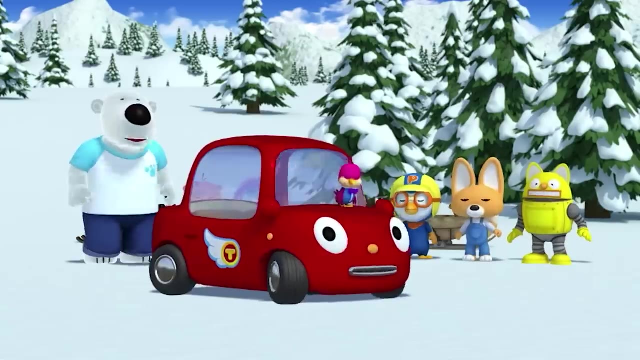 Who are you? Me-huh, I'm Pororo. This is Krong Krong Krong. Huh, What's your name? I'm Tutu. That's a nice name. Huh, It's an avalanche. 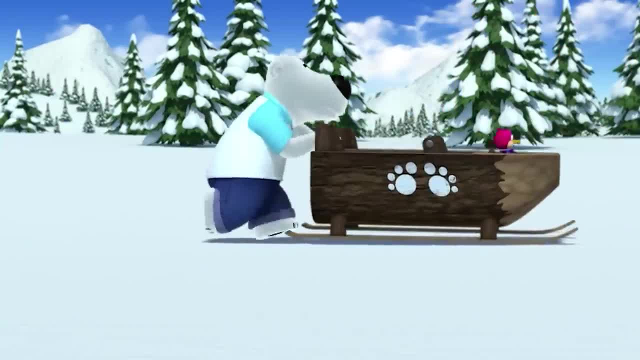 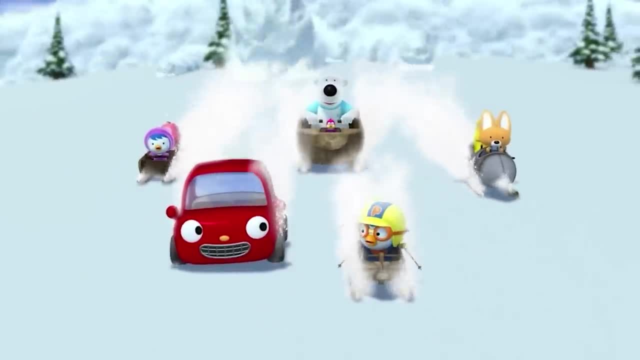 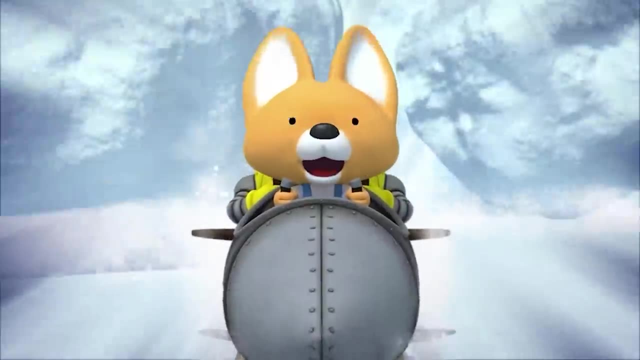 Let's go. Let's go. Oh no, Oh no, Oh no, Huh Huh, Oh no, Oh no Huh, Whoa, Whoa, Whoa There, Get behind that hill. 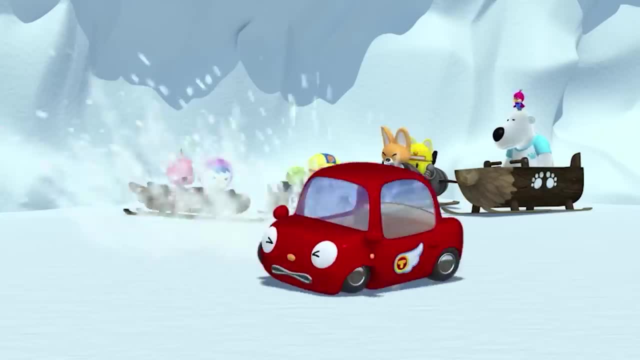 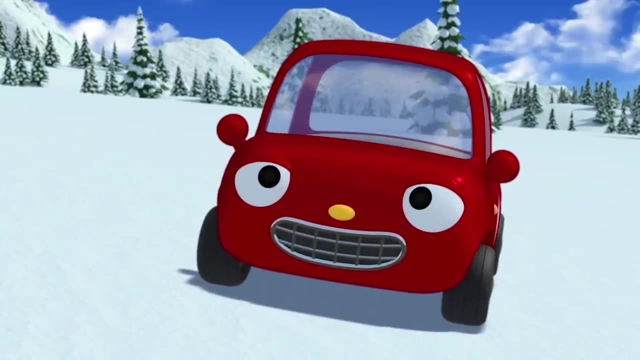 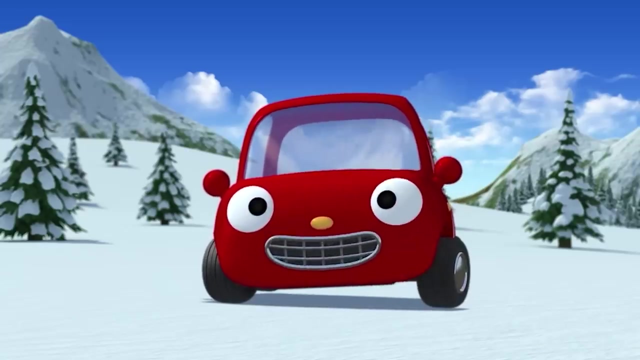 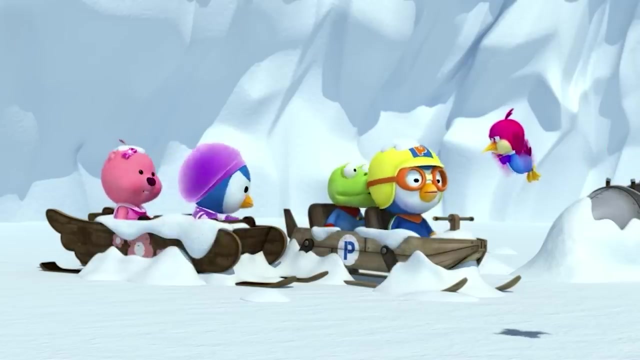 Relief: Whoa, I'm safe. What a relief. Phew, Huh, Oh no, Everyone is covered in snow again. Huh, What's wrong? It's all your fault. Let's go home, Okay? Bye-bye, Tutu. 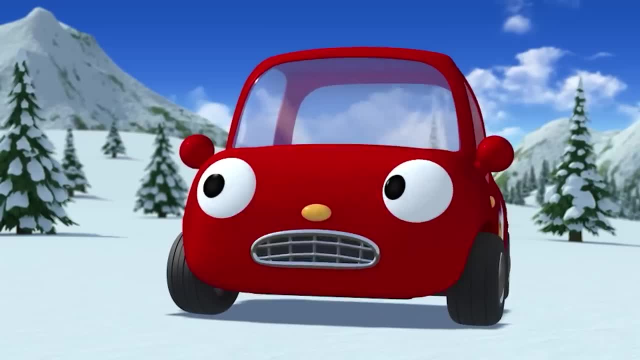 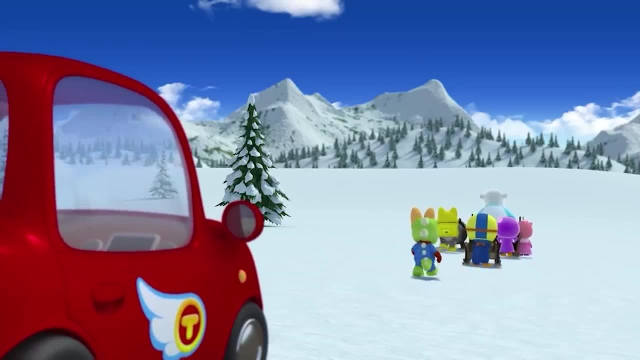 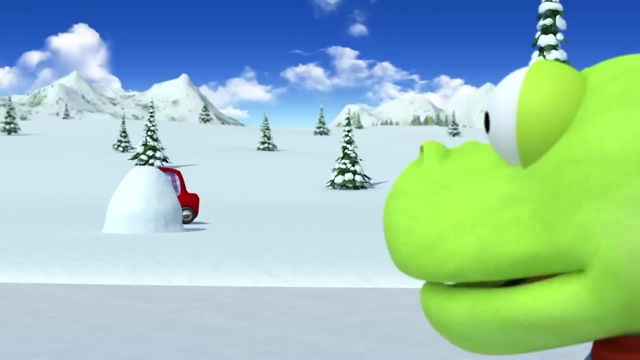 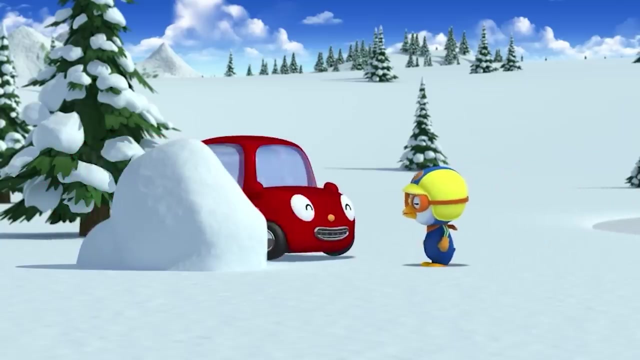 See you, Crong-crong, Bye-bye, Crong Dum-dum-dum-dum, Crong, Crong, Dum-dum-dum-dum, Crong Tutu, Where do you live, Tutu? 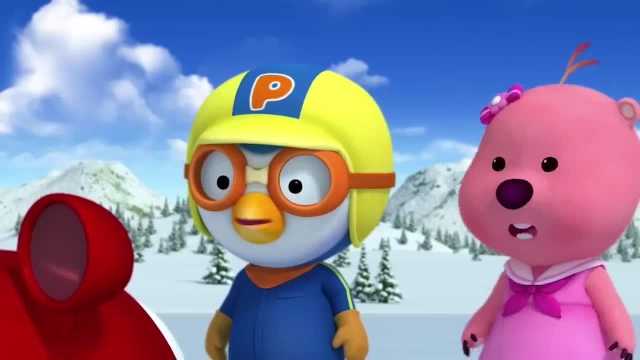 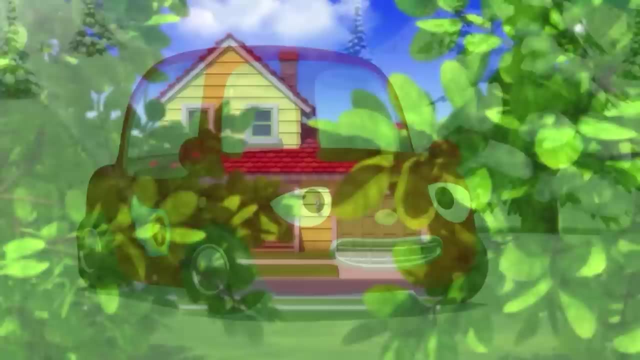 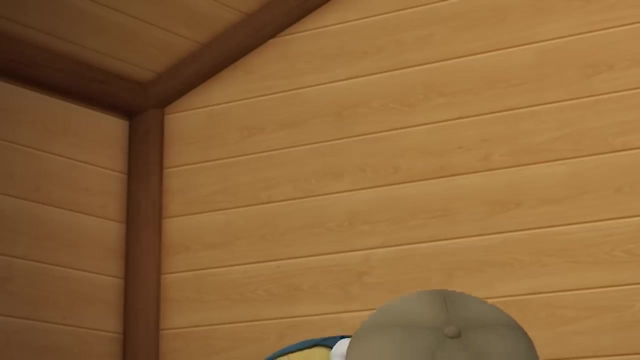 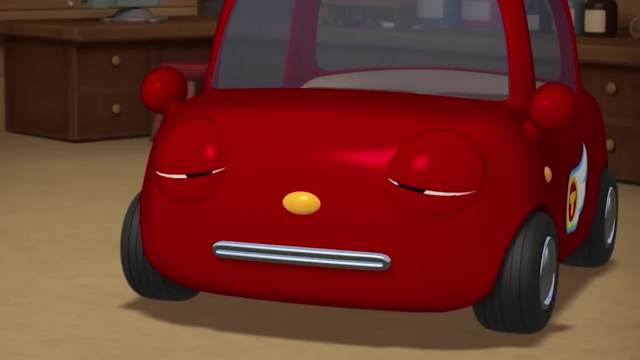 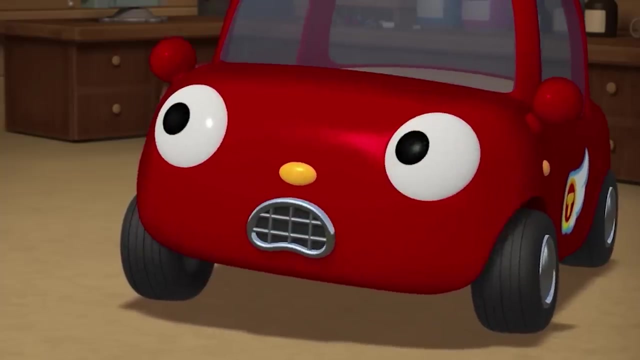 I live really far from here, Then how'd you end up here? Well, Tutu came from that house. There It's done. Will it move? Where am I? Hi there, Hello, Who are you? I made you little friend. 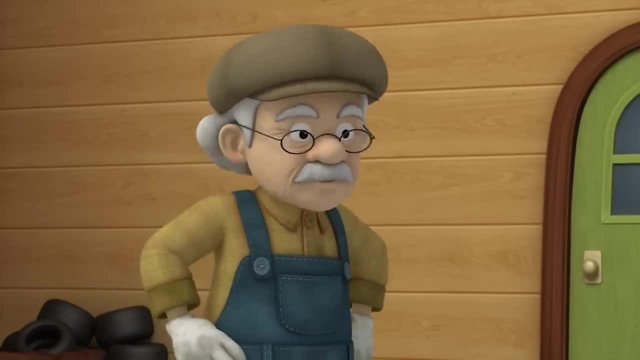 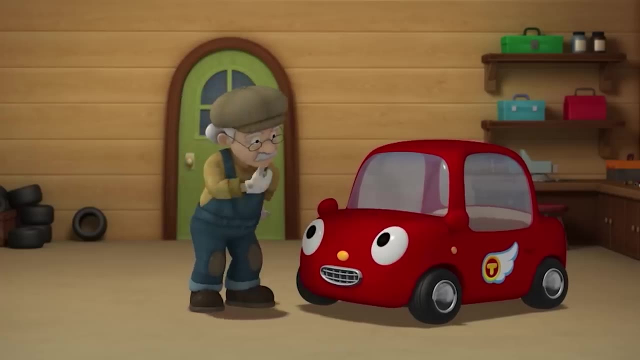 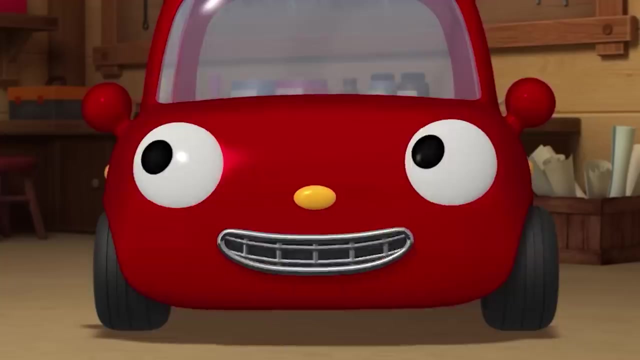 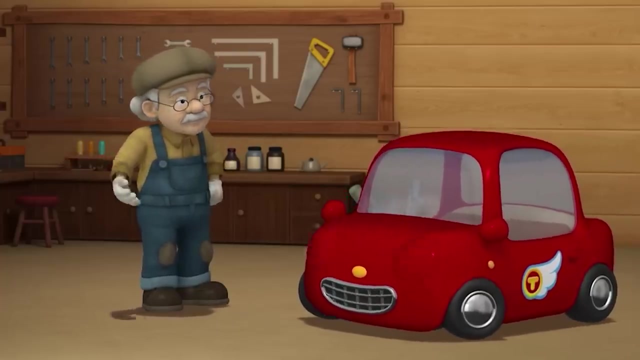 Really You did. Yes, Tutu, That's your name, Tutu. Yes, Let's see how well you move. Come over here, Okay. Oh, very good, Can you circle this place? Sure, Sure, Great job. 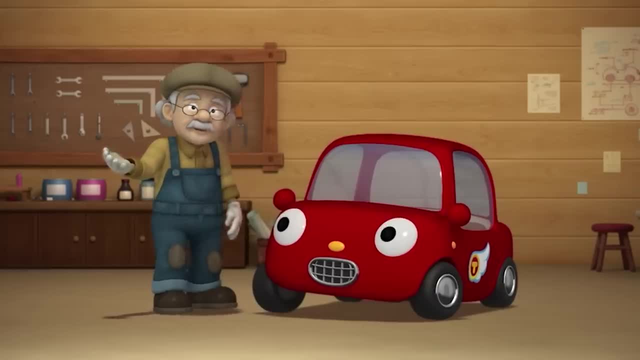 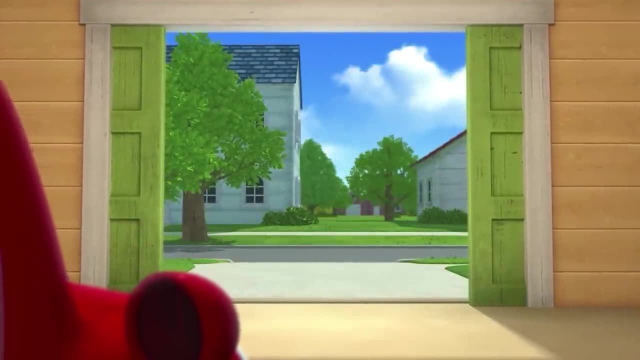 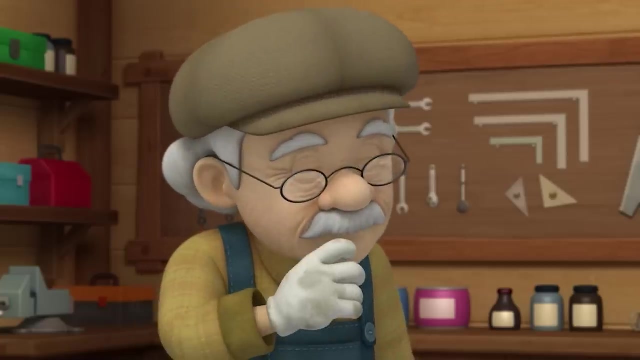 Tutu. that's all for now. Tomorrow we'll go outside, Outside. Yes, I was very anxious to go outside. Wow, Can we go out now? Now, Hmm, You'll have to wait. You have more to learn. 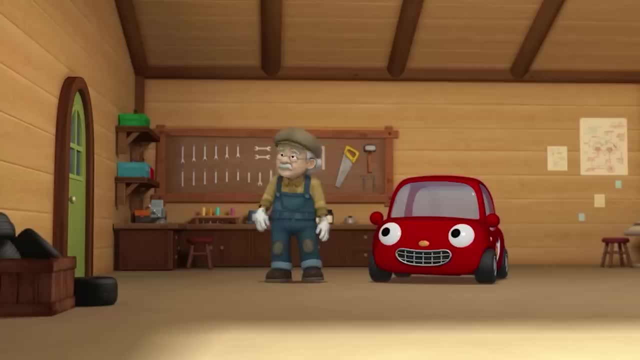 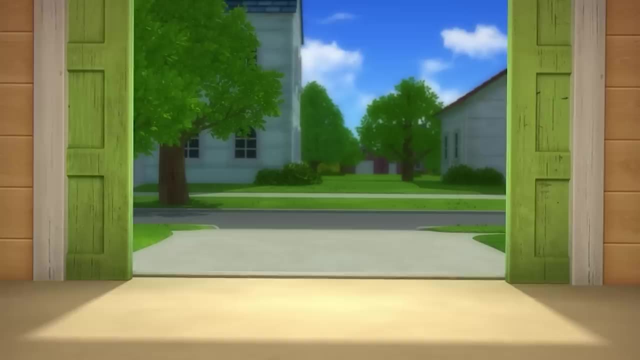 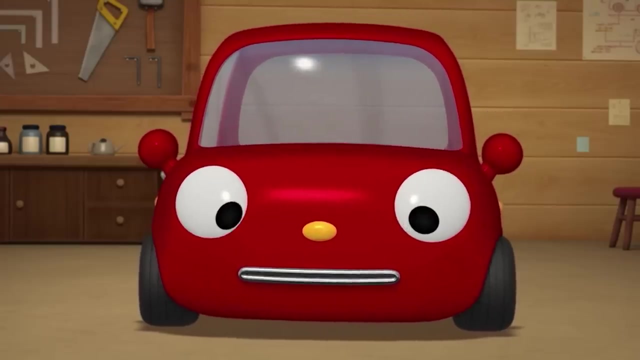 Oh, the phone's ringing, I'll be back. All right, I'll wait for you outside. I'll be right back, Bye, Bye, Bye, Bye, Bye. I can't wait to see Tutu. So what's your name? 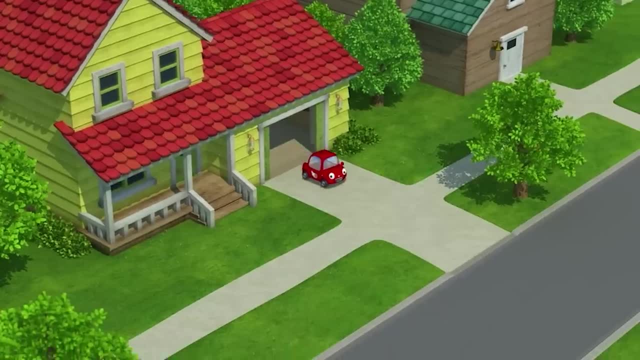 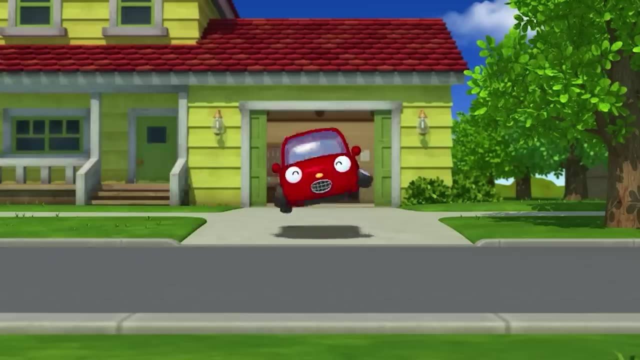 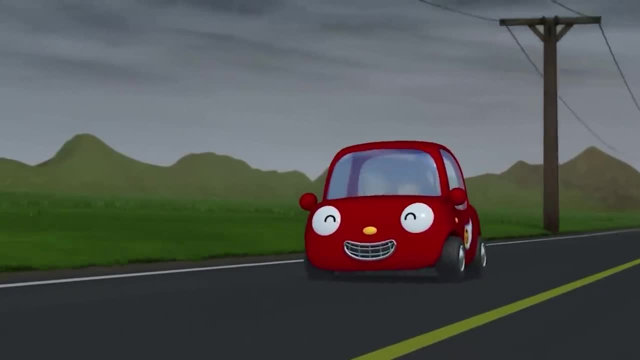 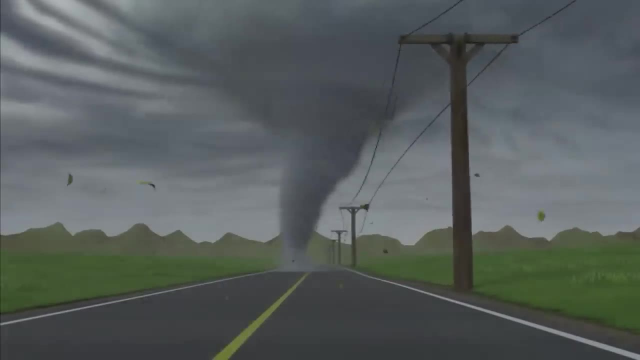 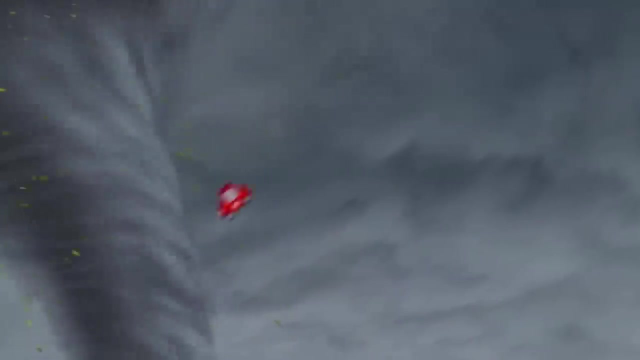 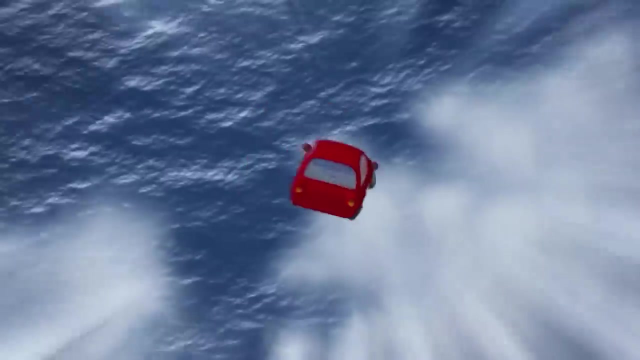 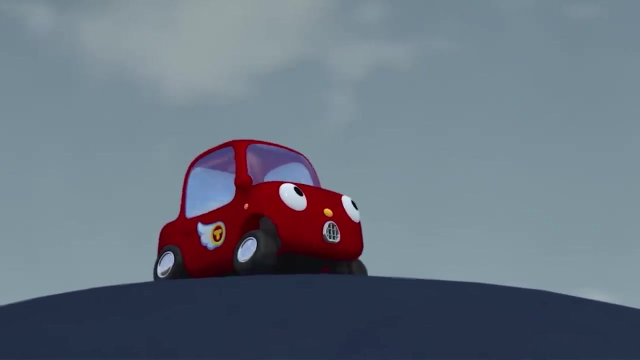 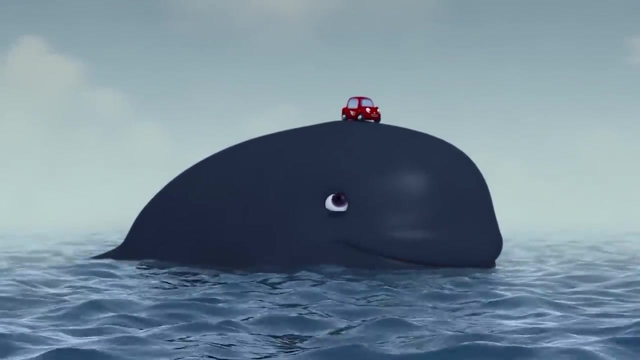 Tutu, Tutu. Should I head back now? A tornado was heading towards Doodoo. What's that? No, Doodoo flew into the sky. I'm flying, Yikes. Where is this My back? Hi little car, I'm Whale. 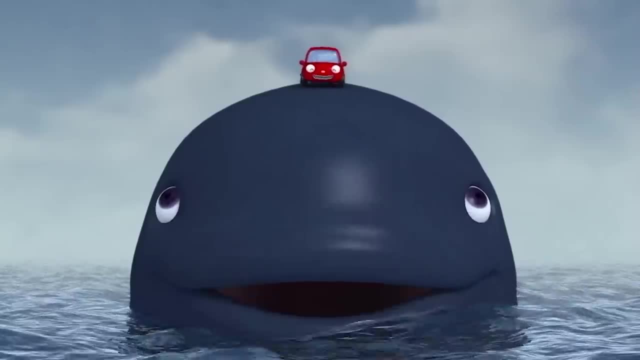 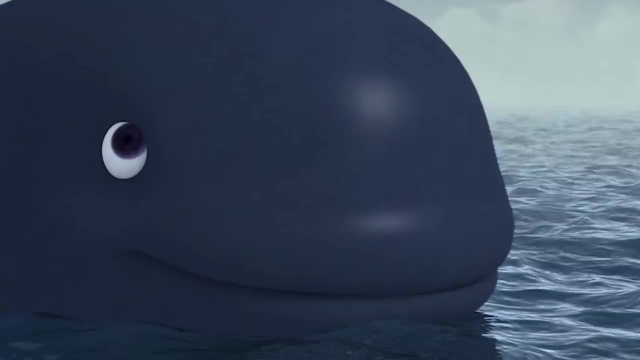 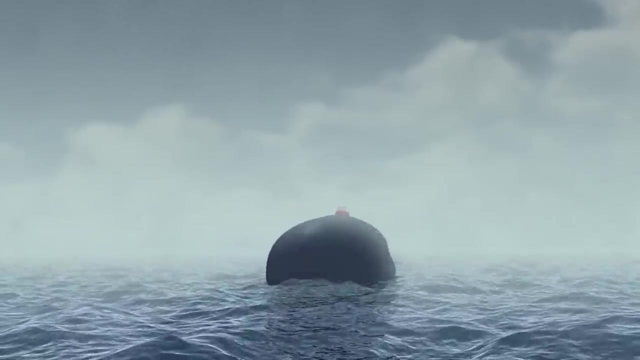 Hi, I'm Doodoo, Doodoo. where's your home? I'm not sure The wind brought me here. Then I'll tell you. I'll take you to a safe place. Whale took Doodoo to the far side of the sea. 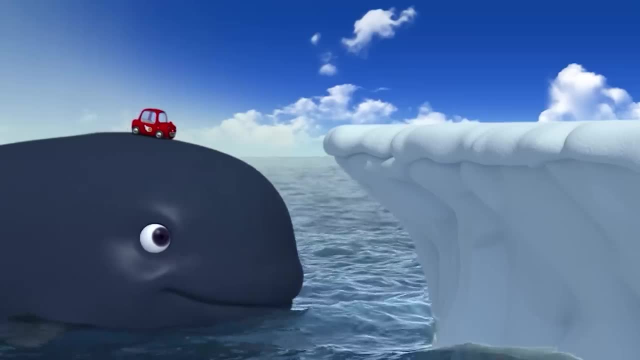 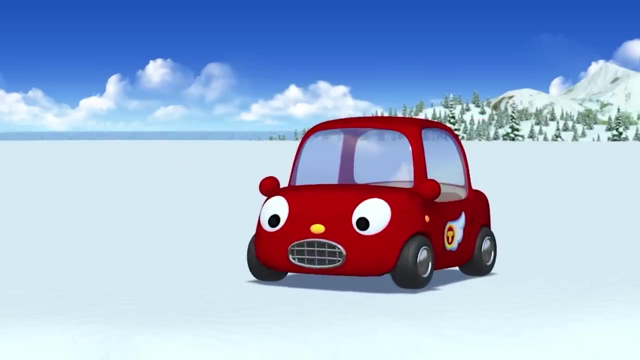 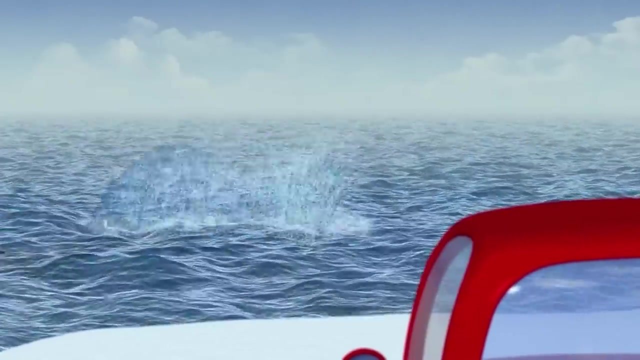 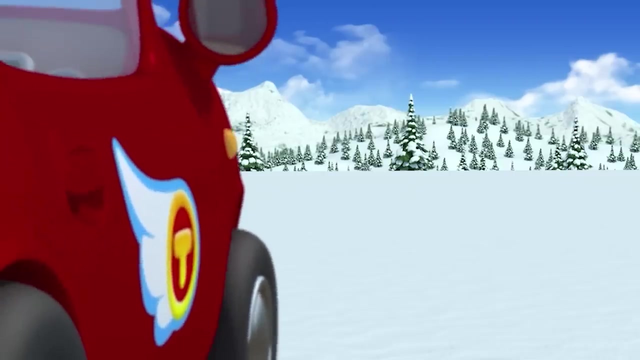 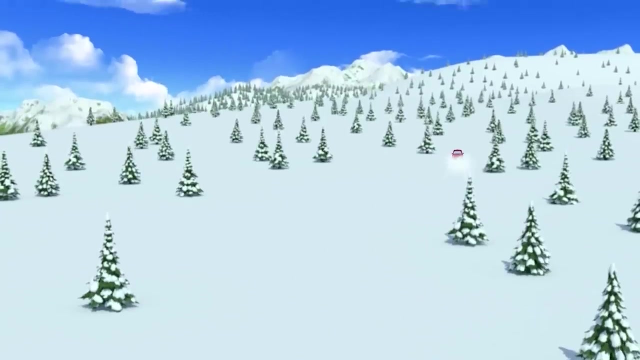 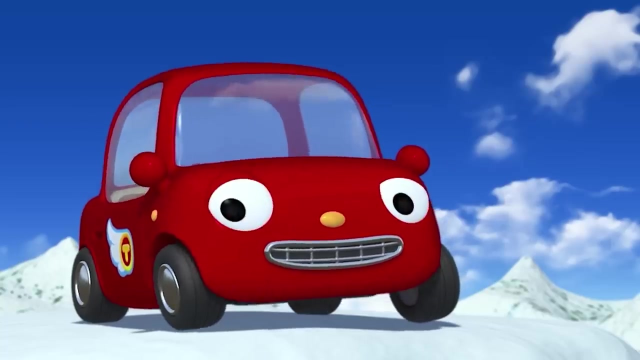 You can get off here. Okay, We're here. Thanks, Whale, You're welcome. I hope you get home safely. Bye, Thanks Bye. Where am I? I'll just explore What's that sound. It's coming from below. 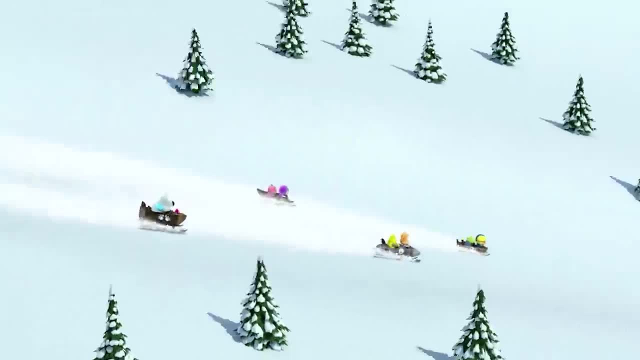 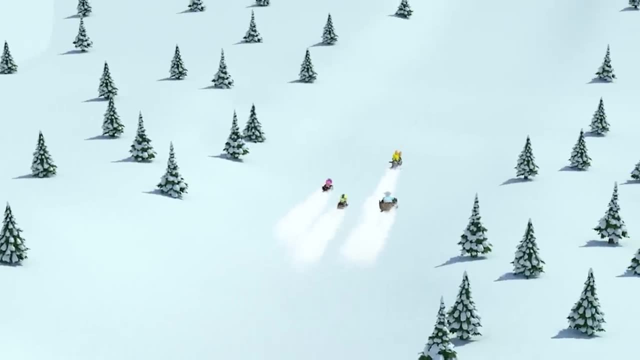 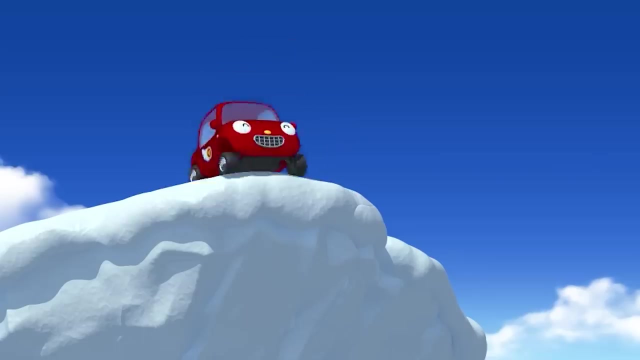 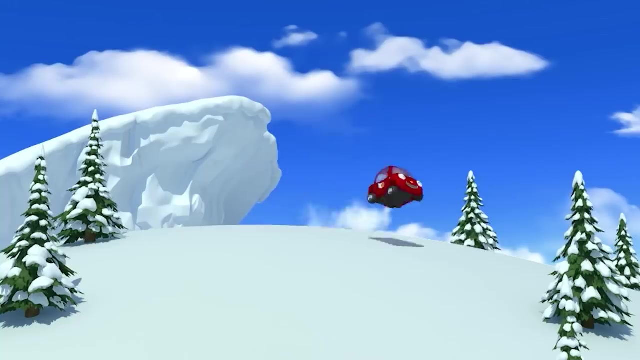 Whee, Ooh, Whoa, What's that? Wow, that's cool. That looks fun. Whoa Yippee. Oh, they're good. I'll try. I don't want Whoa Whoo. 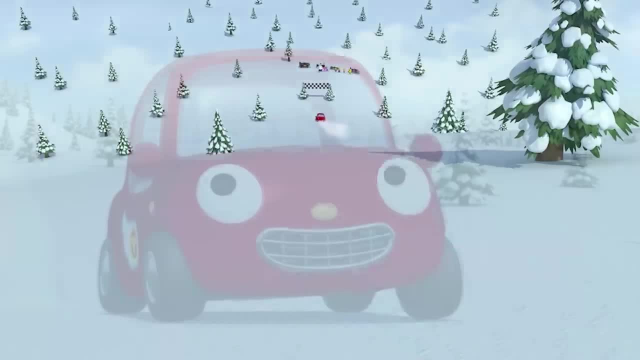 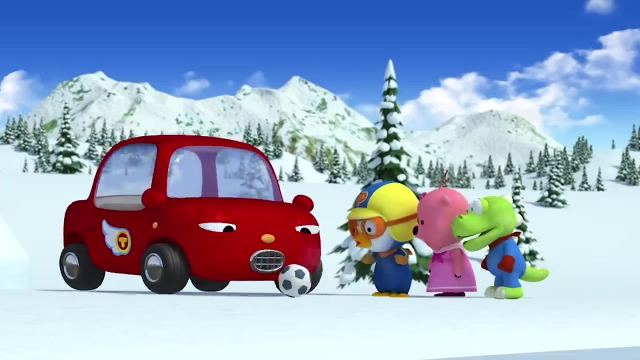 Yippee, Ha-ha, Boo-hoo, Ha-ha, And that's what happened. Oh okay, Oh, Krong, And Oh oh, oh Huh, Can you kick the ball? Let's play together. 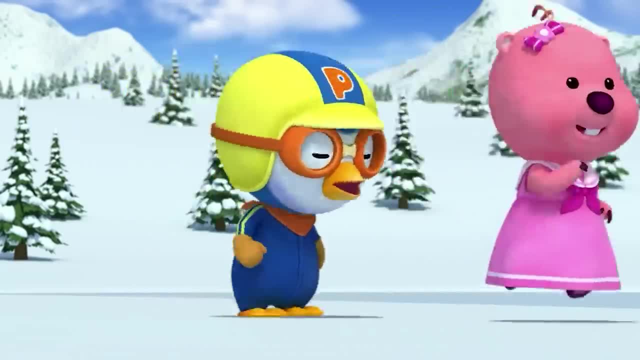 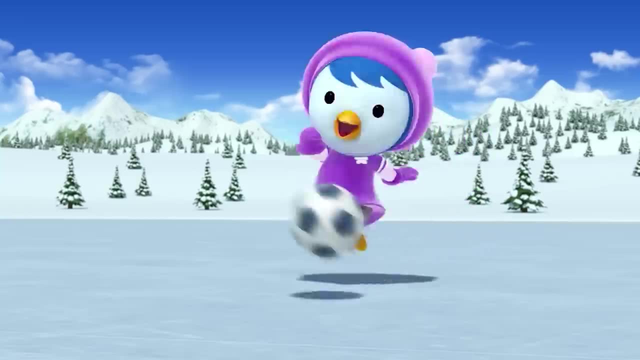 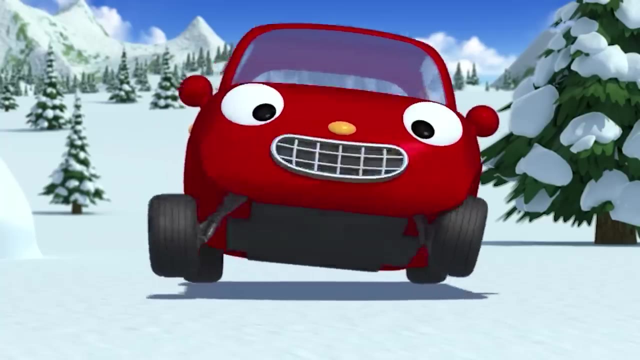 Krong, Krong, let's play together. Oh Doo-Doo, I'll be right back. Okay, All right, Here I got it. Whoa, Oh, wow, how fun. One, two, one, two, one, two. 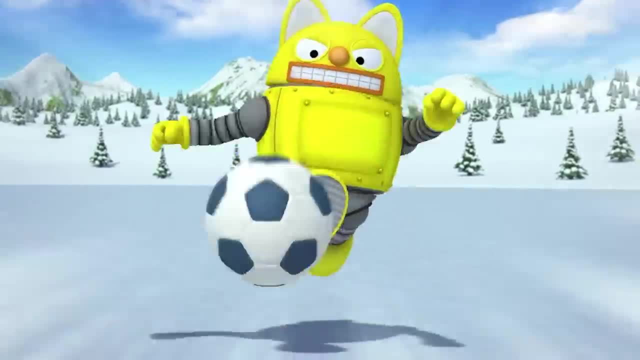 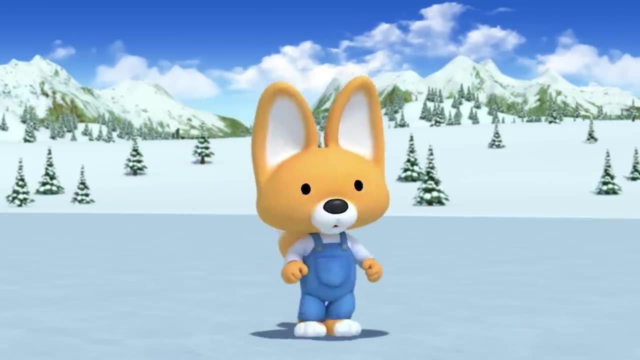 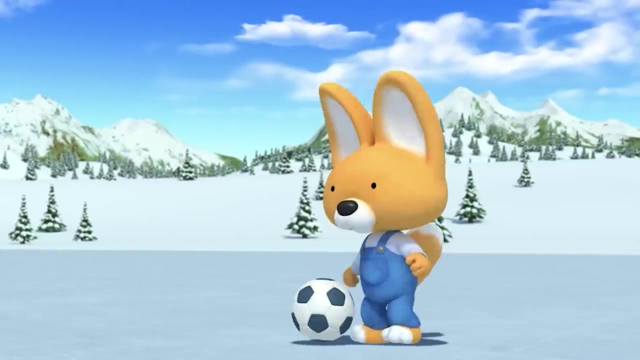 Roadie, kick the ball. Okay and shoot. Oh caught it. Oh too bad. Yeah, Great, Huh, Huh, Huh, Uh, Yeah, Oh, oh, that was great. Thanks, I'll play. 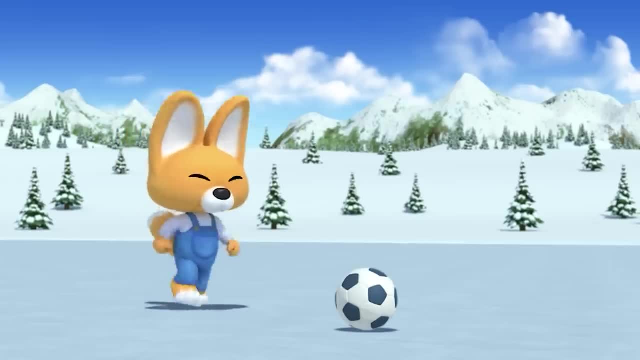 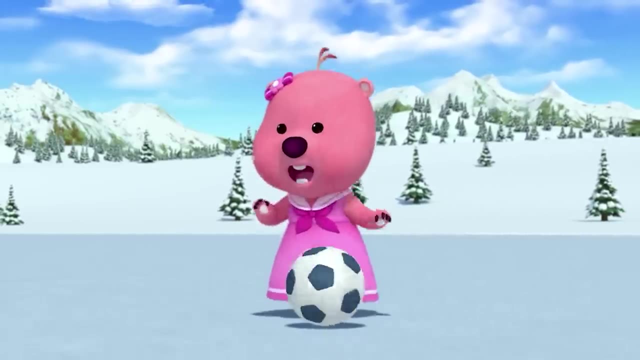 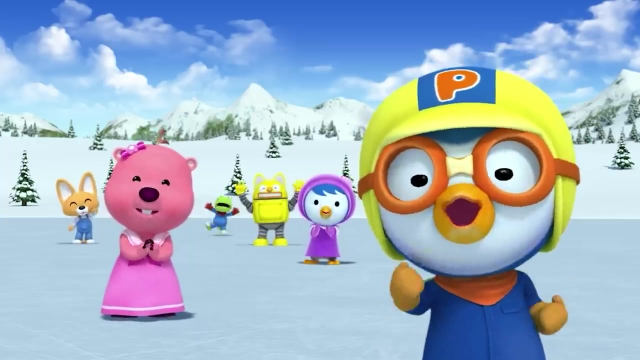 That car even plays ball. Uh, here Cha Get it Lupe. Uh uh uh. all right, Doo-Doo, I got it Goal. Ugh Whoa, Oh, you're a pro at playing. 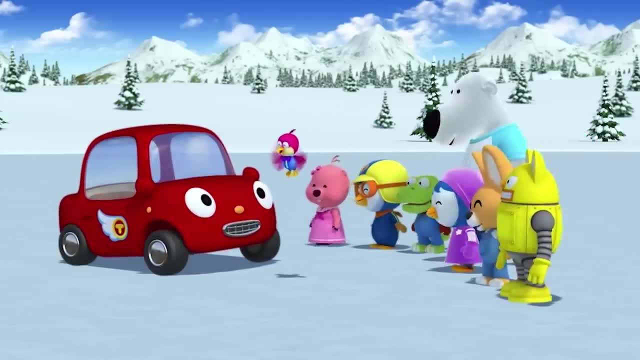 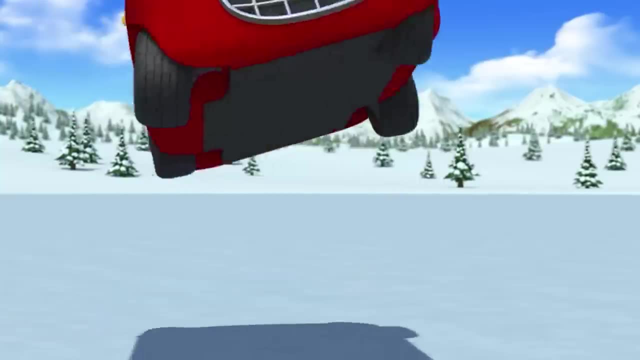 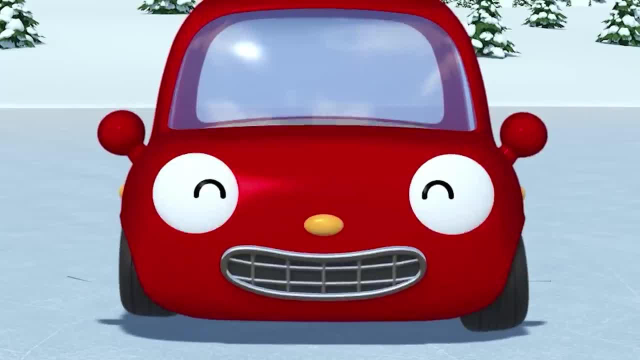 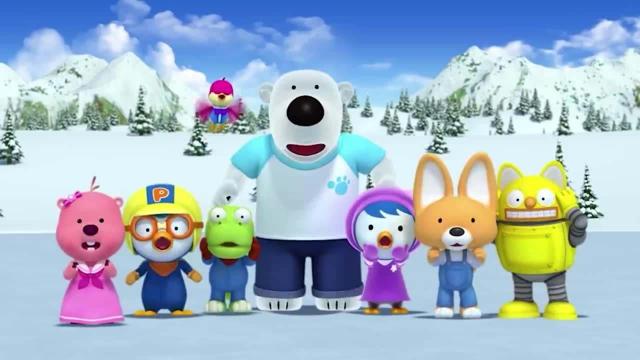 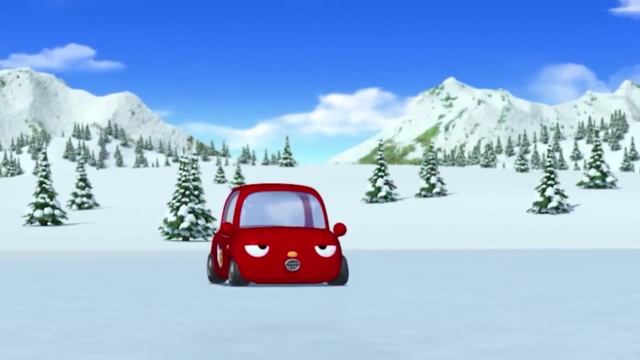 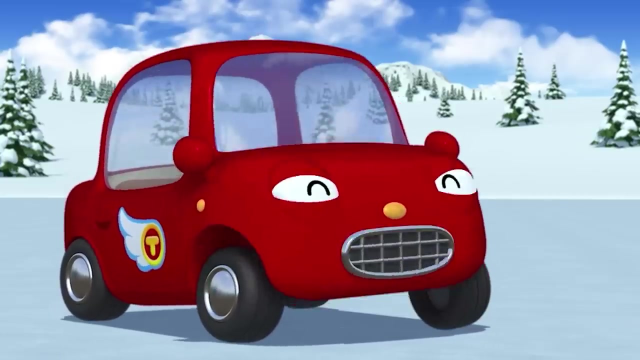 whoa, whoa, whoa, whoa, whoa, whoa, Ah Doo-hoo. How'd you do that I have the ability to swim underwater. We were worried. What a relief. Huh, Huh. 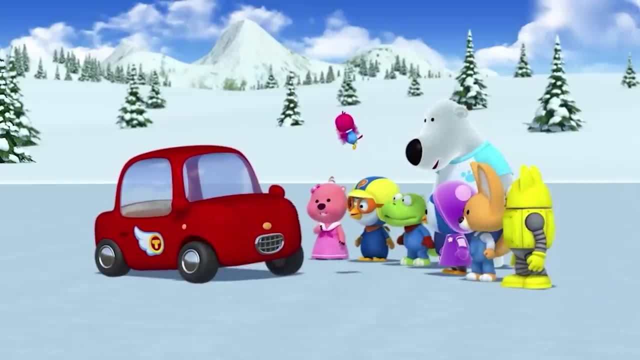 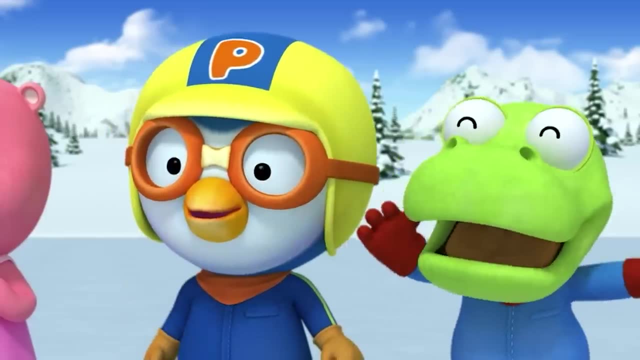 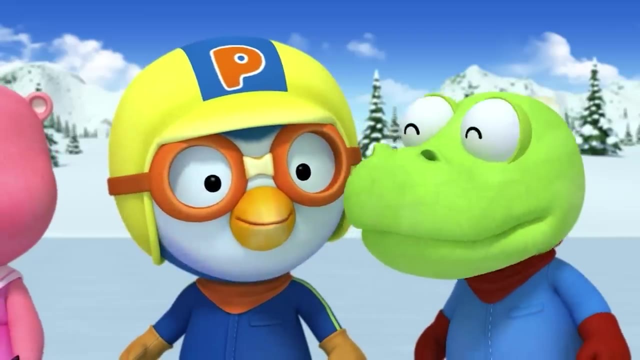 Huh, I made sandwiches. Let's go to my house. You're the best Luffy Tutu. where are you going? Uh, I don't have a place to go. Then do you want to come with us? 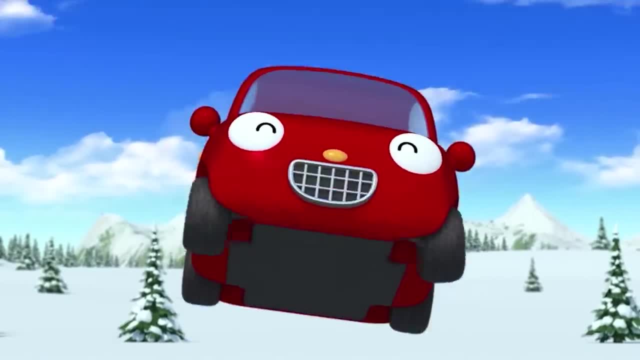 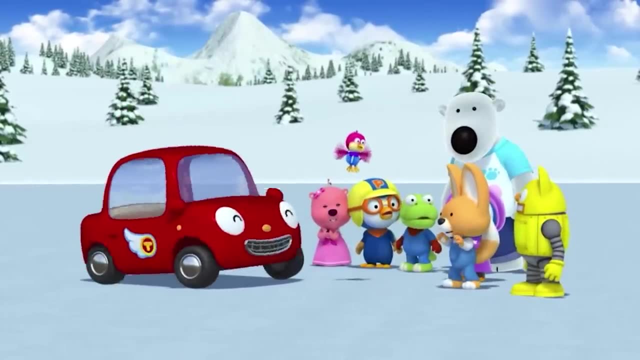 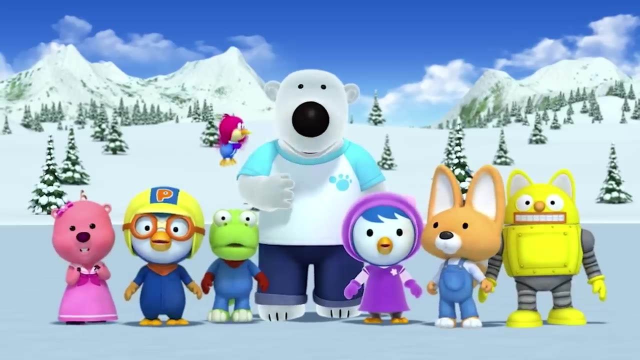 Really Thanks, Yay, Wow, thanks so much. Calm down, These guys might break again. Huh, I'll give you guys a ride. All of us. How can you get all of us? Really Okay, here we go. 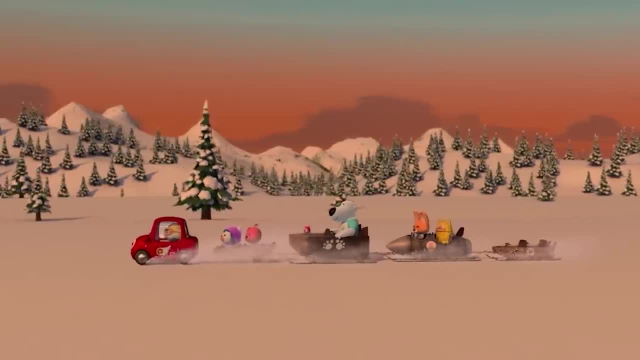 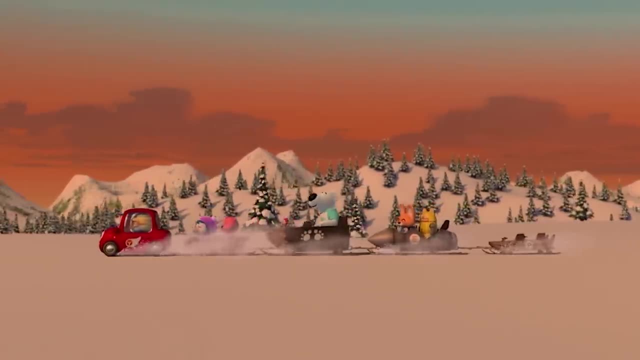 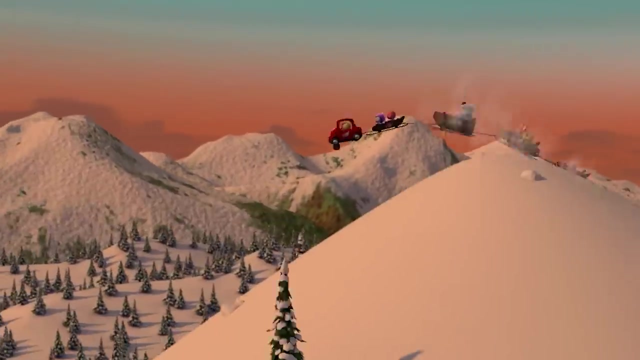 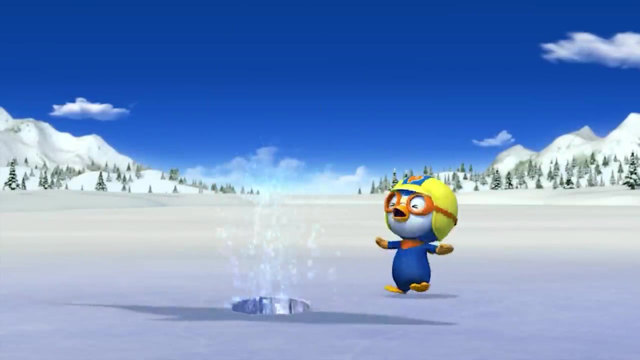 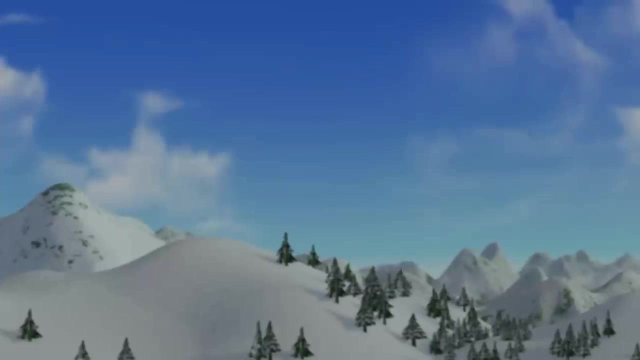 Yay, You can ride any time from now on. There's a new friend in Borong Borong Village. What other adventures Will happen next? Clumsy Magician Pororo and Krong are headed to Tongtong's house in their plane. 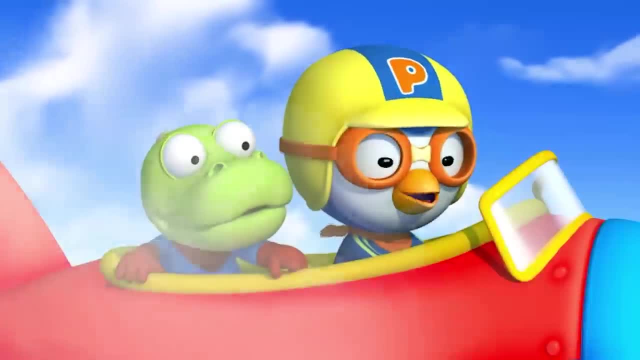 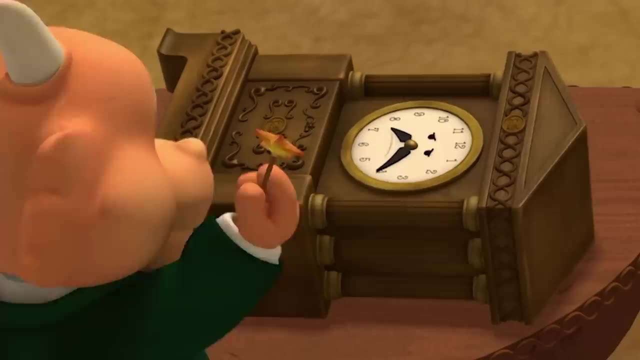 I was sure it was somewhere around here. Krong, Krong, There it is Kuri, Kuri, Tongtong, There's Tongtong over there, Chongtong, are you sure you can do it? That's what I told you. 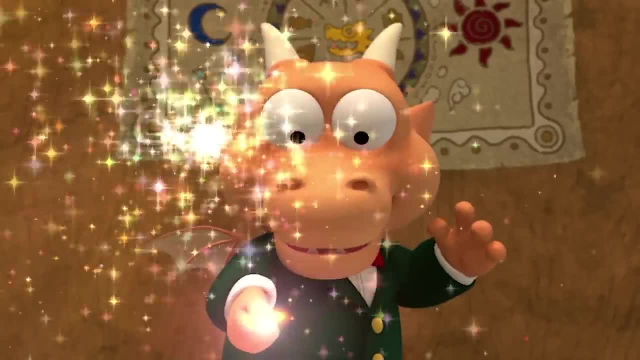 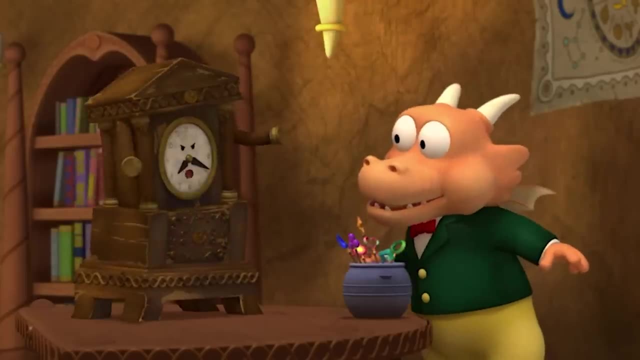 I'll make you into a brand new clock. Now charge. Let's see. huh, Oh, what's this? Huh, What's going on? I've become an antique. Huh, That's strange. Guess it wasn't this one. 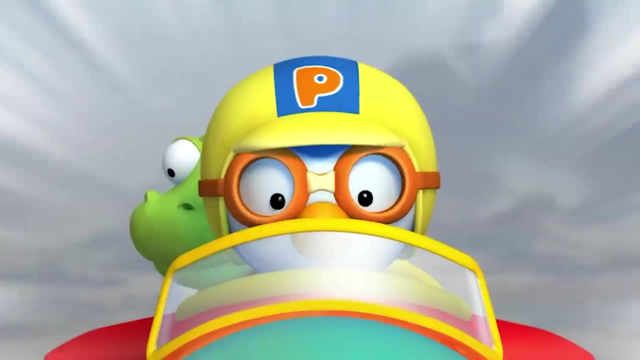 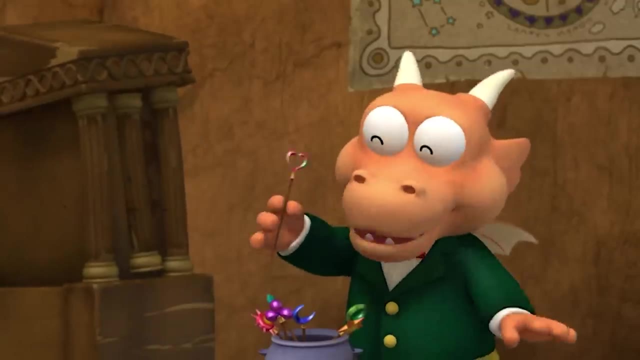 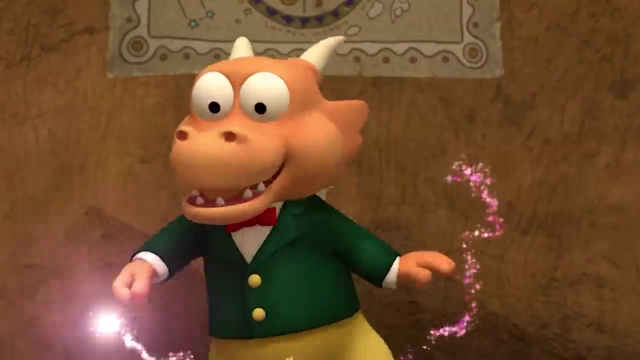 Maybe another. Now, let's go down. Now, let's go down. Oh, I think it's this, Are you sure? Of course, I am Kuri Kuri Tongtong, Kuri Kuri Tongtong, So. 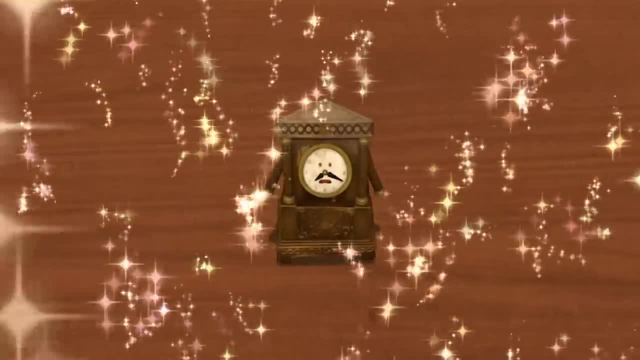 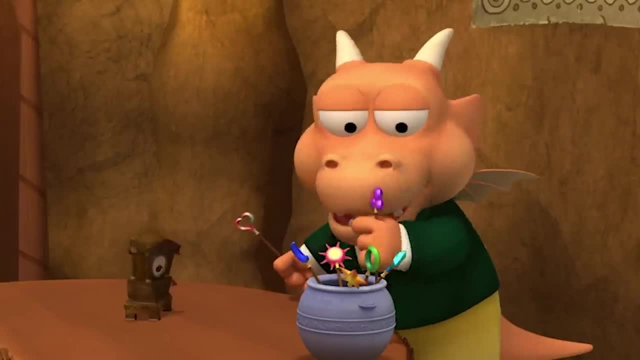 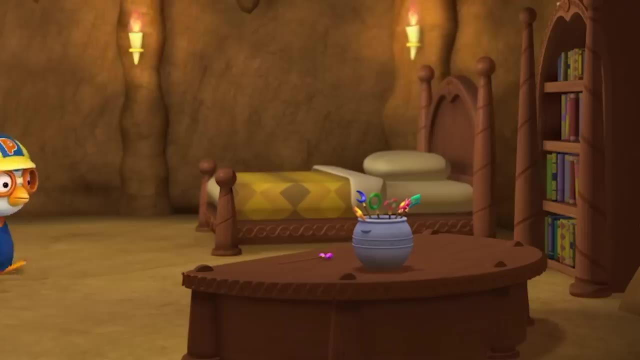 Then is it this? No, no, Tongtong, Huh Hi, It's us. Krong Krong, Krong Krong. Wow, What's this? Wow, There's so many interesting things. Krong Krong. 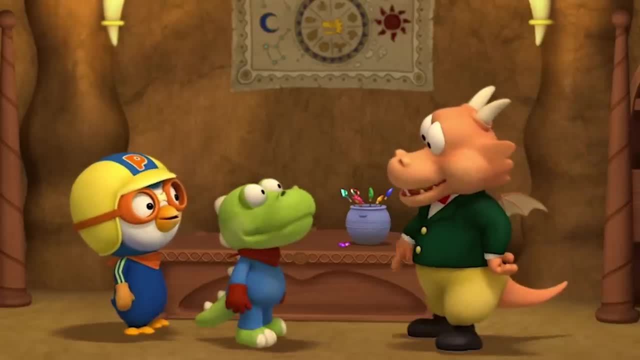 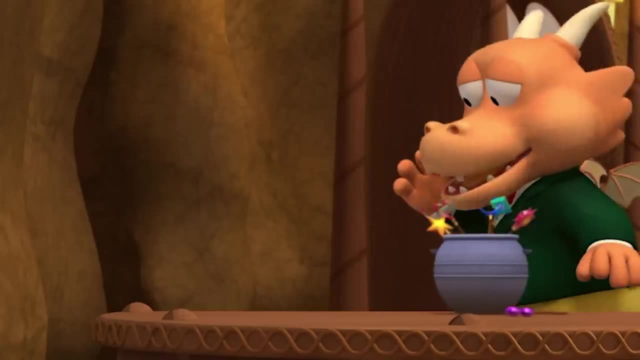 Huh, Ah, That's a magic wand. I was in the middle of fixing the clock. Huh, Oh, He's gone. Clock, Clock, Come out. I'll be right this time. Hmph, I can't trust you. 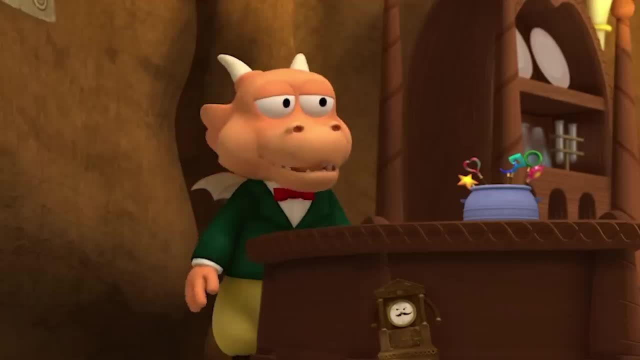 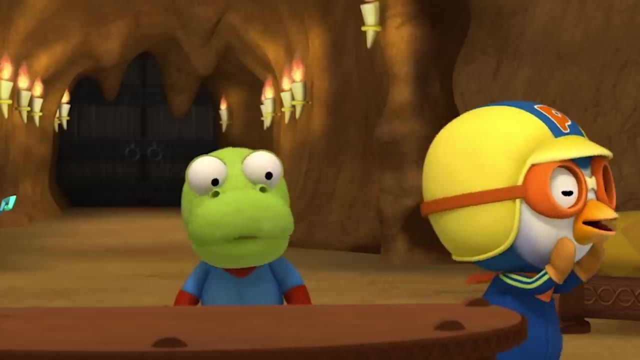 Tongtong. What are you doing, Krong? Oh, I'm looking for the clock. Uh, Clock, Oops, We'll help you find it, Clock, Oh, I'm so coral In ja dum Here. Well done all of you. 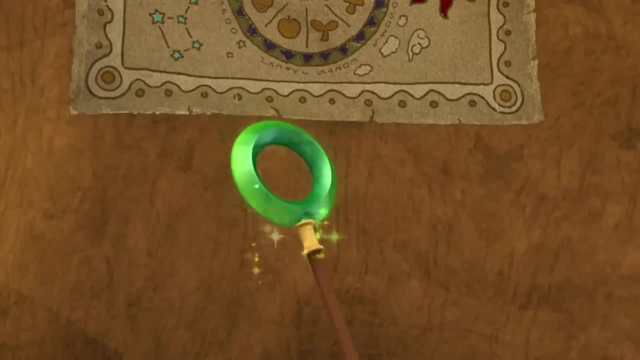 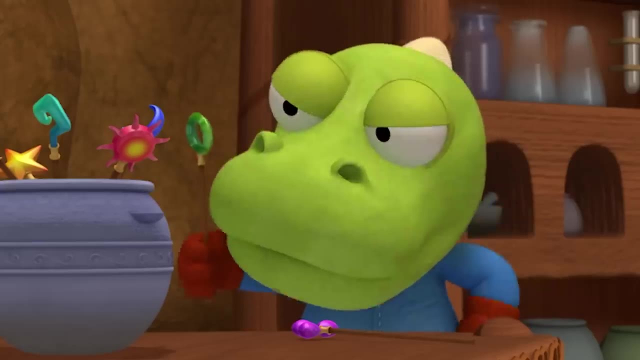 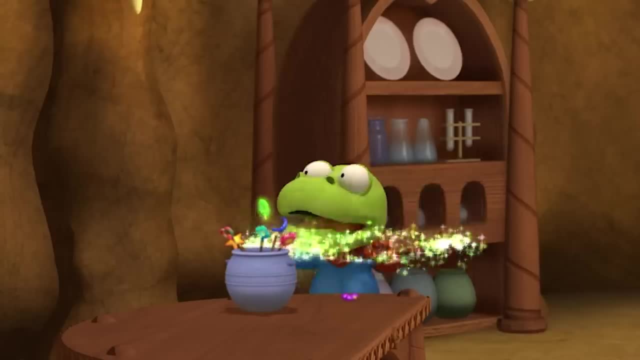 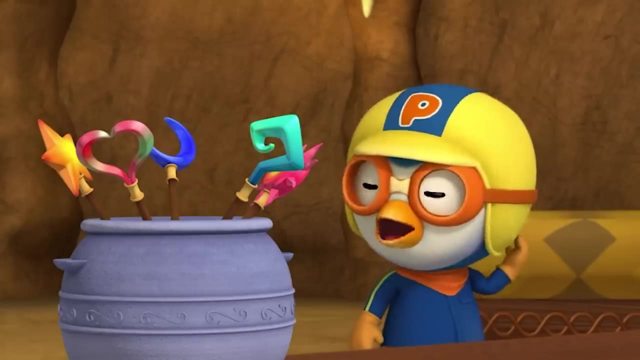 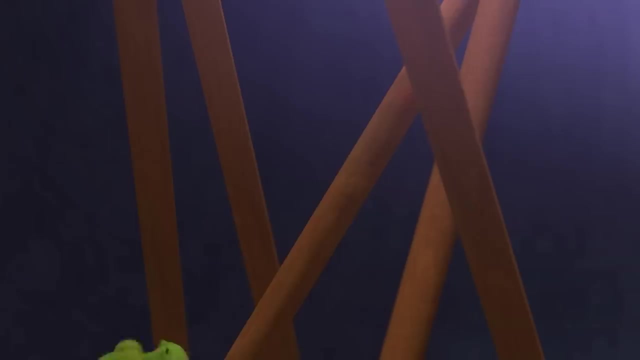 Krong Hup, Hup. Oh no, Krong is touching the magic wand. He shrunk and fell into a jar. Mmm, I thought I saw something flash. Hmm, Krong, Krong, Krong, Krong. 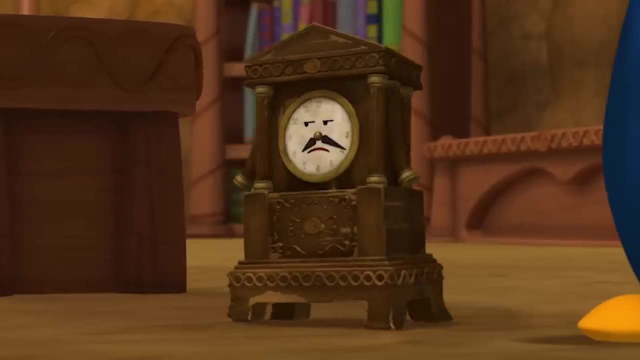 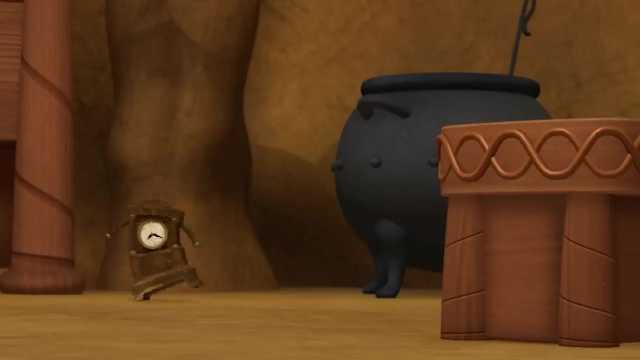 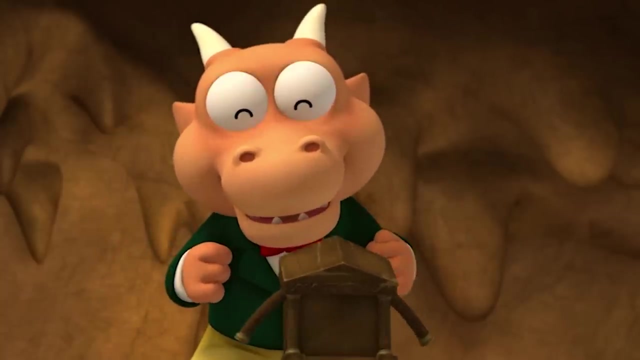 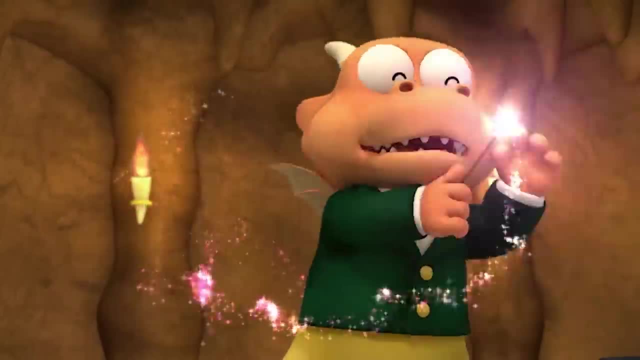 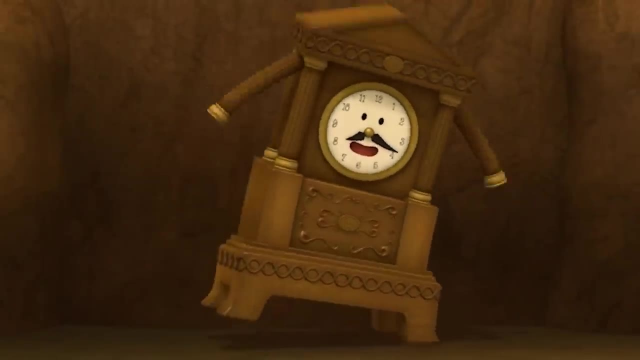 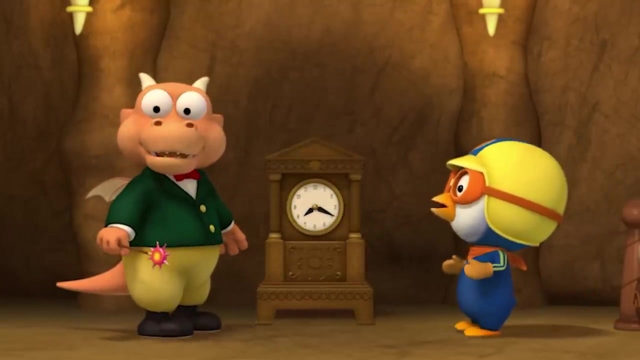 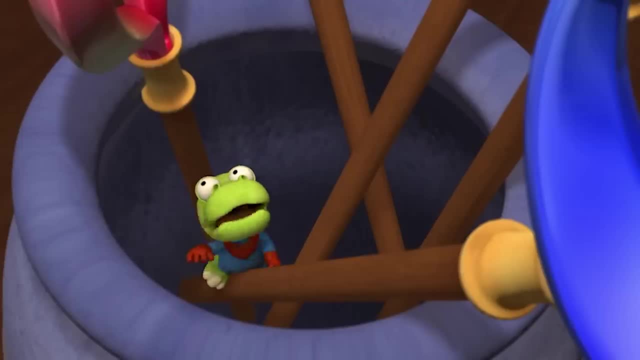 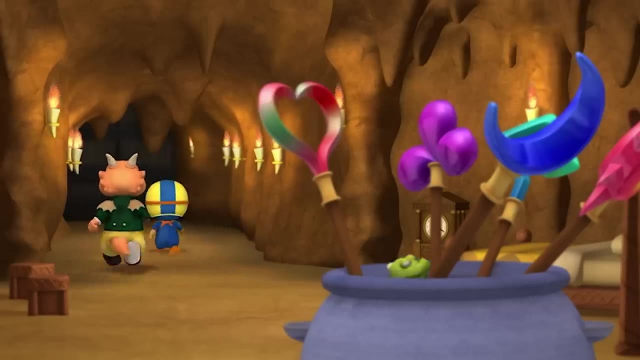 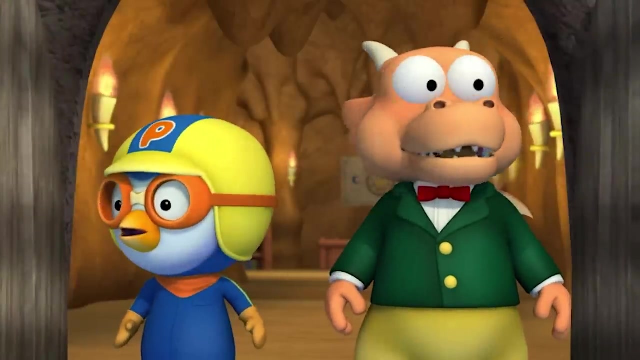 Krong Krong, Krong, Krong. Where is he? Maybe he's out, Let's go out. Oh okay, Krong Krong, Oyo-yo Krong Krong. Potoro and Tongtong went outside to look for Krong. 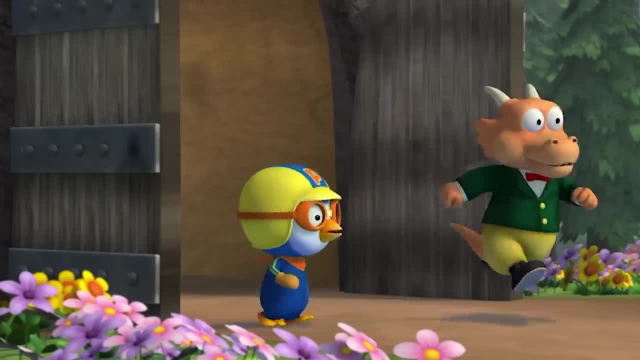 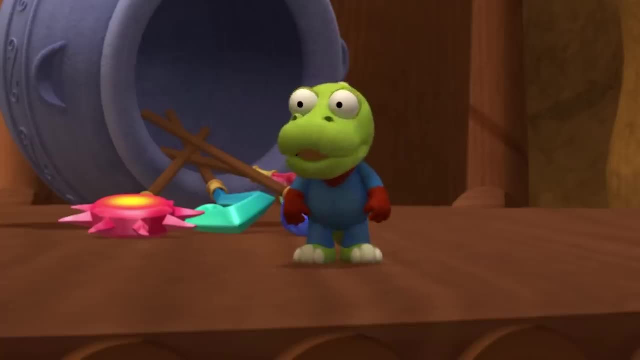 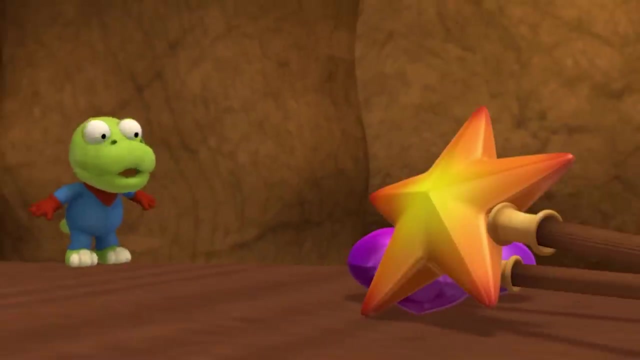 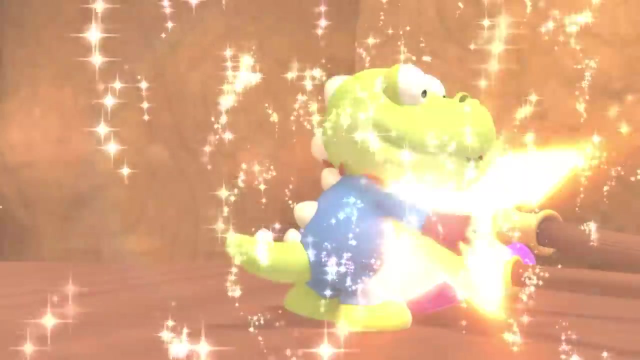 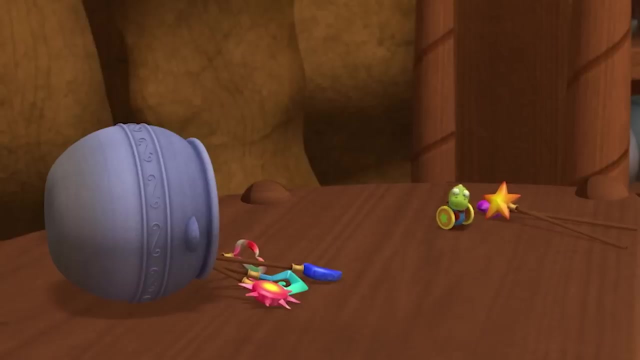 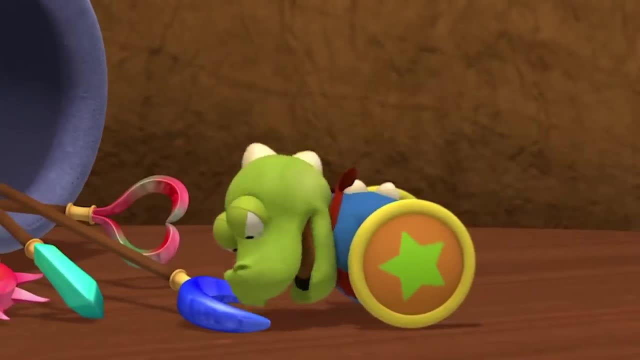 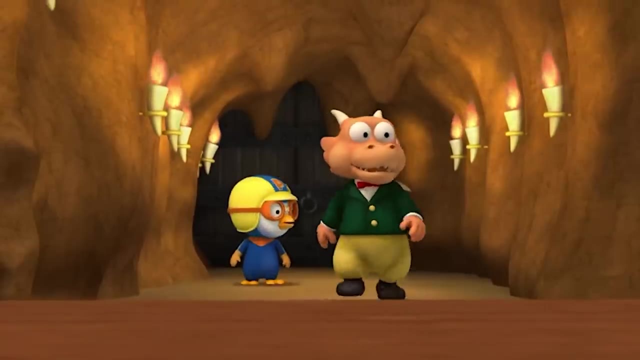 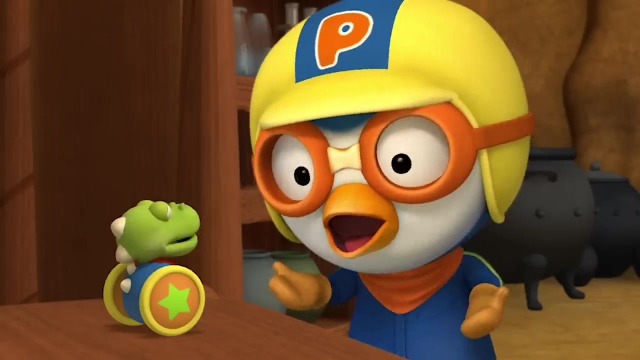 Krong Krong, Krong Krong couldn't reach the magic wand. Krong Krong, where were you? Krong Poyoyo, Huh, Poyoyo Krong. What happened? Krong, Krong, Krong. 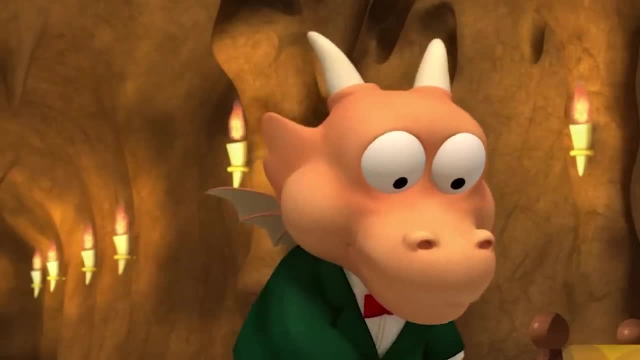 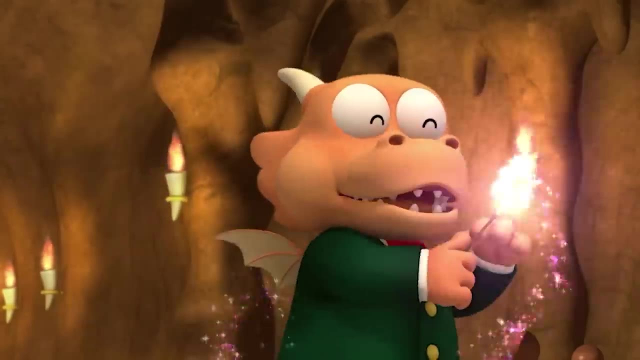 Oh I know Krong is under magic. Let me help. Can you turn him back to how he was, Of course? Kuri kuri tong tong. Kuri kuri tong tong, Change Krong. 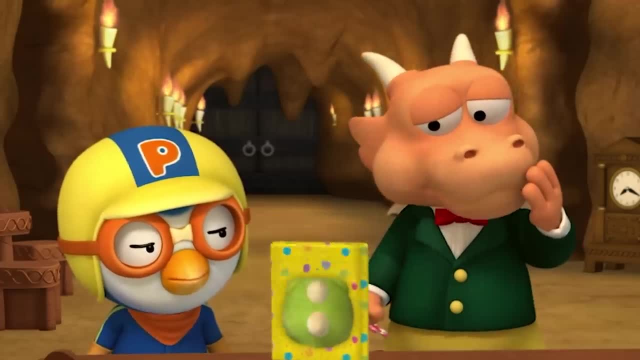 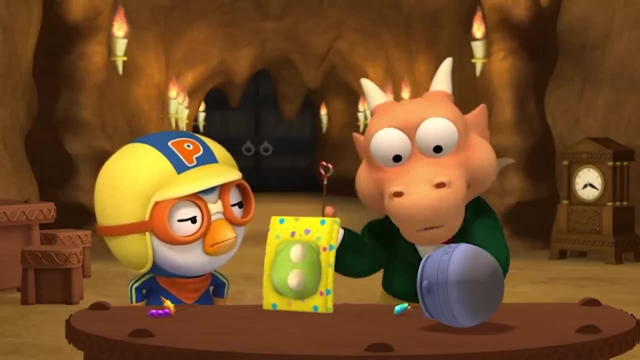 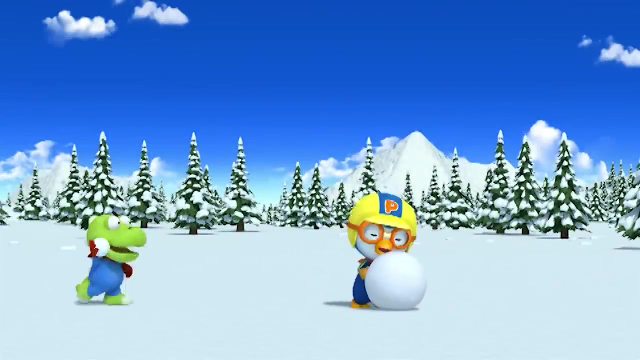 Krong, Krong, Krong. Oops, you turned into a book. You said you could do it. It wasn't this one. Will Tong-Tong be able to change Krong back A day in Porong Porong Forest? 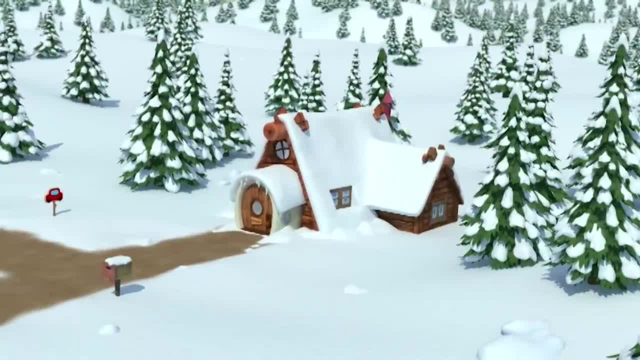 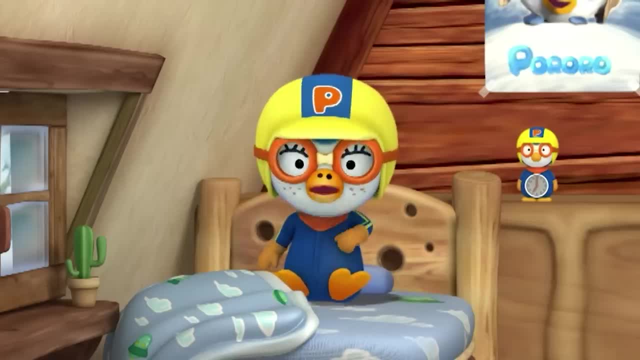 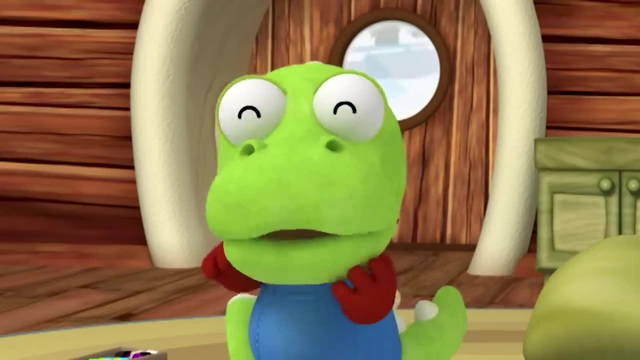 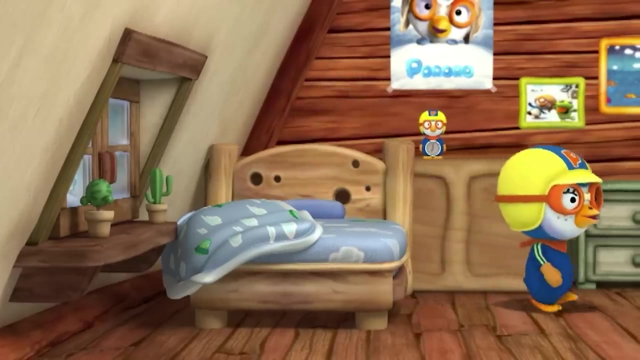 It's a fine morning in Porong Porong Forest. Oh yeah, Oh yeah. Huh, Krong, you're up early. Huh, What's with him? Better go wash my face, Krong. What is this? 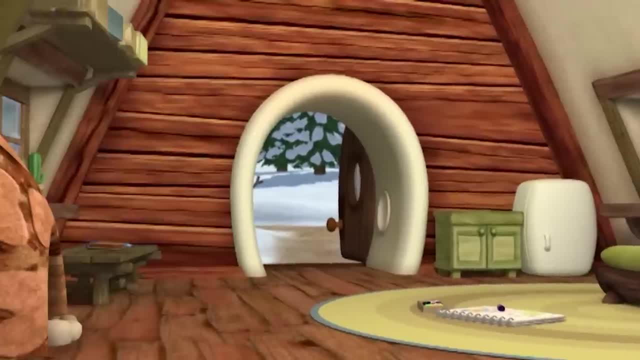 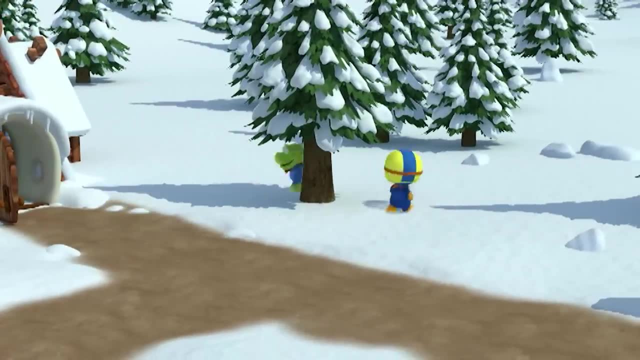 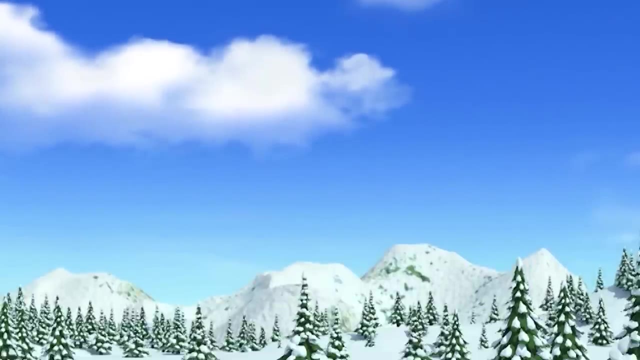 Krong? where are you Come out here, Krong? Huh, What Did I get a hold of? you Get over here. It looks like Krong's prank has caused quite a commotion this morning. There's Loopy and Petty. 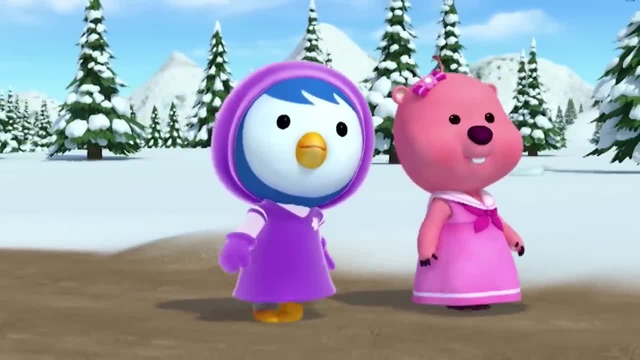 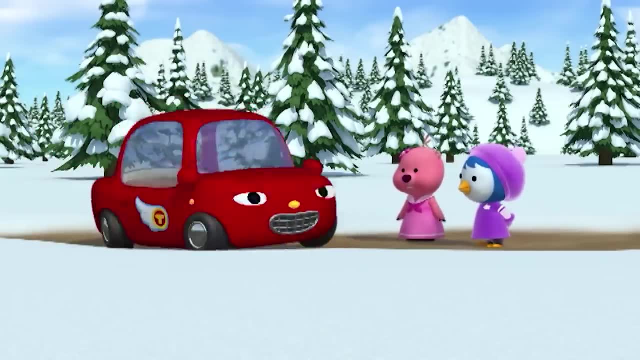 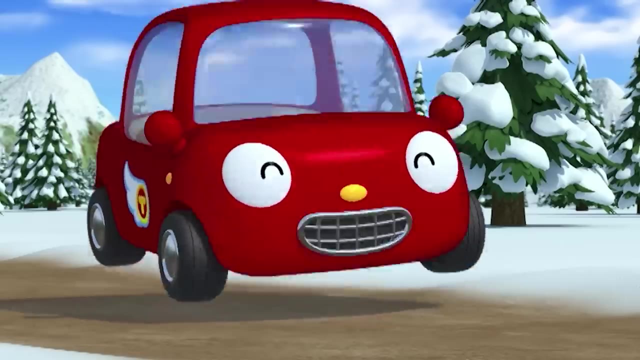 Ah, the weather is great today. I know Huh T. We're driving around the village early in the morning. Where are you off to? We're going to Pororo's Mm-hmm. Let me give you a lift. 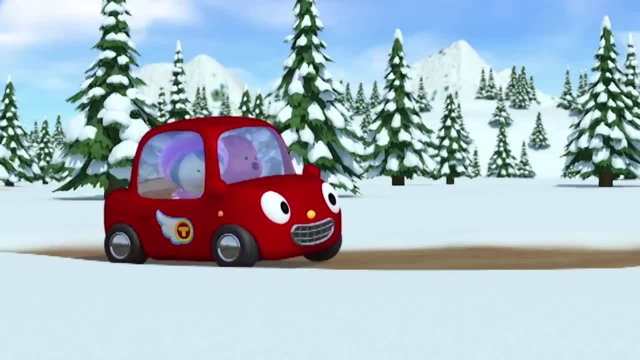 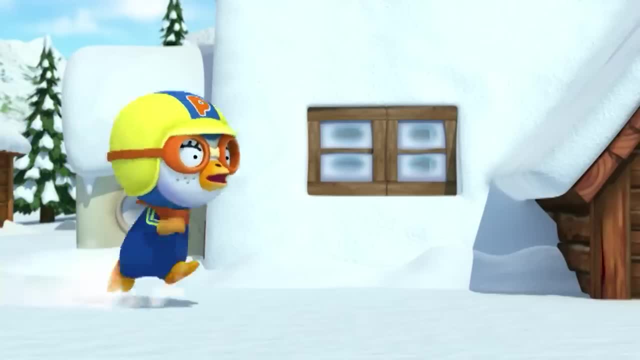 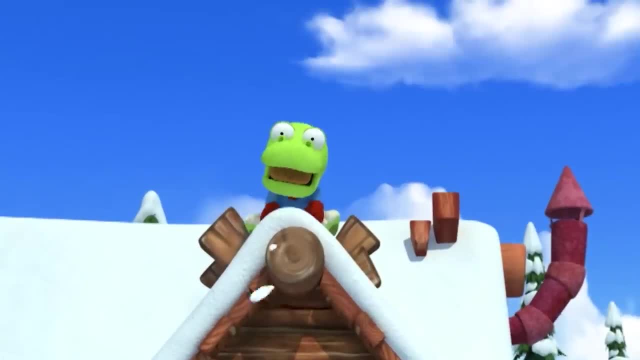 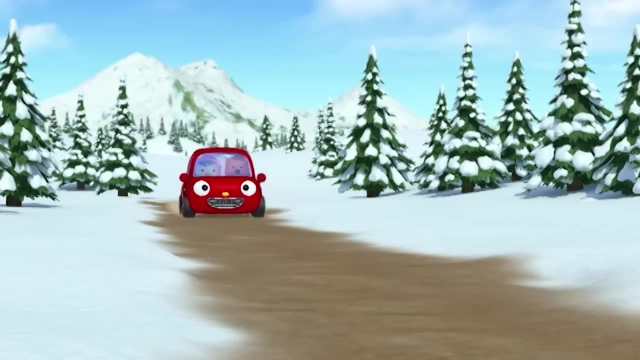 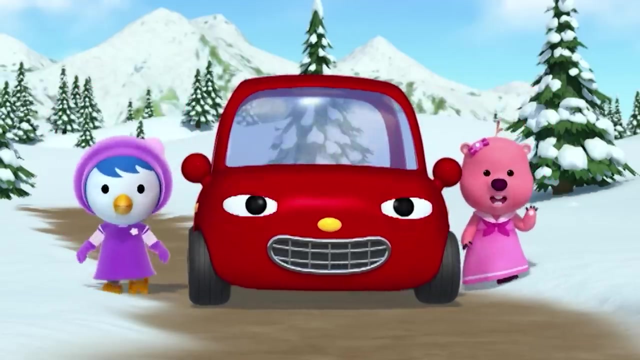 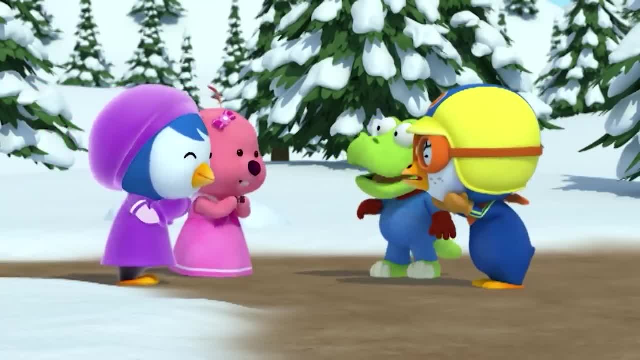 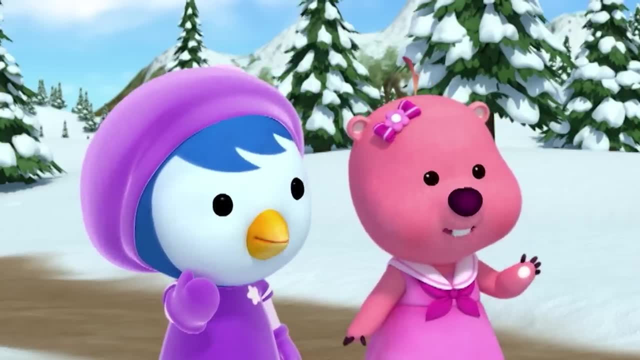 Kro. What happened to your face? Another one of Krong's friends. Ugh Kro, Kro, Kro Kro, Do you want to go to Eddie's with us? Eddie has something fun to show us. Simple, Okay, Kro. 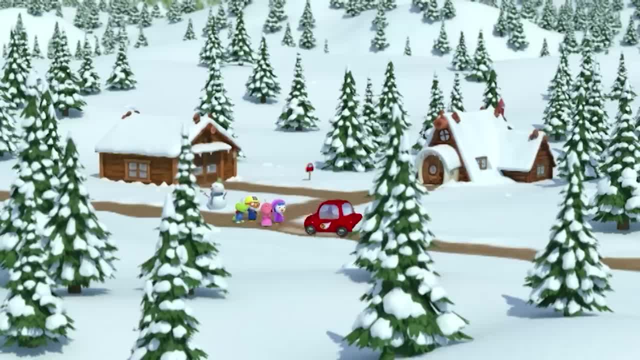 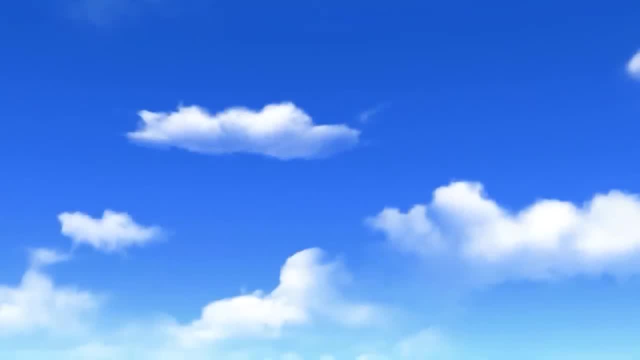 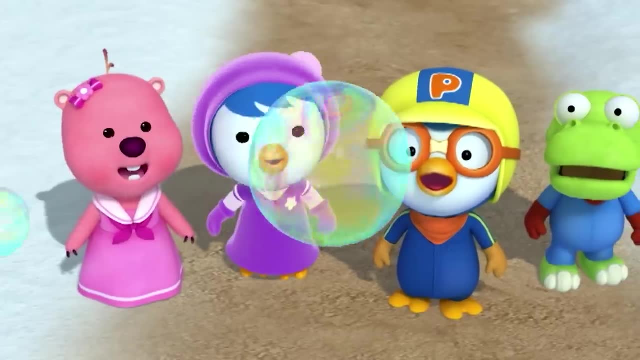 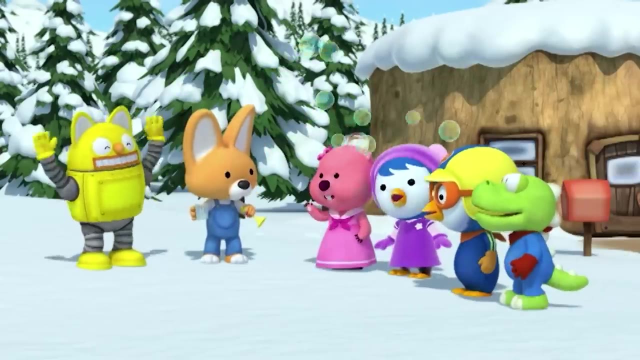 Kro, I'll come over after my drive. Bye, Juju, Bye, Bye. Cool huh. What's that? Wow, they're soap bubbles. They're so pretty Over there. Hey, Johnny, Hey, you all came. 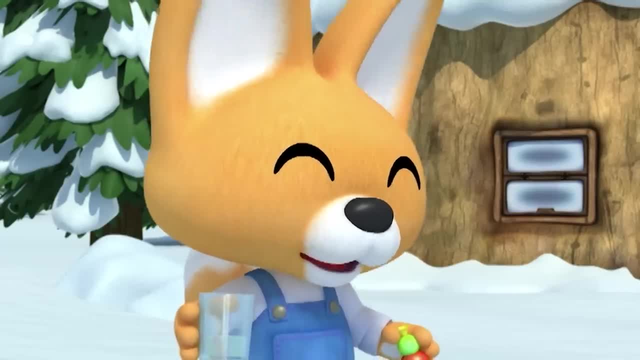 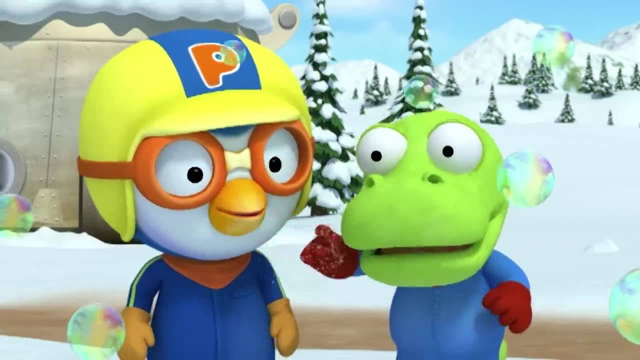 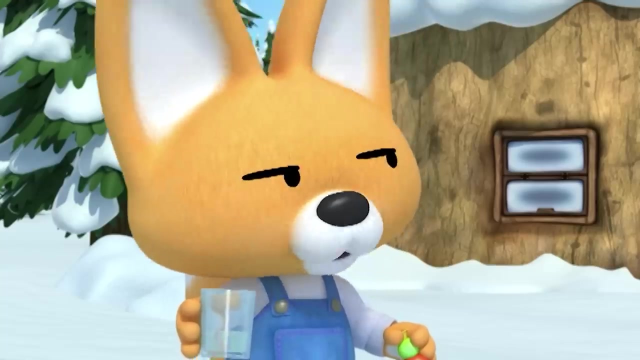 Were you making the bubbles? Yeah, here, watch. Wow, Eddie has made another fun gadget. Eddie, can you make bigger bubbles that don't burst? Bigger bubbles that don't burst? That shouldn't be a problem, Just hold on. 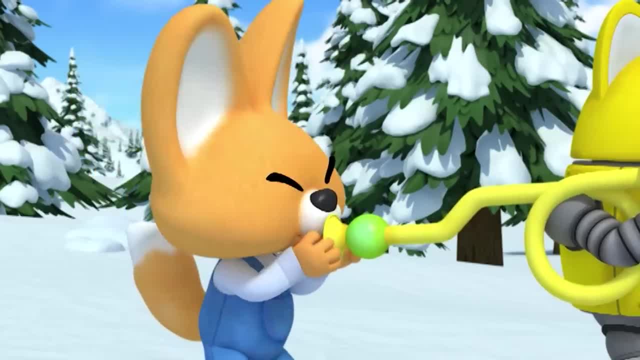 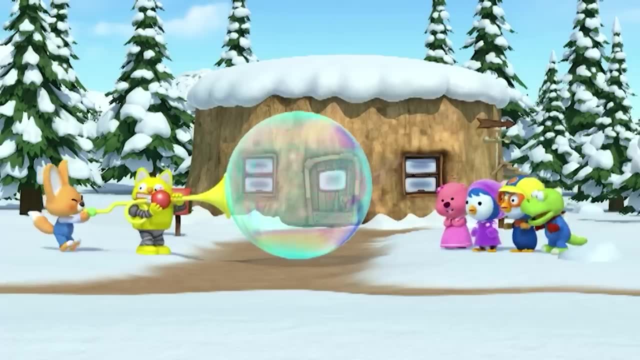 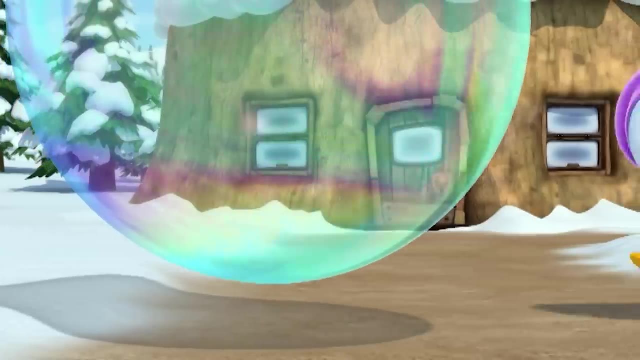 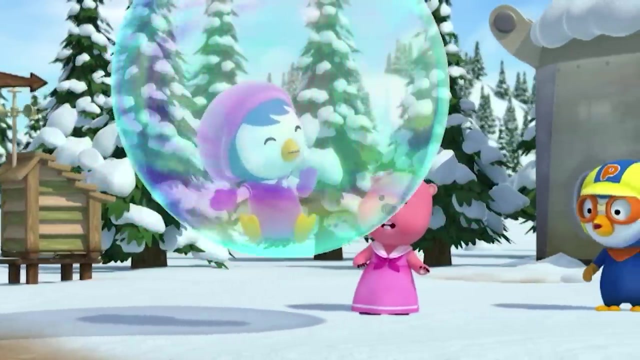 Okay, here I go. Hey, you can do it Just a little more. Wow, you did it, Eddie. Whoa. oh boy, A piece of cake. Wow, so pretty. Patty Guys, look at me, I'm inside the soap bubble. 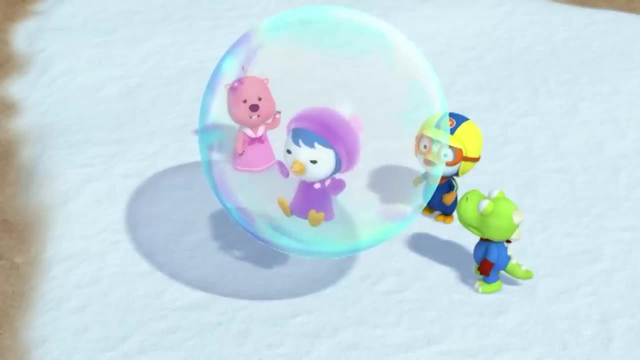 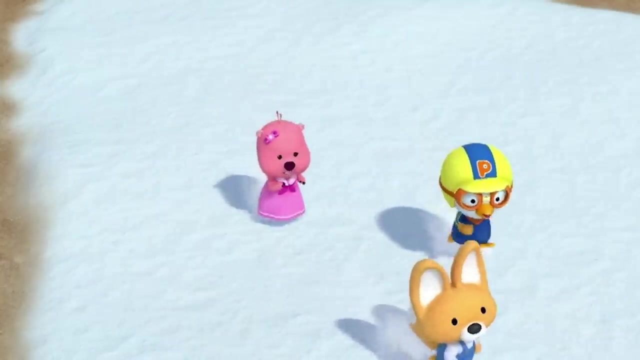 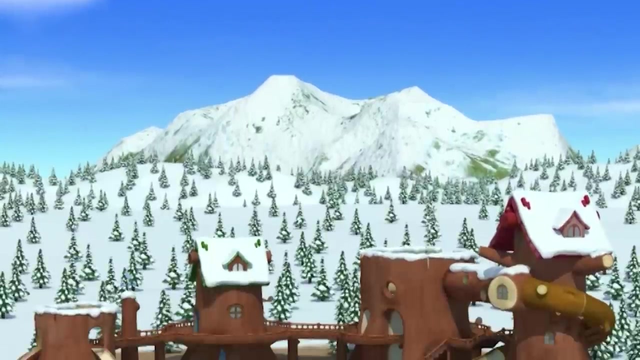 It's dangerous. Come out, Come out, Patty. no, Come down, Come out, Let's go after her. The bubble is taking Patty higher and higher into the sky Over there. Brody, stretch your arms and grab her. 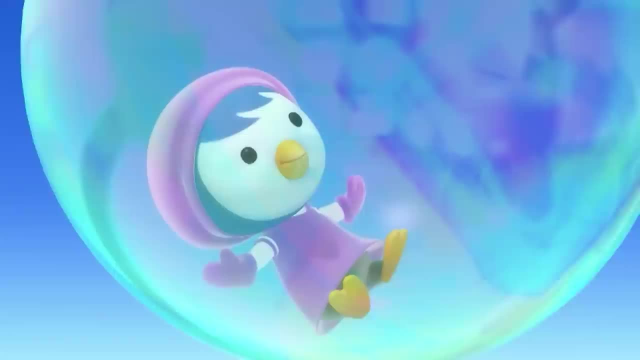 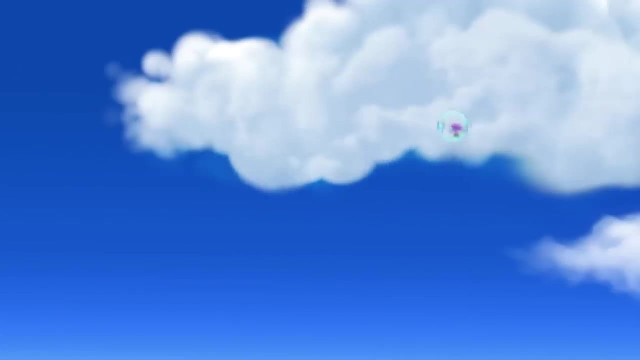 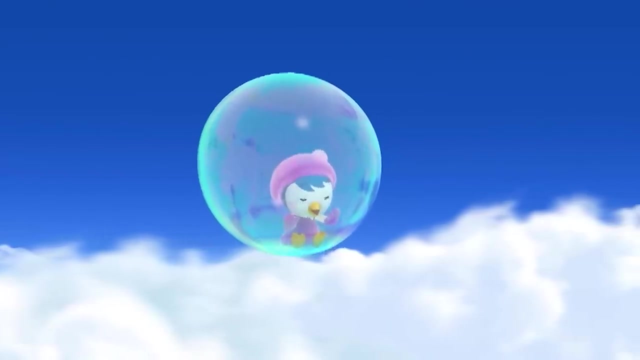 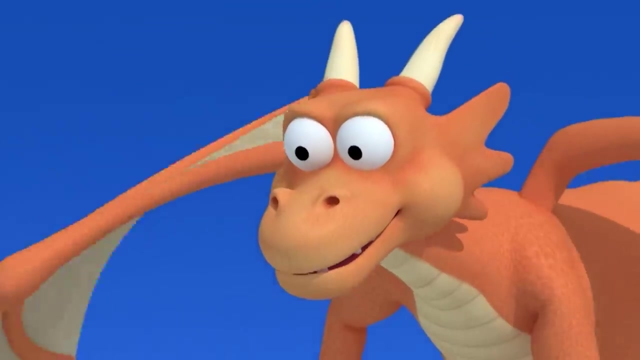 Yeah, The wind is blowing. I want her. No, Patty, Wow, So pretty. How am I going to get down? At that moment? Tongtong was on his way to the village. Huh, What's that, Hi Patty? 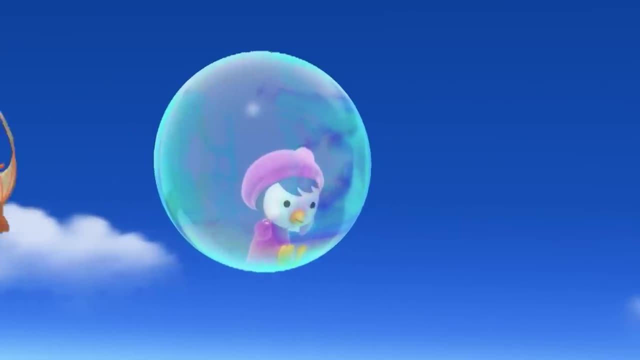 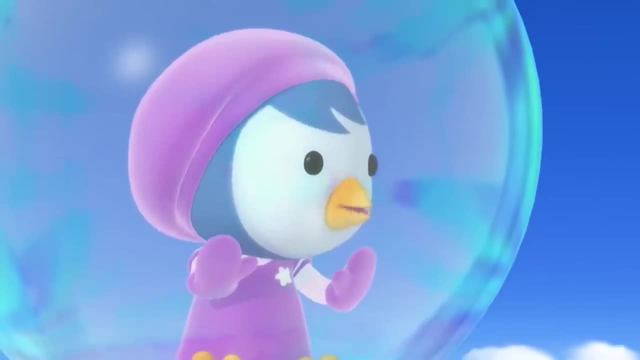 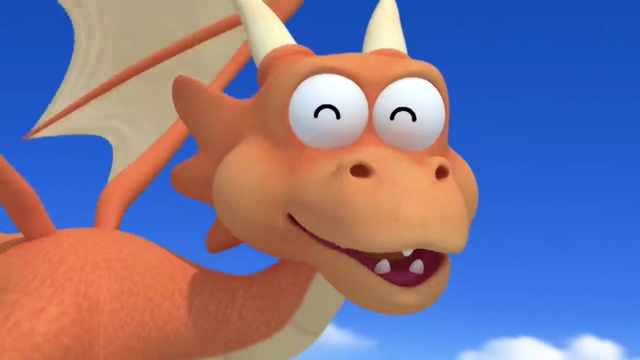 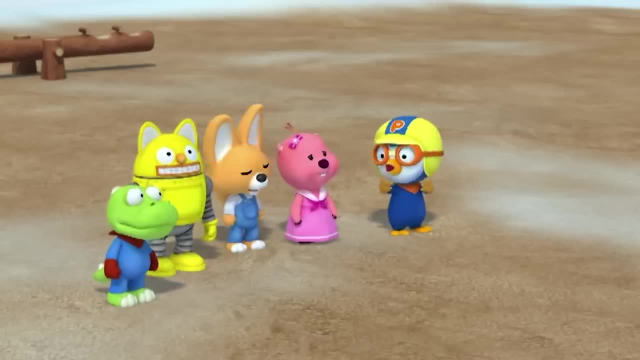 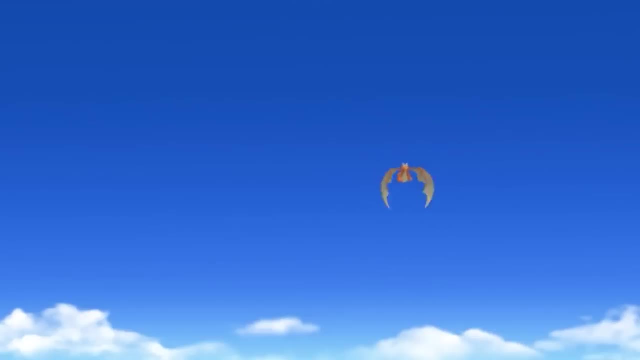 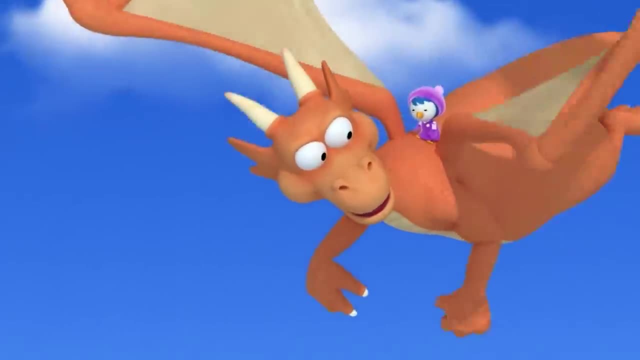 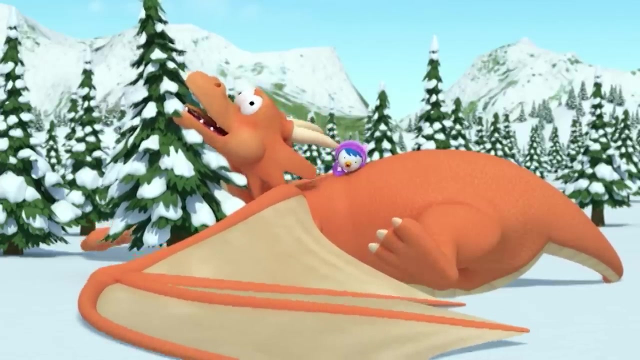 Okay, Oh, Patty, I'm sorry, But could you get off my back. Huh, Okay, Huh, Whew. Oh, I'm sorry, Patty. I'm sorry, But could you get off my back, Huh. 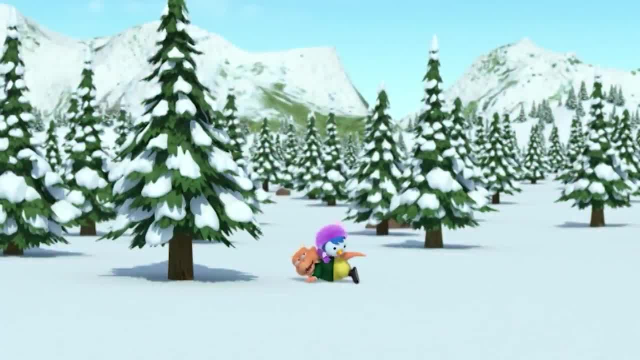 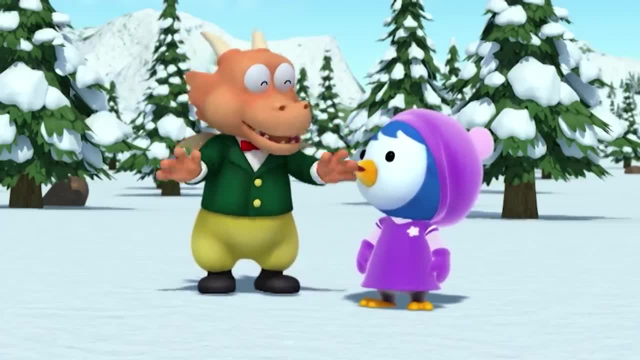 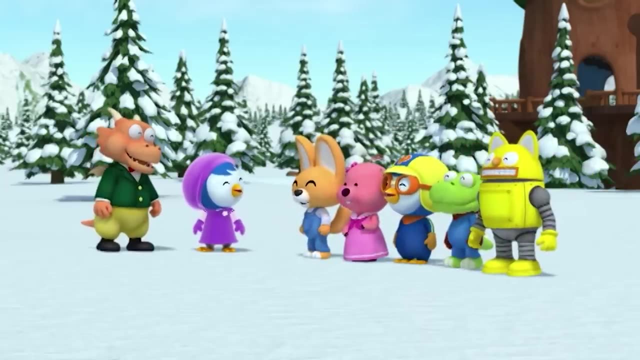 Huh, Okay, I Phew Patty, I'm sort of tired. Oh, Are you okay? This is nothing, Don't worry, Are you okay? Bye guys. Thanks to Tong, Tong, Petty is safe and sound. 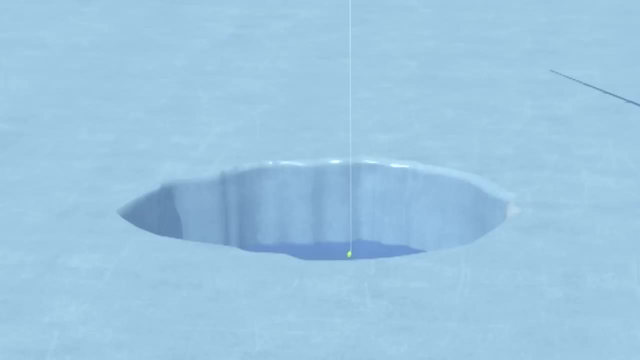 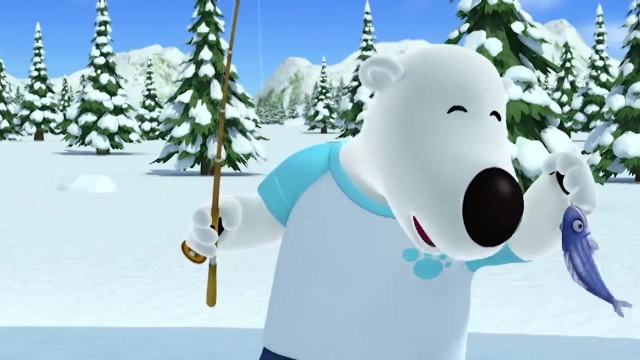 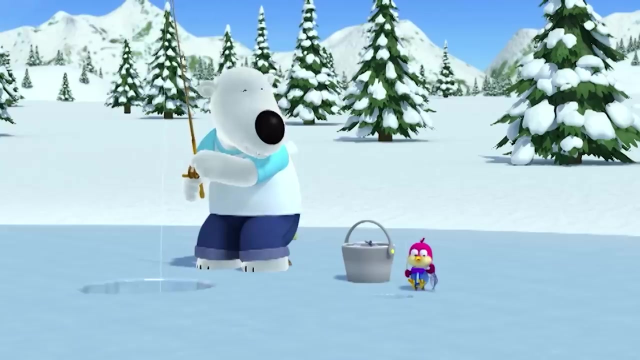 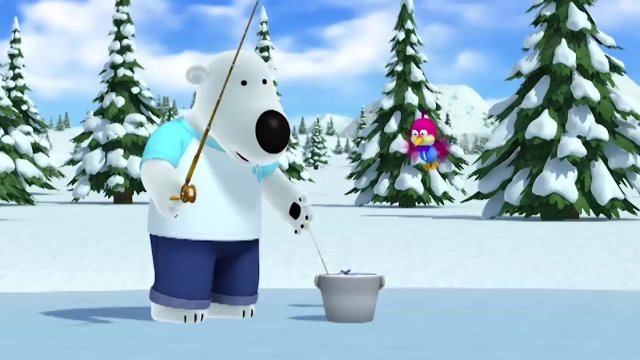 Poby is ice fishing with Harry. Wow, look at this, Harry, It's really big. Yeah, good catch, I got it. Nice one, Harry. Harry, I got another bite. The bucket is full. Yeah, let's head back. 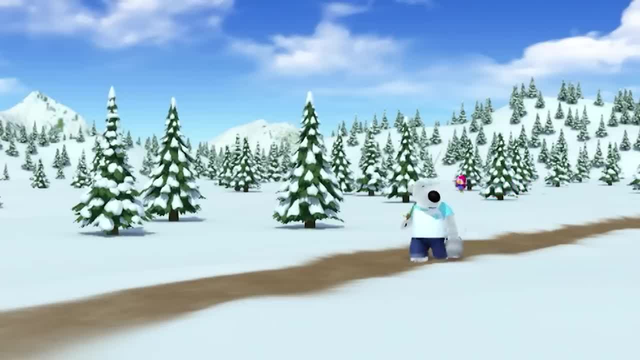 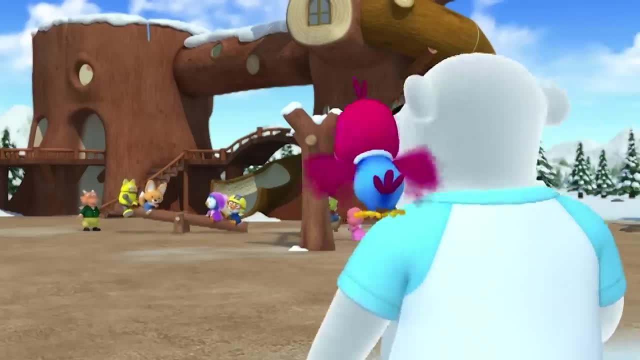 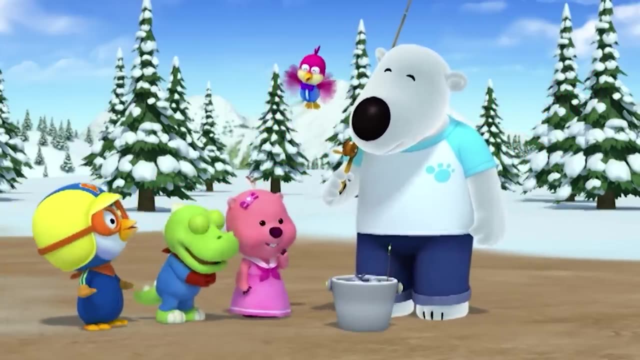 Okay, Poby and Harry went to the playground in a great mood. Hey guys, Hi Poby, Hi Hi, Hi guys. Look at this, Poby and I caught them all. You caught a lot, Wow. 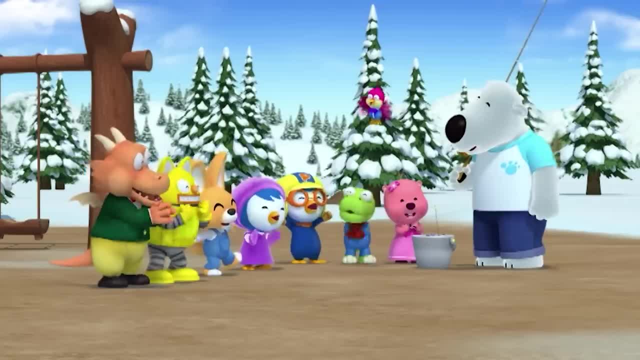 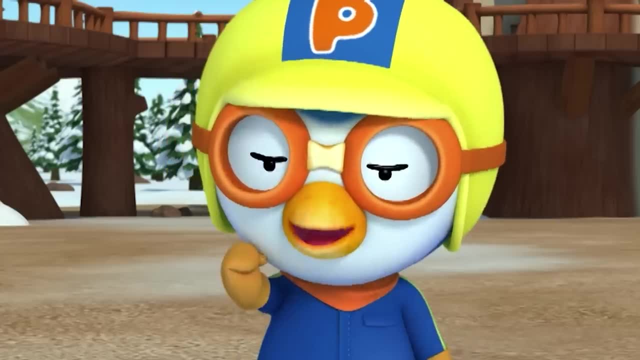 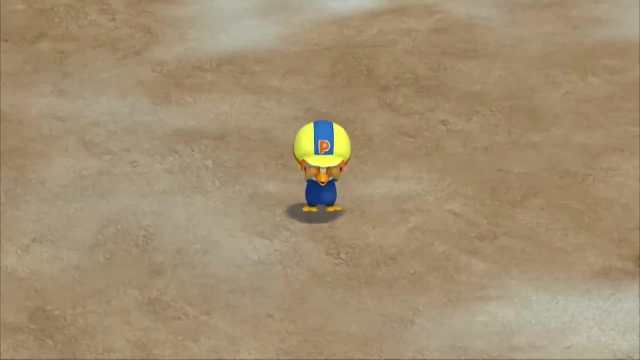 Yeah, we caught a lot so we can all share. Who's going to be it? Rock paper scissors- Oh, I lost. I guess I'll seek. I'll count to ten. Everybody hide One, three, four. 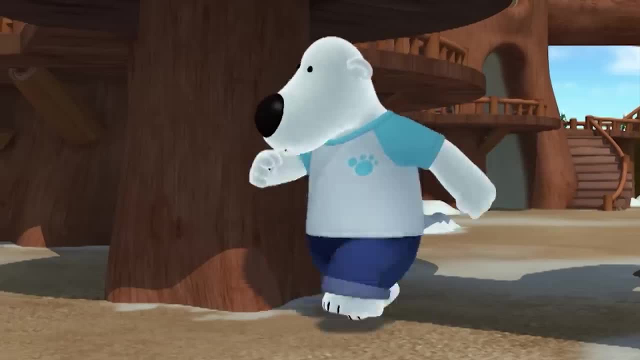 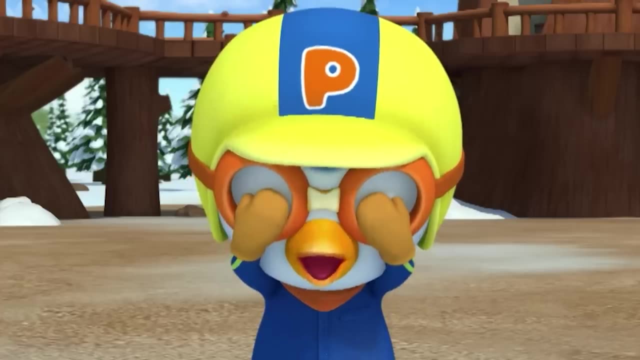 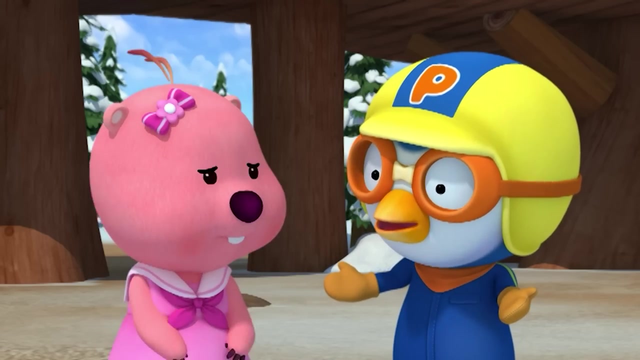 five, six, seven. Where should I hide Over here, Over there? Eight, nine, I don't know Ten. Here I come. Ouch, Are you okay, Luppy? Yeah, I'm okay, I couldn't even hide. 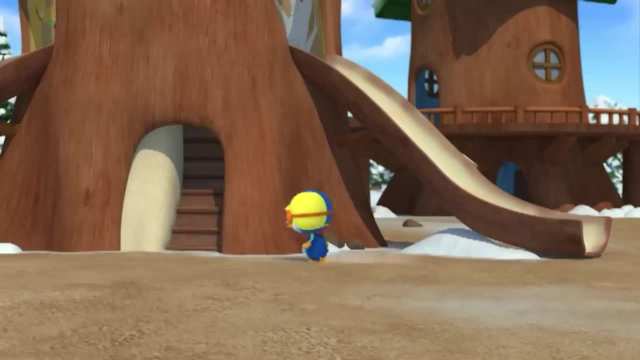 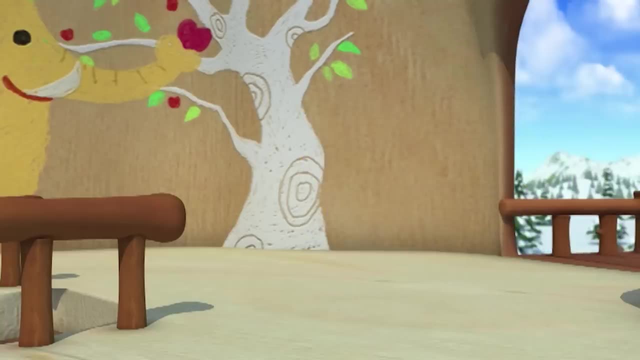 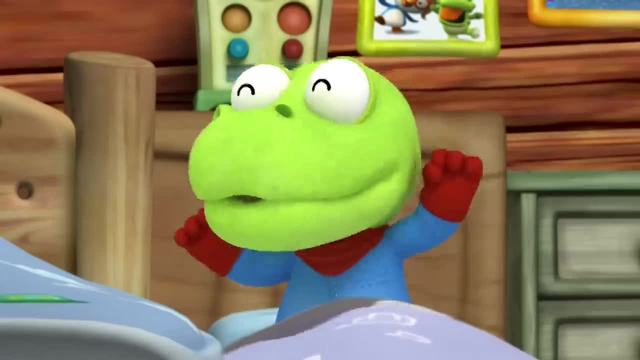 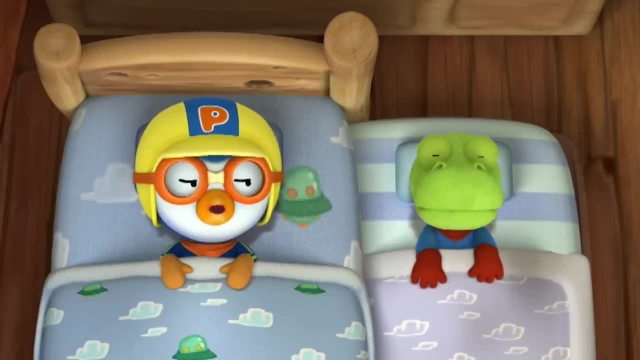 I think I heard Petty and Harry's voice: Krong, Krong, Krong, Krong, Krong, Krong. You're on. Let's have fun tomorrow too. Time for bed, Krong, good-bye. 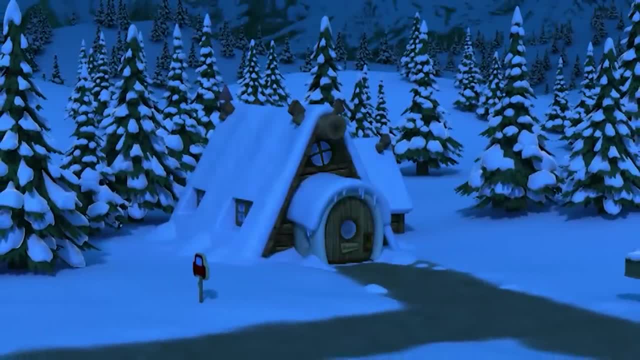 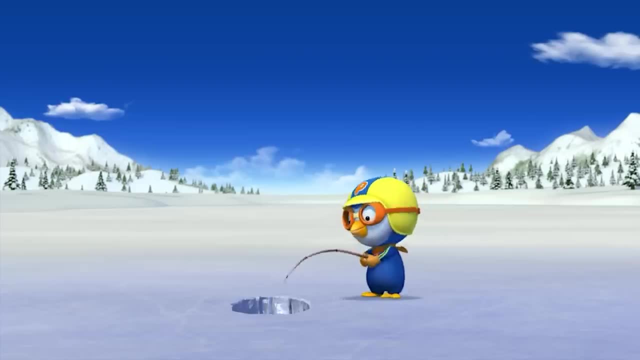 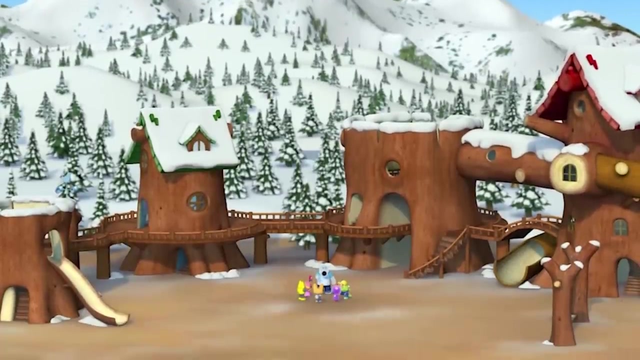 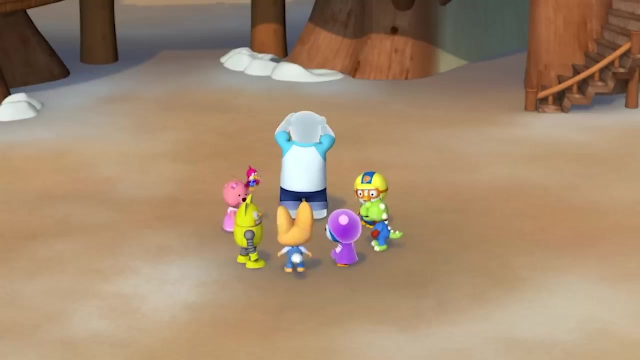 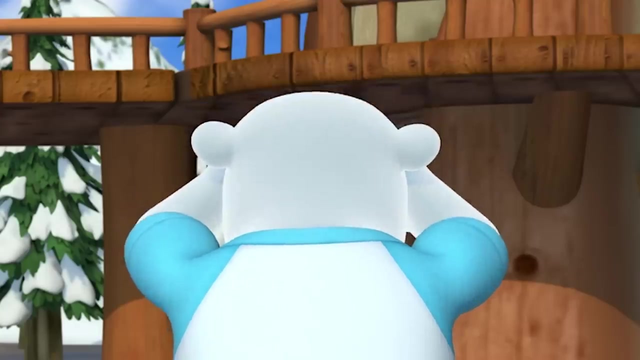 Today was another great day. Pororo, Krong, sweet dreams, Wonderful Playground. Pororo and friends are at the playground. I'm it. I'll count to ten. One, two, three, four, five, six, seven, eight, nine, ten. 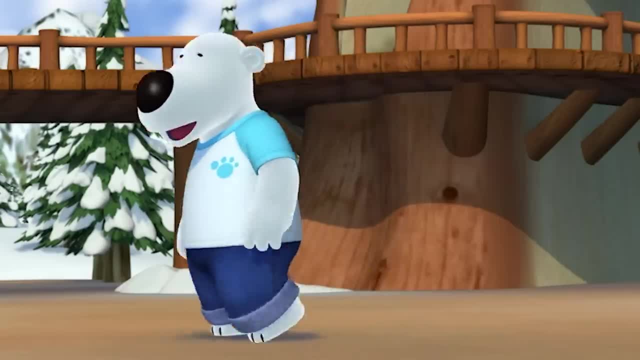 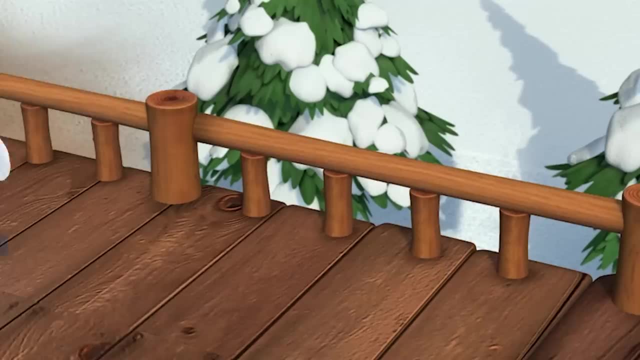 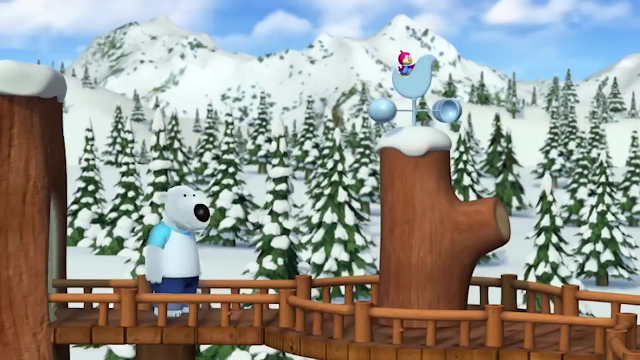 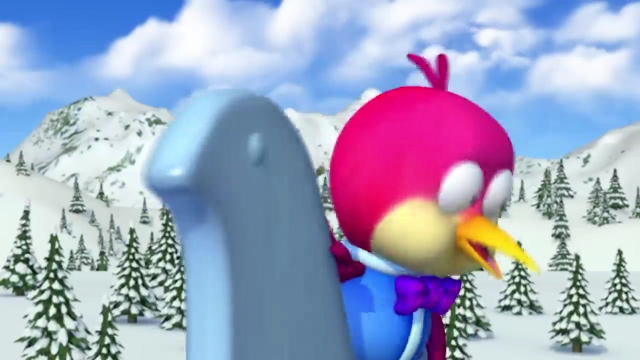 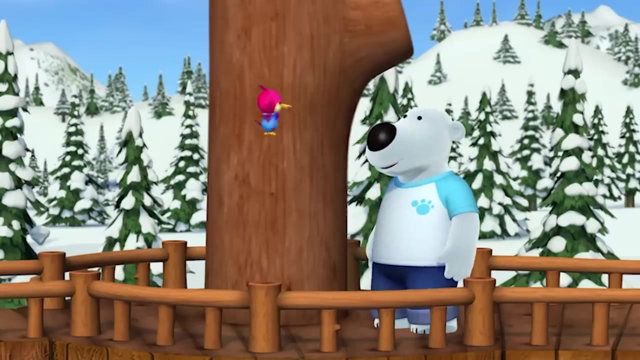 Here I come. Where should I start? I'll start over here. Nobody is here. Where are they hiding? Maybe somewhere else? Suddenly, a wind blew. I'm getting dizzy. Ouch, Found you. If it weren't for the wind, I'd still be safe in my hiding. 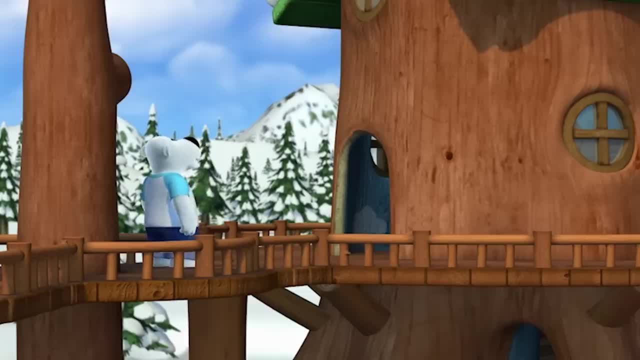 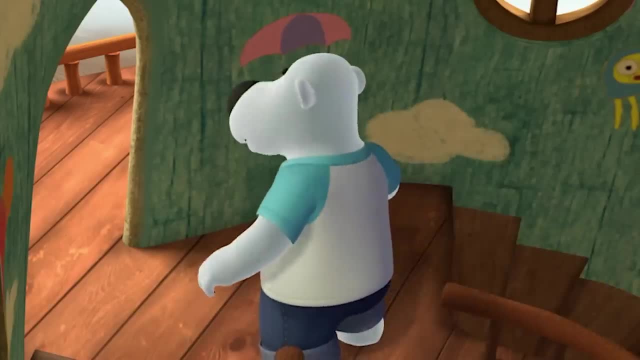 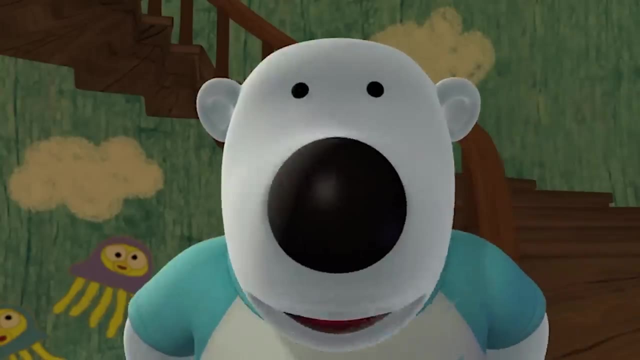 Where should I go next? Maybe I should go to the park, Maybe over here. Oh, he's coming this way. Where are you hiding? Where are you hiding? Should I try upstairs? Something is strange. Did the picture change? Oh, that tickles. 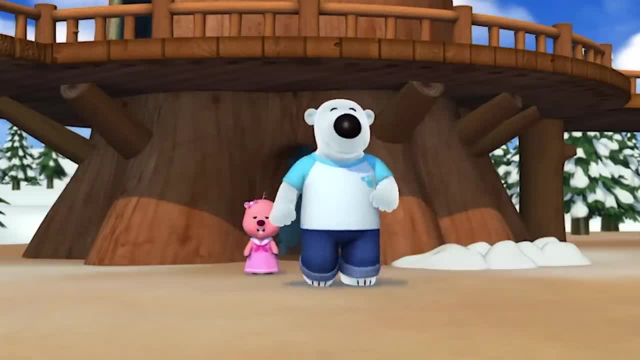 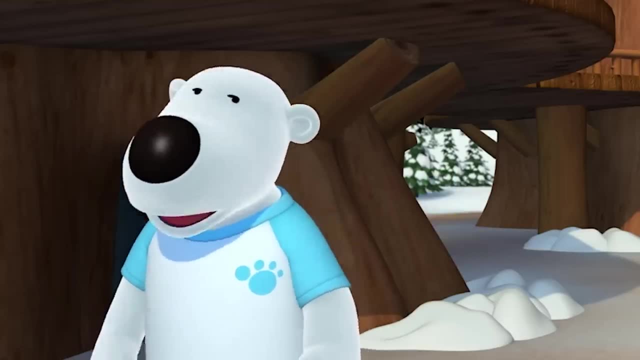 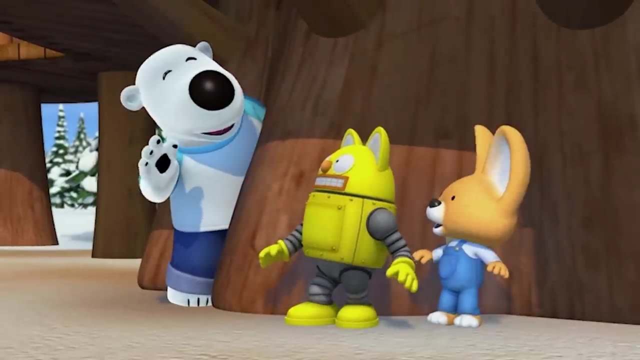 Ruby got you. Can't believe you found me so fast. Where should I look now? Hmm, Should I go that way? Don't make any noise. He almost got us, Not almost. I got you. Should I go this way this time? 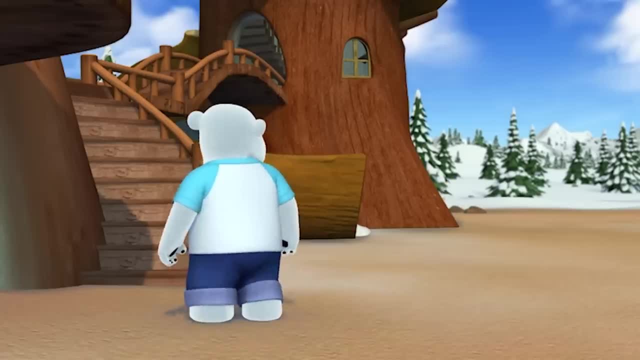 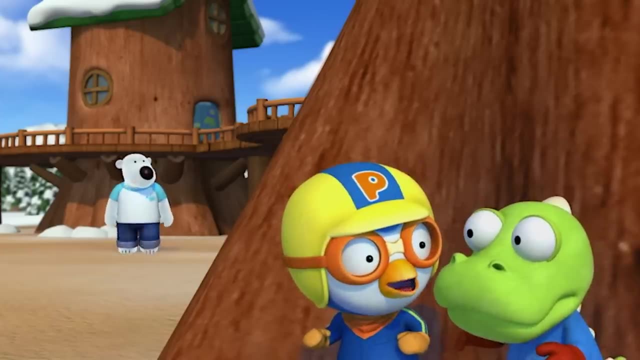 Or wrong? Hmm, No, I'll go that way. Poby headed to where Pororo and Krong are hiding. She's coming this way. Krong, Krong, Pororo, Krong, Shh, Quiet. Poby is coming this way. 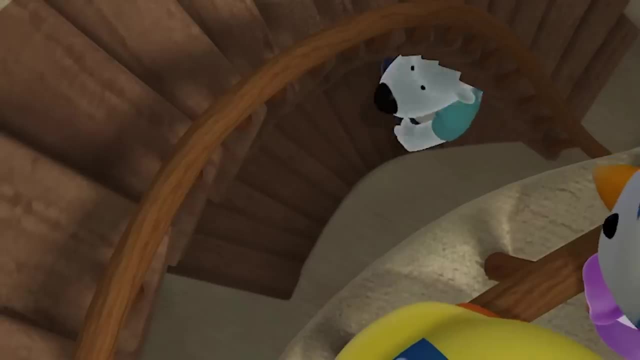 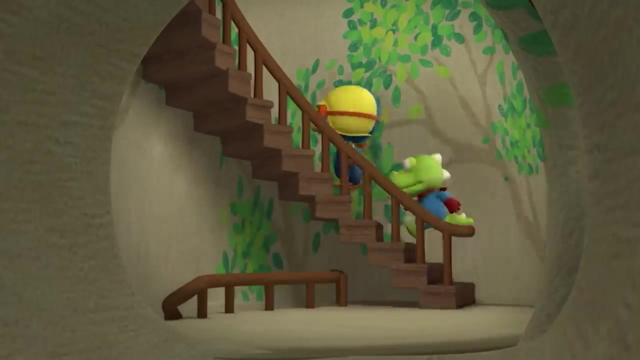 Krong, Krong. Poby is coming this way. Poby is coming up. Hide, hide. if you can, We should hide. I'm going this way, Krong, let's hide upstairs. Hmm, How should I start looking here? 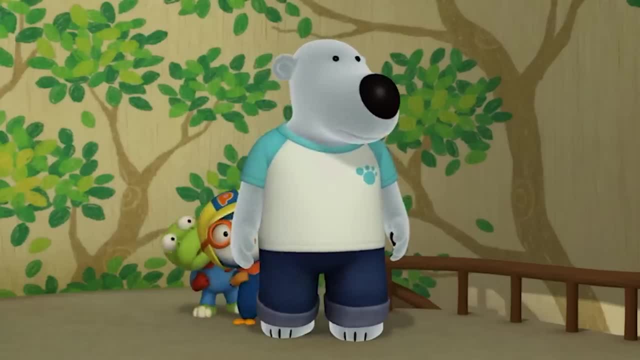 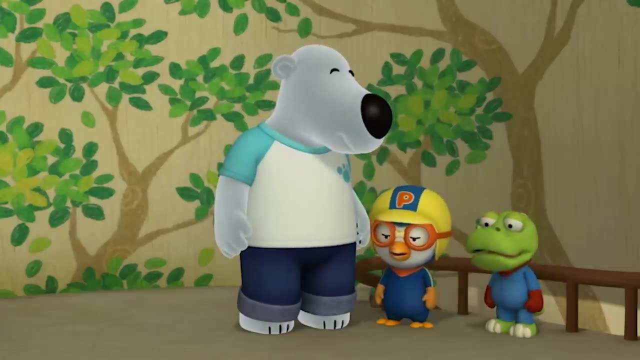 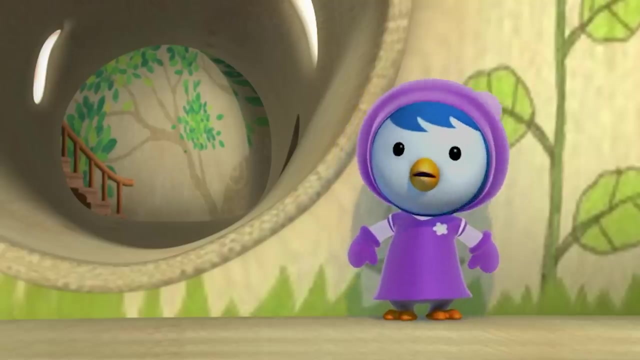 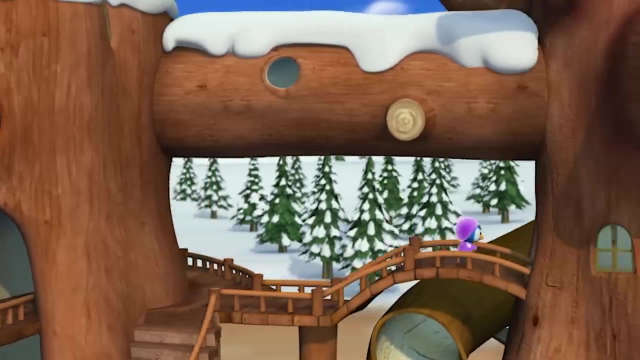 No one's here. Krong, Pororo, Krong, I found you. Now all I have to do is find Petty. Which way should I go This way? Petty went away from Poby and went to hide. Hmm, Not here. 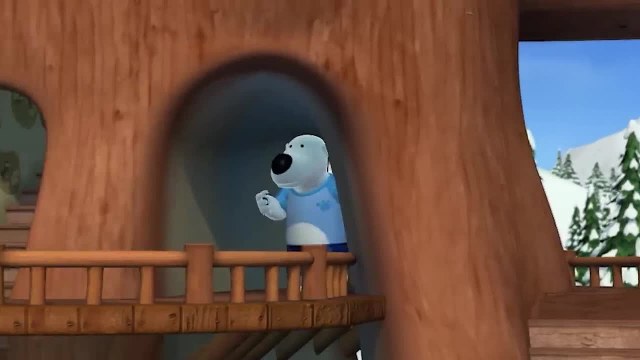 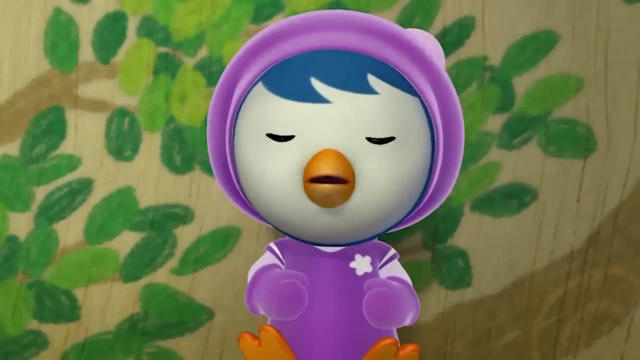 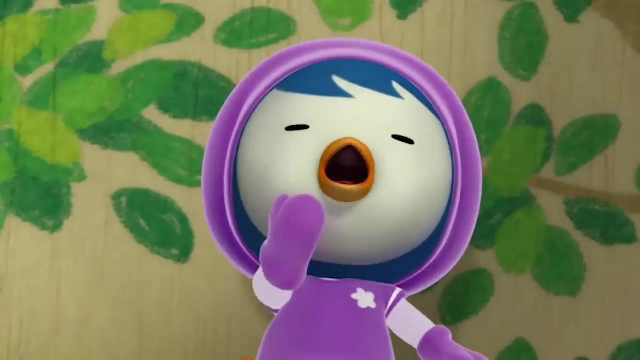 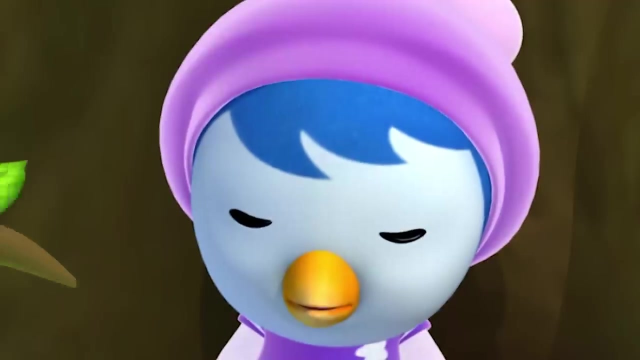 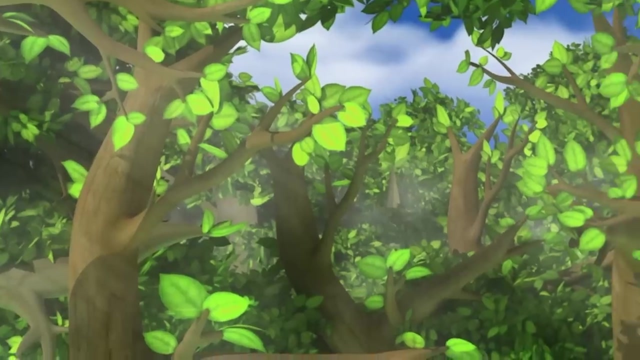 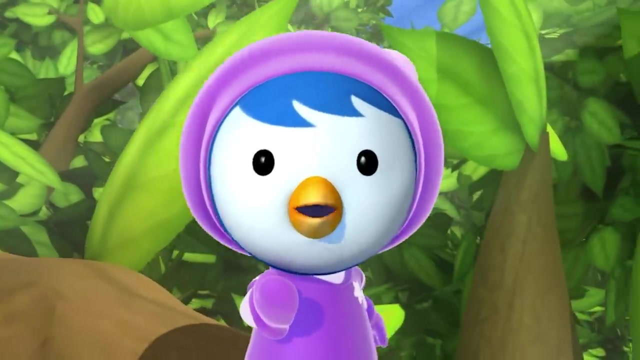 Where is she hiding? Hmm, He almost caught me. Huh, This is Wow. What pretty pictures. Oh, I should rest here. Uh, Oh, Where am I? Wow, Where is this place? It's beautiful. It's filled with trees. 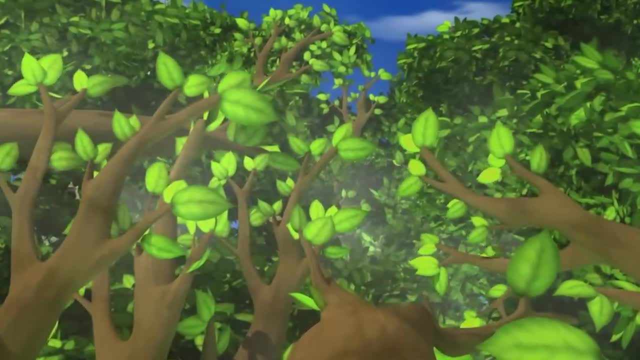 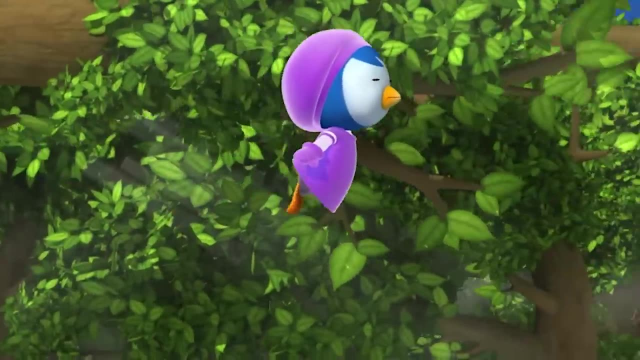 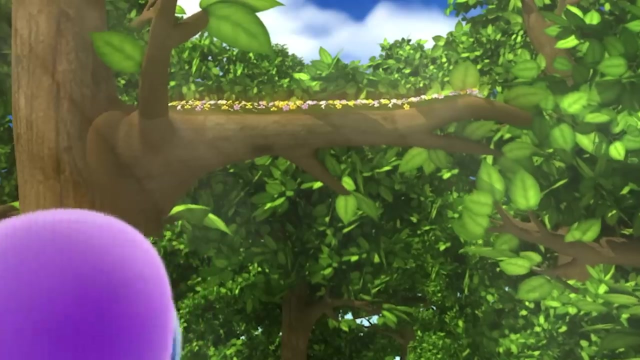 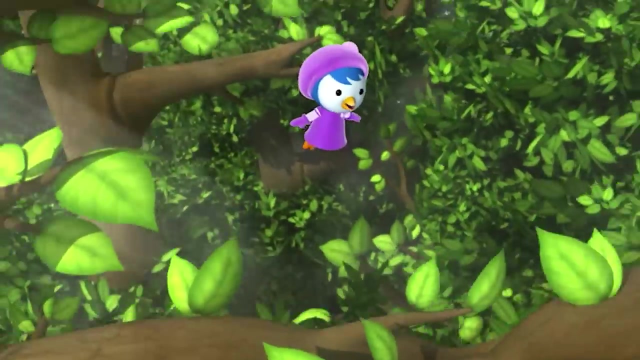 Hi, Welcome Petty. Hello, Hello trees, Oh, Oh, Oh, Where should I go? Wow, There are so many flowers. Let's go and have a look. Petty jumped on a leaf and jumped up again. She found where the flowers were. 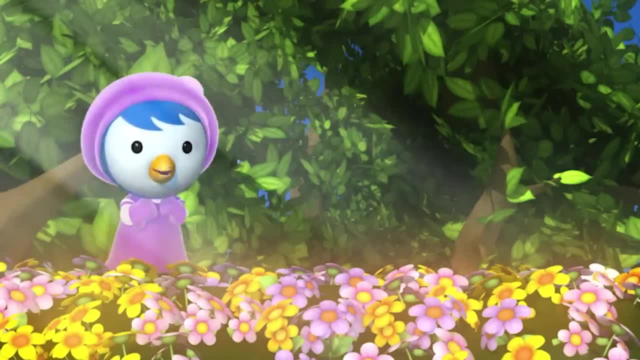 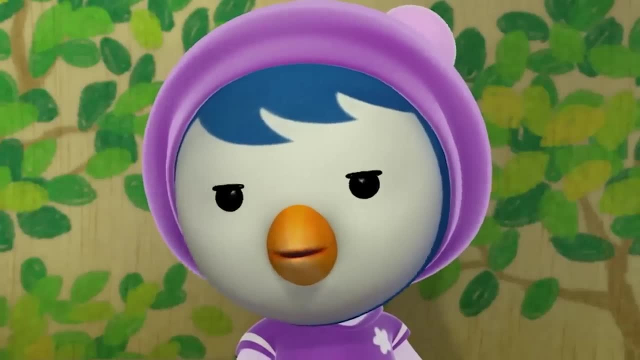 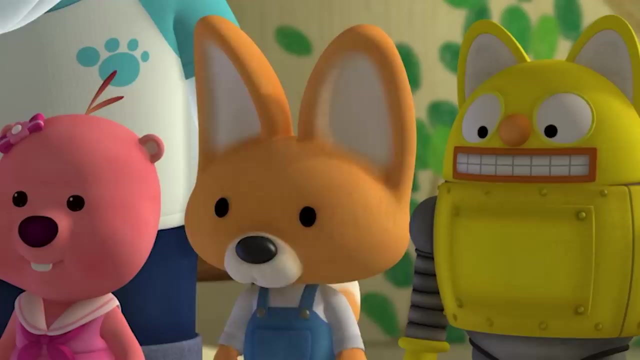 I'm here. Wow, It's so beautiful. Hi, Hi, Petty, wake up. How can you go to sleep during hide and seek? How come I fell asleep? Yes, And we've been looking for you everywhere. That is right. 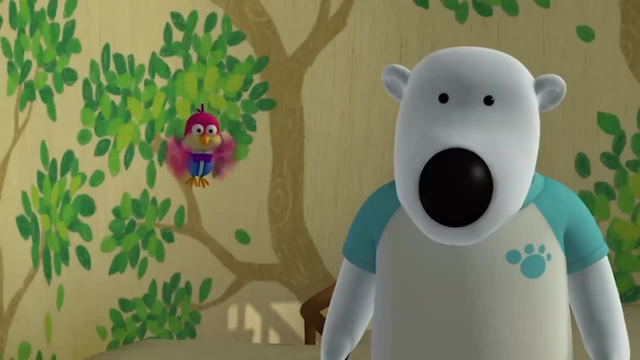 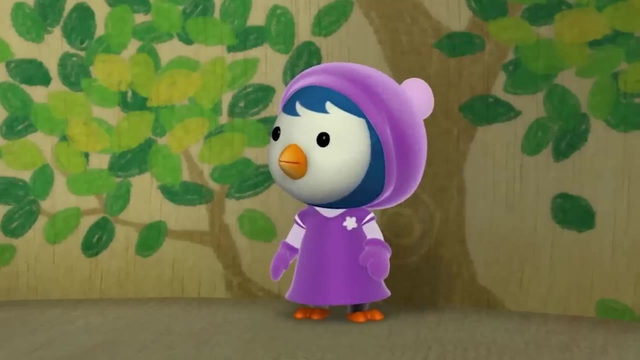 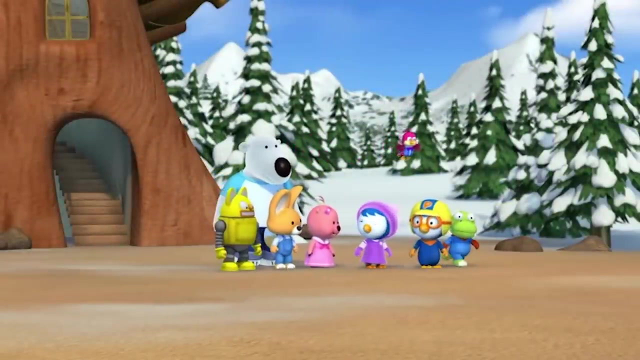 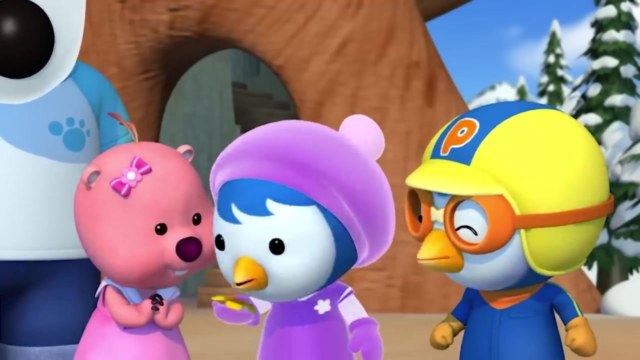 I'm sorry, It didn't seem like a dream. Let's go home. You're right. Yes, It was fun. Yes, What's this? What kind of a flower is this? I didn't see it a while ago. It was the flower Petty saw. 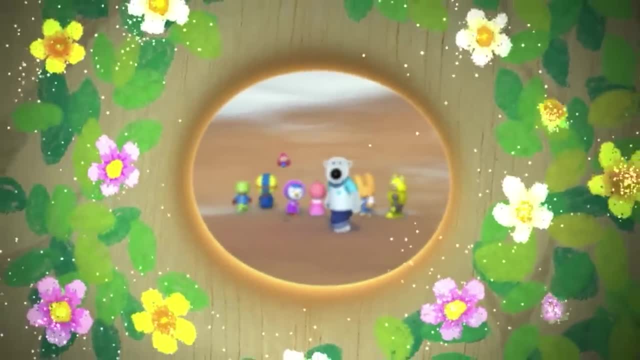 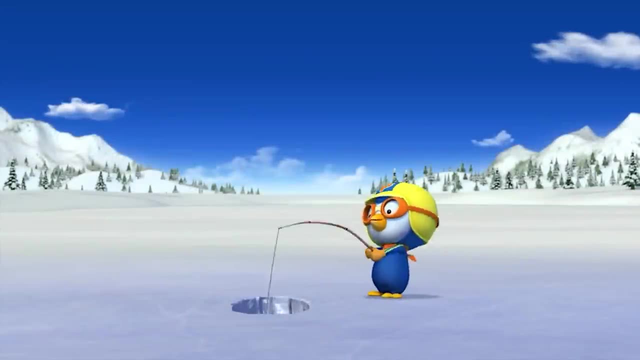 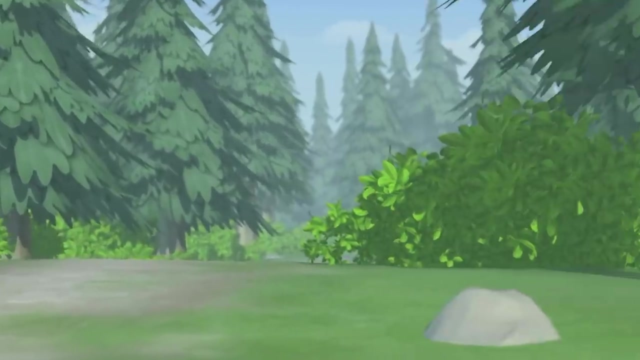 Wow, It's pretty Pororo, and friends might not know it, but it's a beautiful flower. Let's go to the playground. Magic Potion 2: Wow, The fog is so deep I can hardly see anything. It's such a beautiful forest. 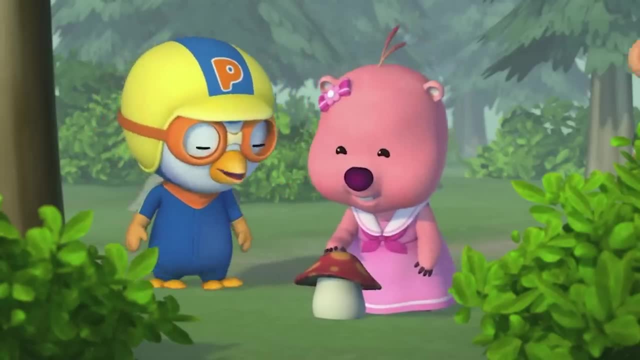 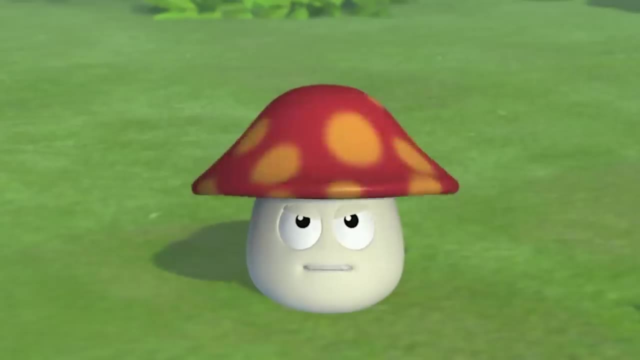 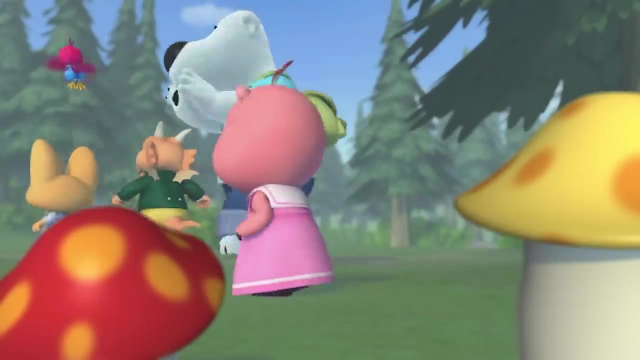 Huh, What a pretty mushroom. Oh, it is. Huh, Who are you? The mushroom is talking. We have intruders- Me too. Let's get them Run Toot toot. Use your magic to save us from the mushrooms. 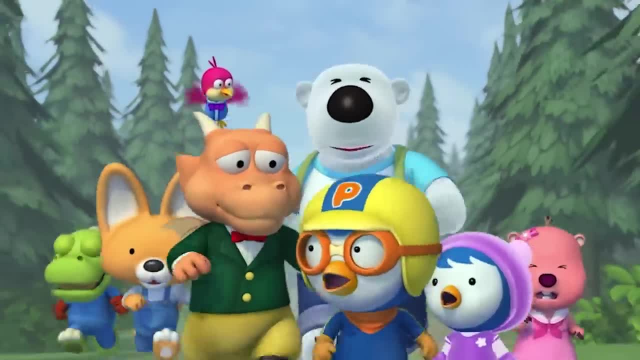 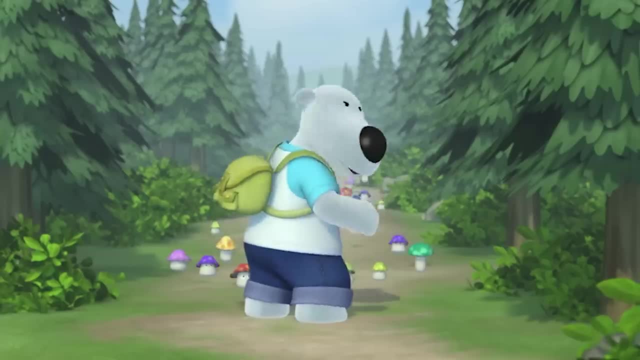 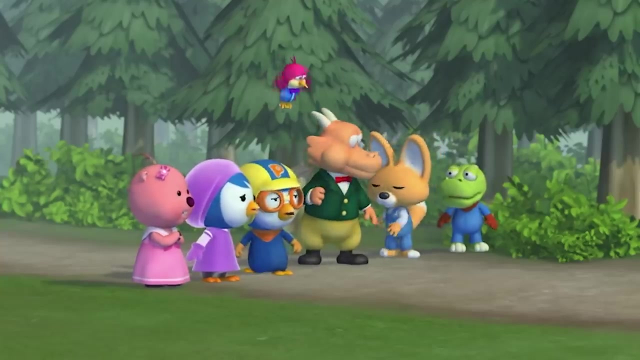 I can't use magic in this forest. What That does it? Hurry up and go. No, Leave it to me. I have a plan. Let's go. You're brave to face us alone. Do you know what I like eating the most? 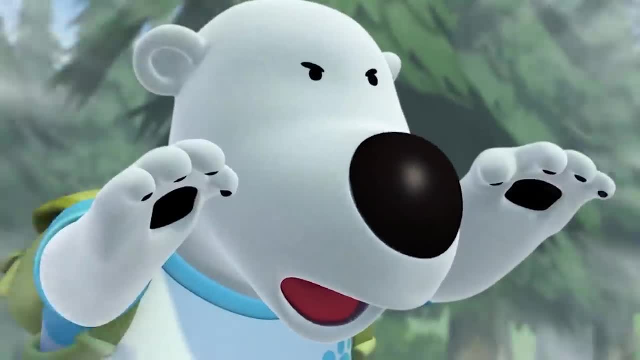 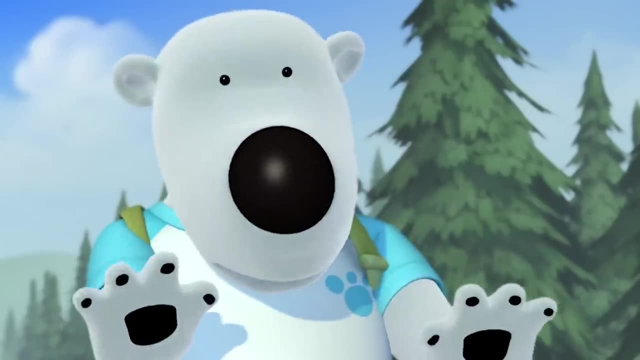 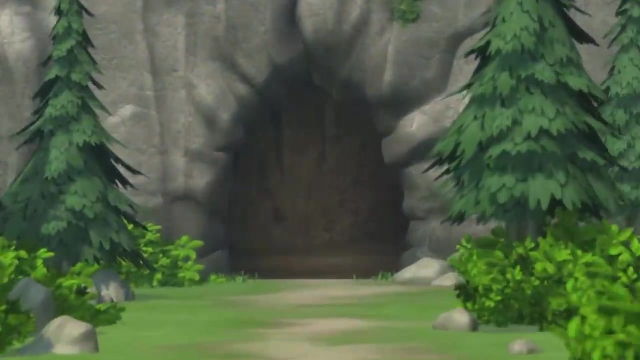 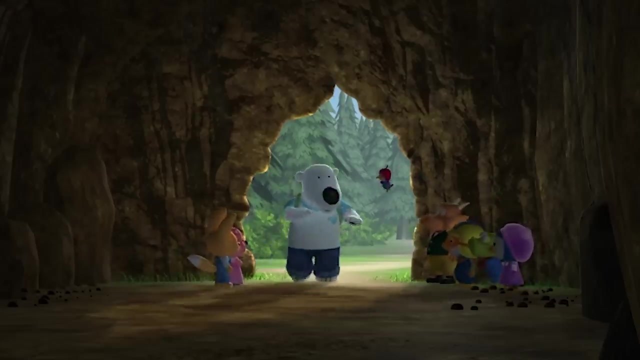 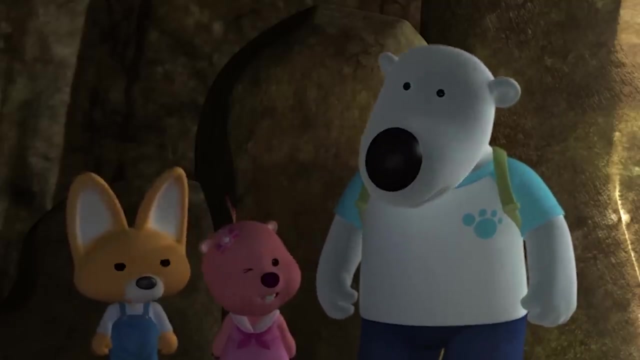 Mushrooms, Mushrooms, Is that so You want to know? mine Bears, Bear, Bear. That was the plan. Let's go run. No, No, Here you are, Hi Bear. It's all right now. I'm glad that you're all right. 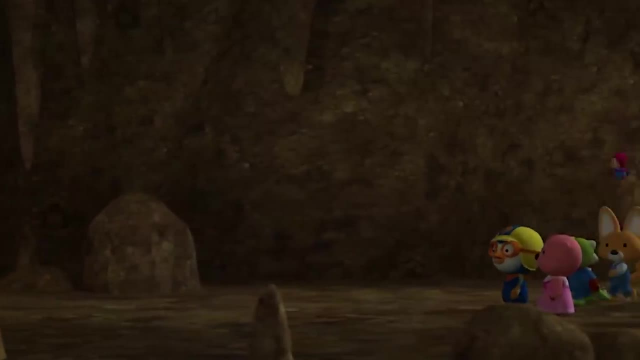 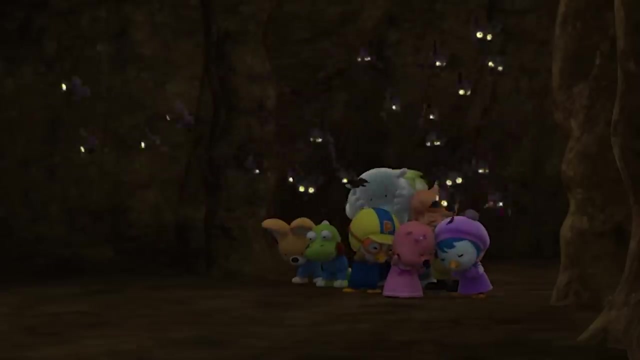 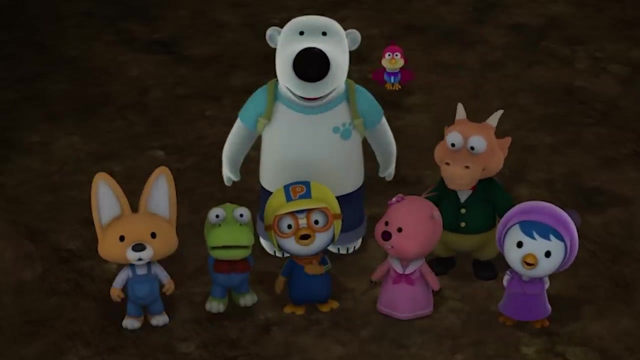 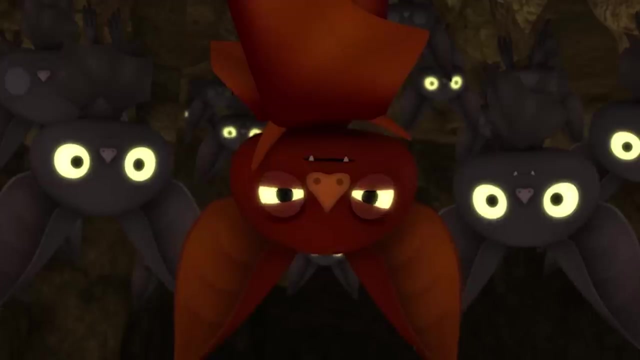 Yes, Bear, Bear, Who are you? You mean us. I'm Boro And they're my friends. What are you doing in here? We're looking for the fruit of the sun tree. Fruit of the sun tree, Why you? 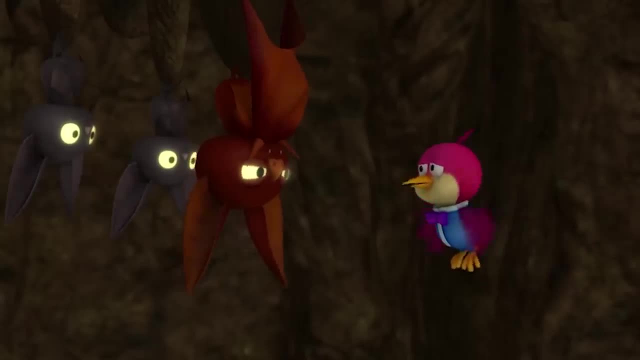 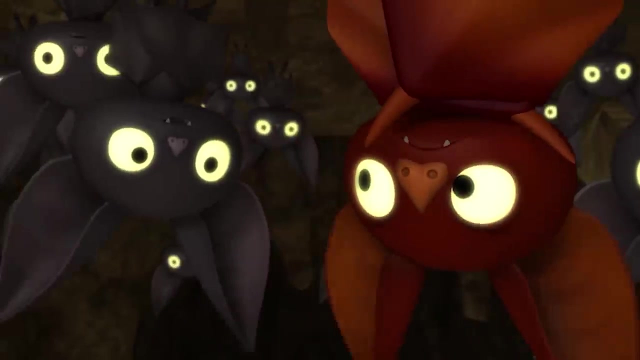 That is our sacred treasure. Wait, Our friend is under a spell. We need the fruit to turn him back. Please help us save our friend. A friend is under a spell and needs the fruit. He's going to die. He's begging us to help him. 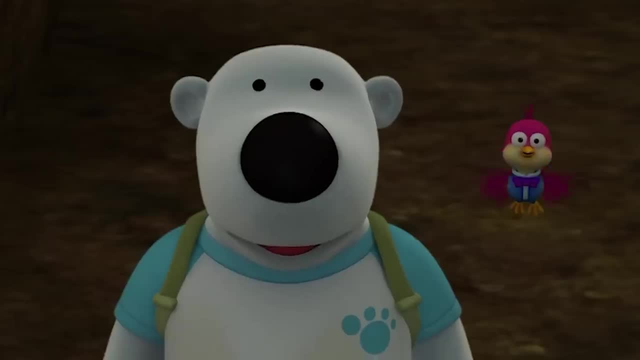 Risking danger to save a friend. I'll let you have a chance to pick the fruit from its tree. I'll let you have a chance to pick the fruit from its tree. I'll let you have a chance to pick the fruit from its tree. 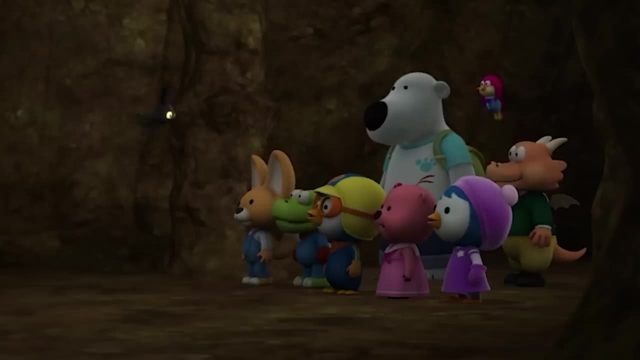 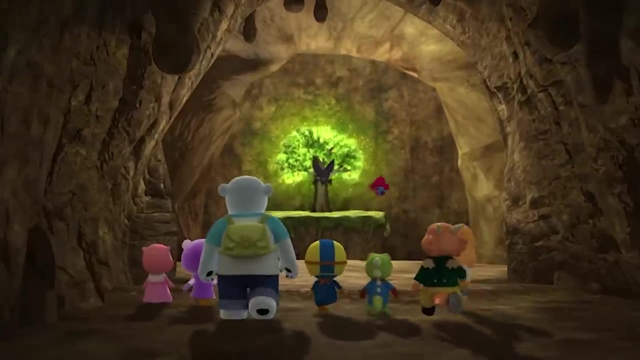 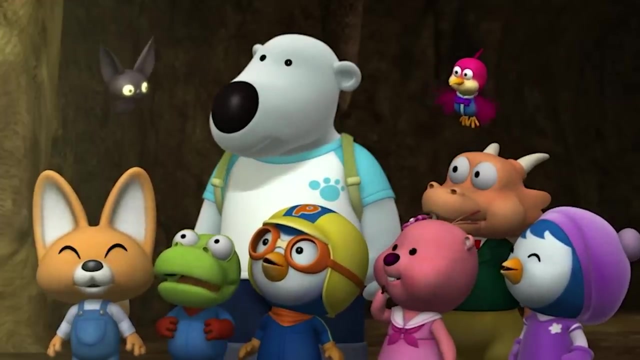 Take them to the tree. Yes, Follow me. Okay, Here you are. Wow, The friends have finally found the sun tree. I'll leave you now. You should be able to know what is needed from here. Thanks, How do we get across there? 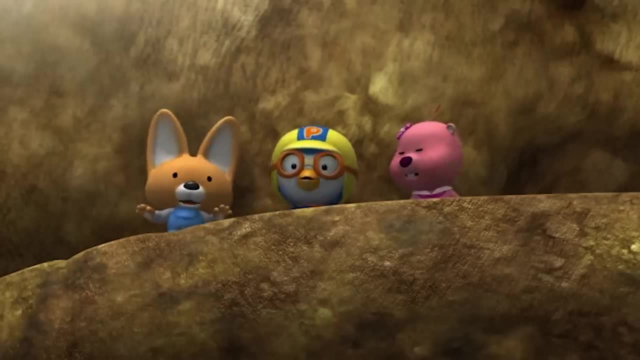 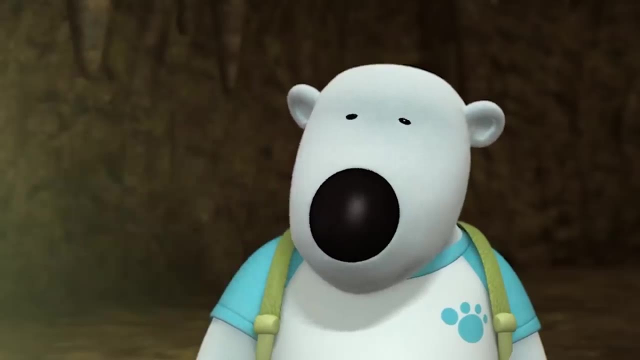 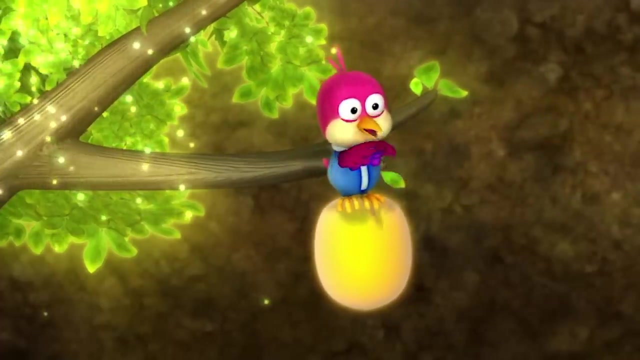 Huh, It's too high, Let me see. No, it's too dangerous, I'll go, I can fly. Be careful, Harry. Piece of cake. Throw the line this way and I'll hang it so you can pick the fruit. 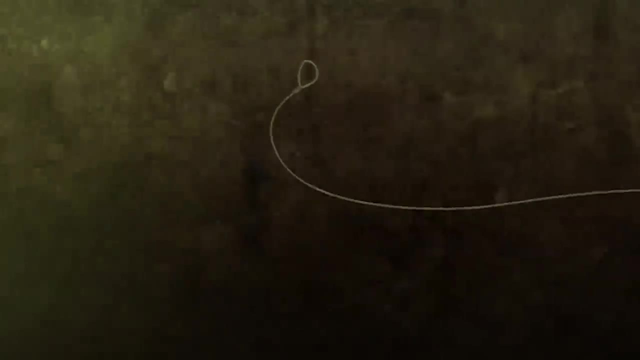 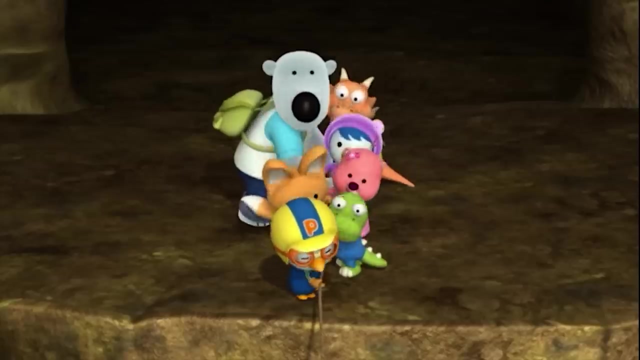 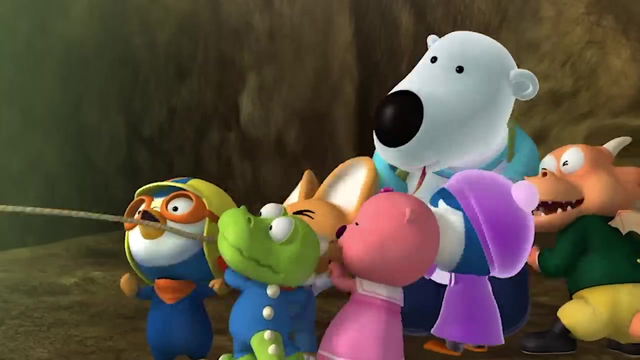 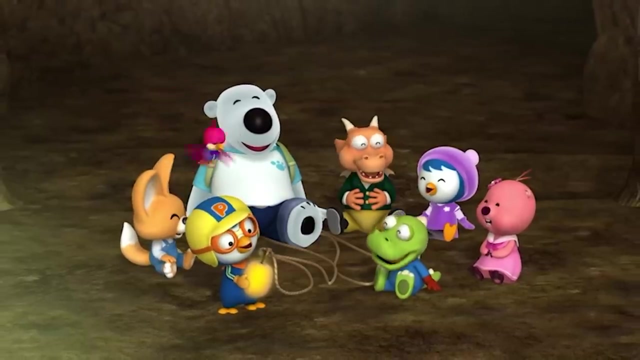 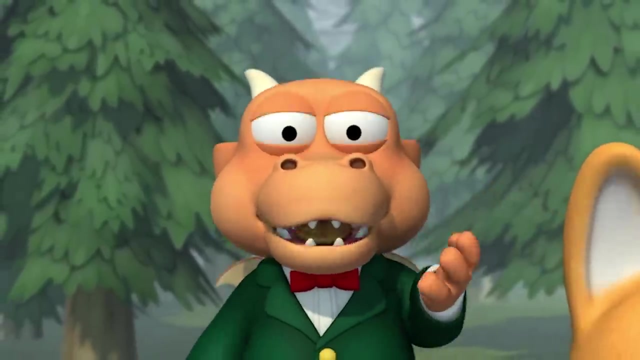 Okay, Catch Done, Now pull. The fruit is moving. Let's give it one more try. The fruit is moving, Let's give it one more try. Whoa Got it, Got it, We did it. Wow Clock. how is Radha doing? 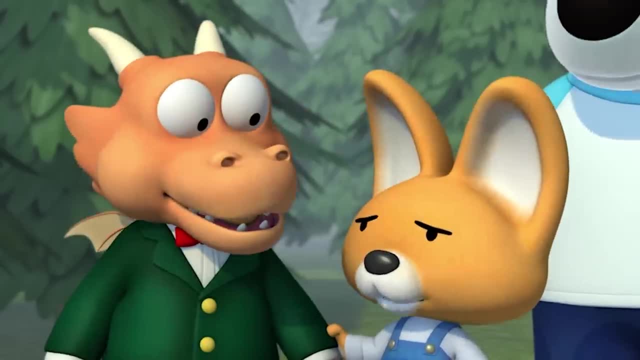 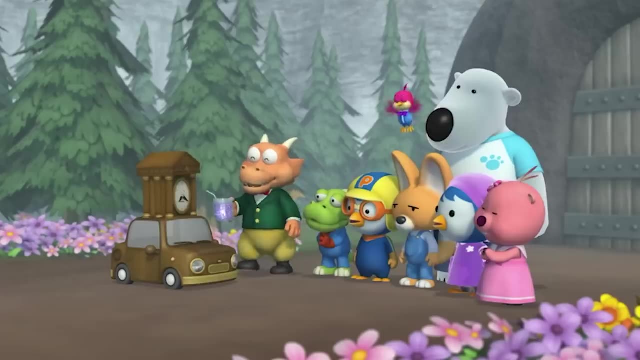 He keeps going in circles like that. You're sure that this will turn Rodi back. You're sure that this will turn Rodi back? Yes, There, All done Drink. I'm sure it'll have the right effect this time.